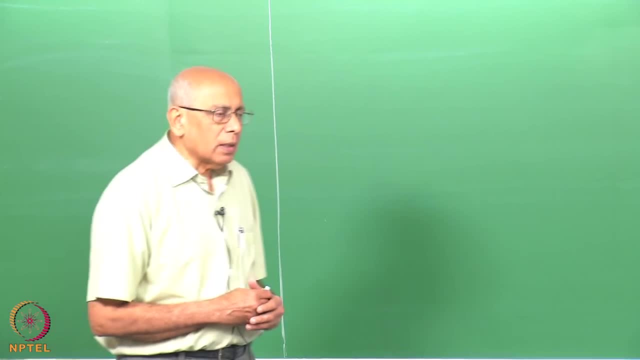 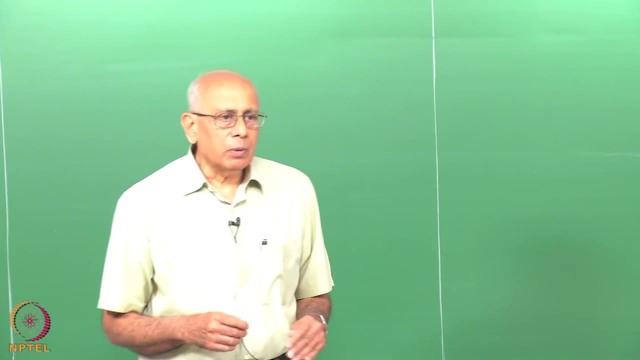 mechanics and the equilibrium level, which is that, for a given system in isolation, all accessible microstates are equally probable. We have no such guarantee now. We are going to Push and pull on a system, we are going to apply perturbations to it, we are going to 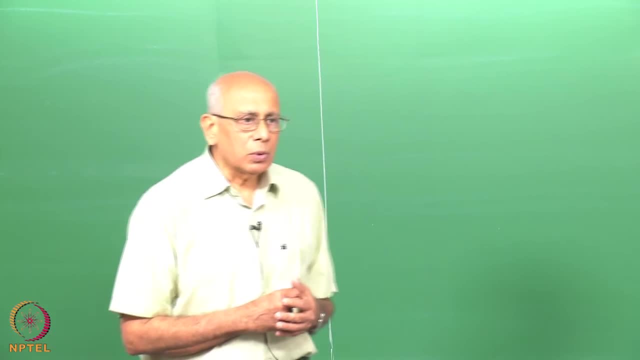 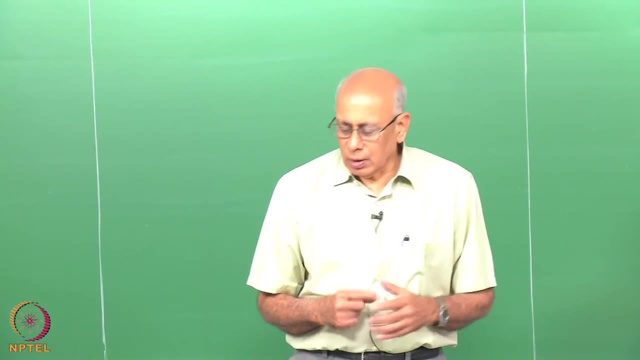 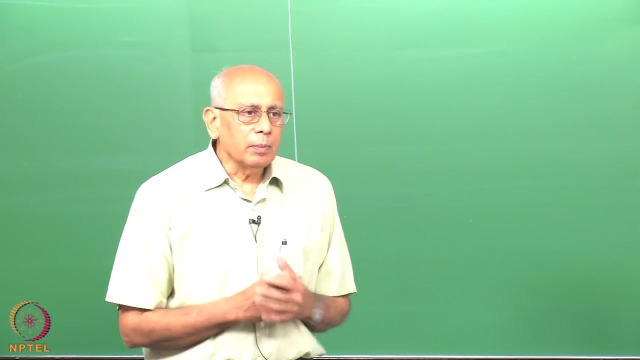 move it away from equilibrium and watch what happens as the system is left alone. Now we need a model to start with, and we will start with the simplest of models. perhaps We will start with a model where you have a fluid and it is in thermal equilibrium at a fixed 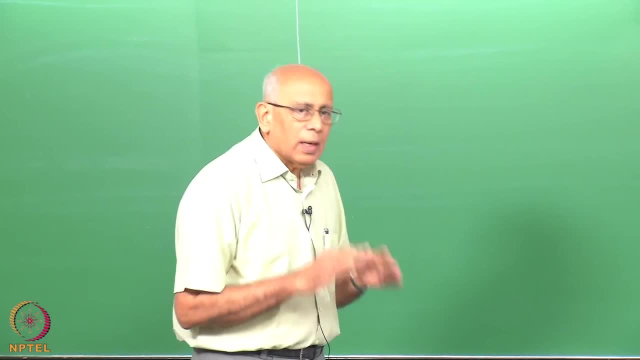 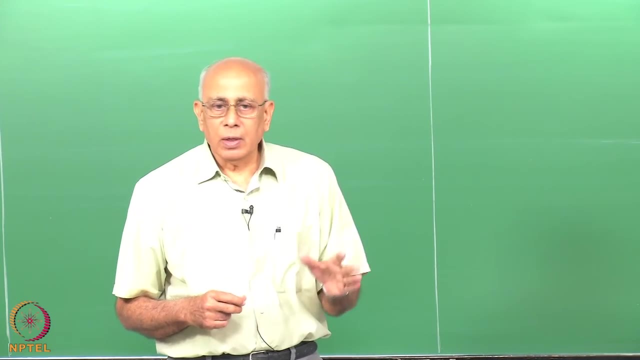 temperature, The fixed number of particles, fixed volume, and it is in thermal equilibrium. If it is a gas, for instance if it is an ion, it is in thermal equilibrium. If it is a gas, an ideal gas, then we will know that the maximum in distribution of velocities applies. 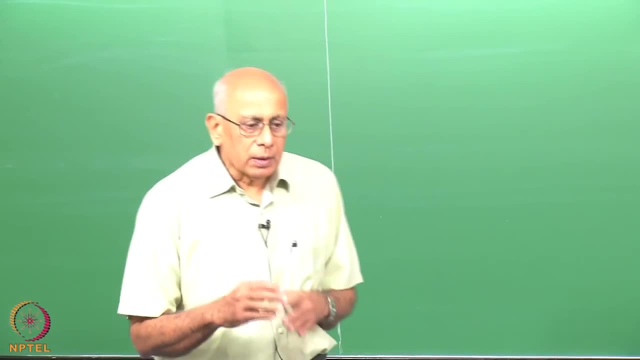 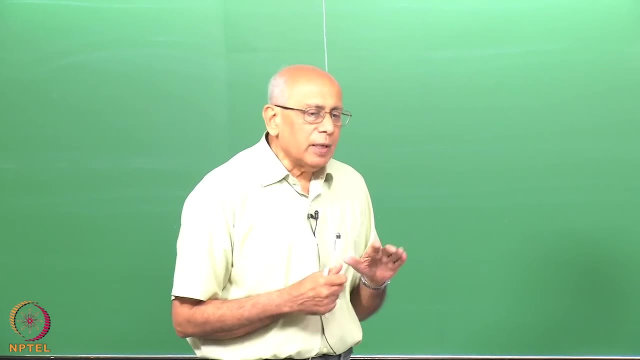 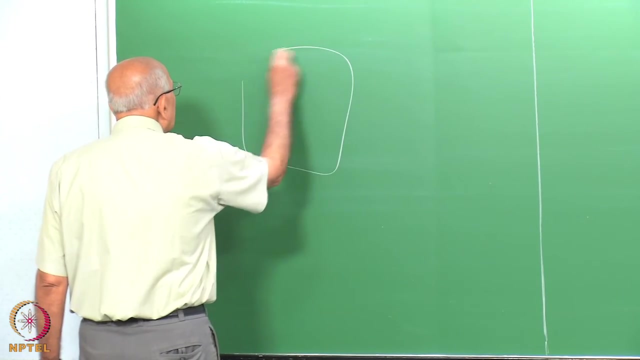 and you also know that the particles are uniformly distributed throughout the volume. We write down in equilibrium what the phase space density is for a given particle. So you can easily write down the fact that if you have this container with a whole lot of particles- inside N of n, for instance, and if it is an ideal gas, I think this is very obvious now, If it is an ideal gas, we can write down what it is, and that could be also applied to that fate space density for a given particle. So you can easily write down what it is, insanally characterize in power, so that we can set a value there and somehow for this that nothing will arrive in that volume. 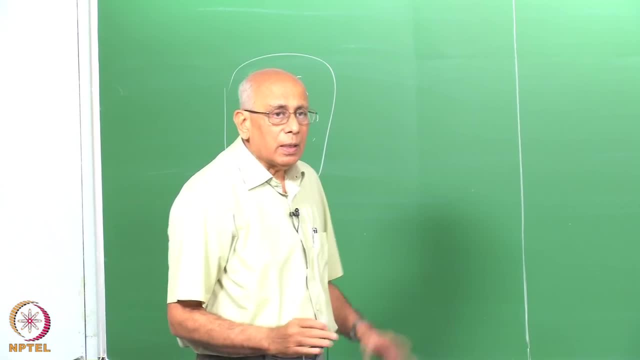 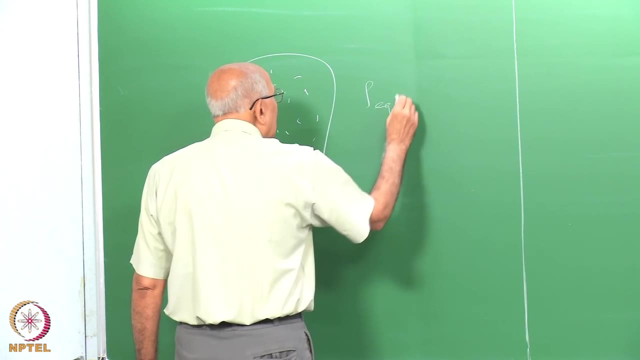 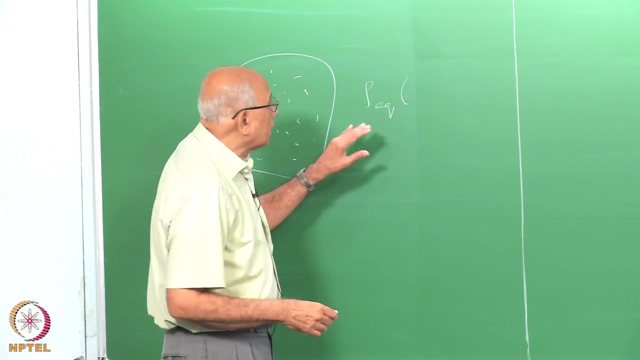 then we can write down the phase space density immediately. It is clear that let me use a symbol for it: rho equilibrium, and now I want the single particle phase space density. This is the probability that the probability density that a particle is at any point r inside the 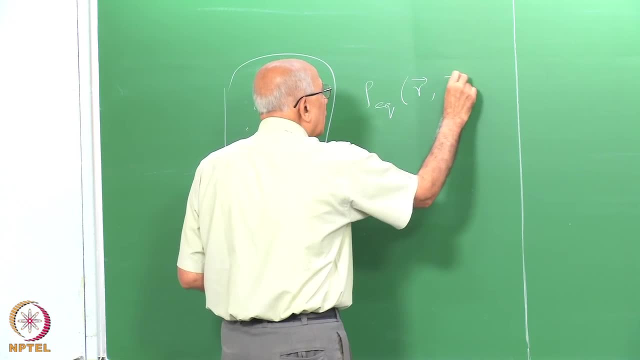 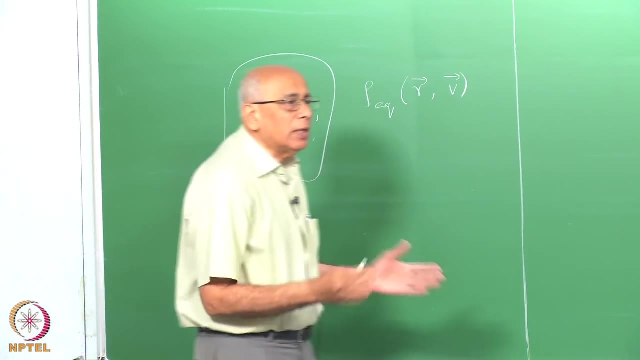 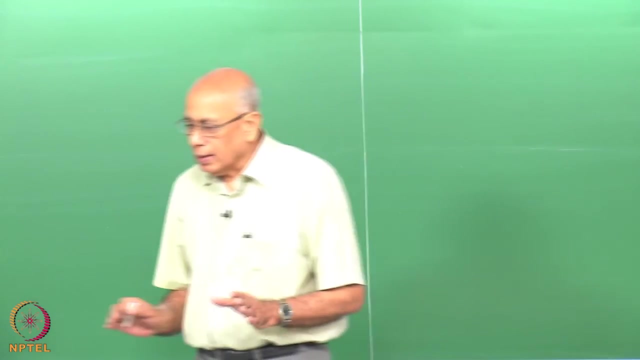 container and its velocity is some value v and it is in equilibrium. and this is an unconditional density, in the sense that I don't say what happens, what the initial value of this velocity and position variables are, or anything like that. I simply say I pick a particle at random. 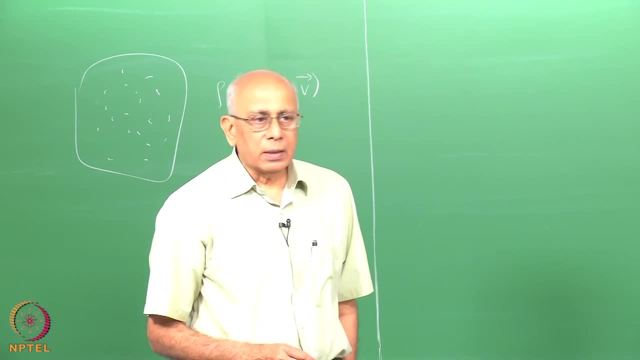 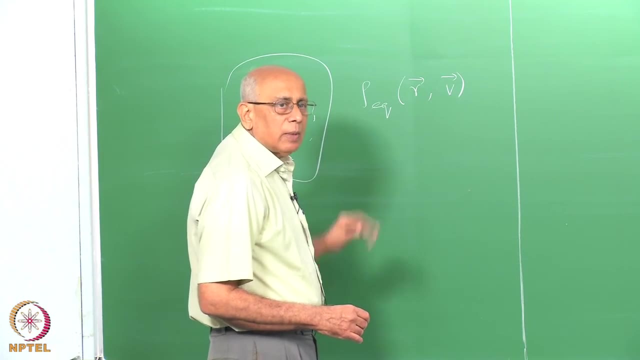 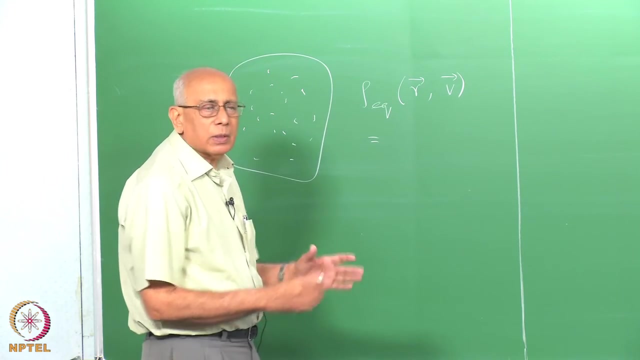 and I ask: what is its equilibrium? phase space density. Now, this is intuitively clear, that equilibrium statistical mechanics, of course, provides an answer. but it is intuitively clear what the answer is As far as the position variable is concerned, the density is absolutely uniform. It has. 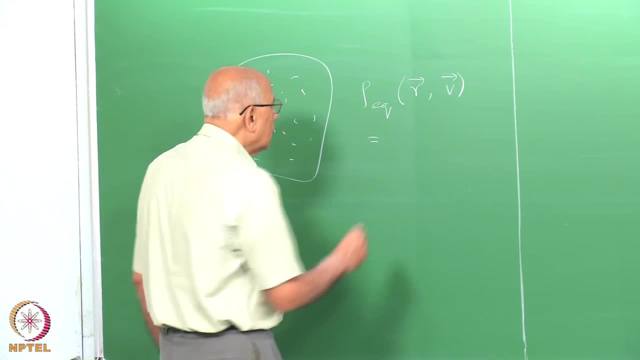 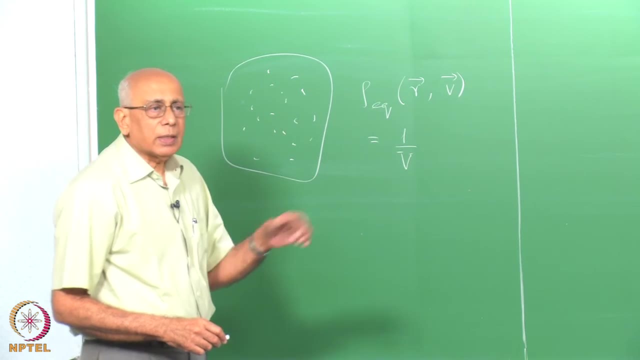 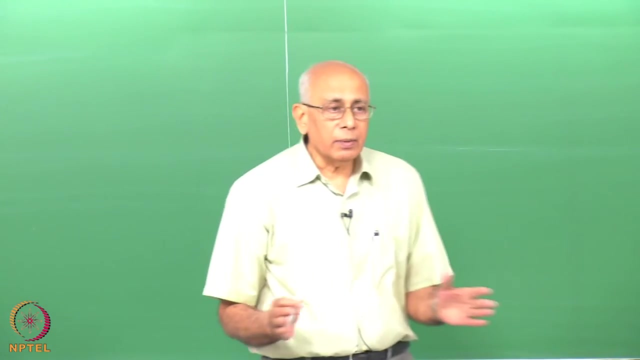 got an equal probability of being anywhere in this entire volume. So this is just a 1 over the volume. and then there is a portion which tells you how the velocity is distributed, and we know then that since the energy of this particle, if it is ideal, it is not interacting. 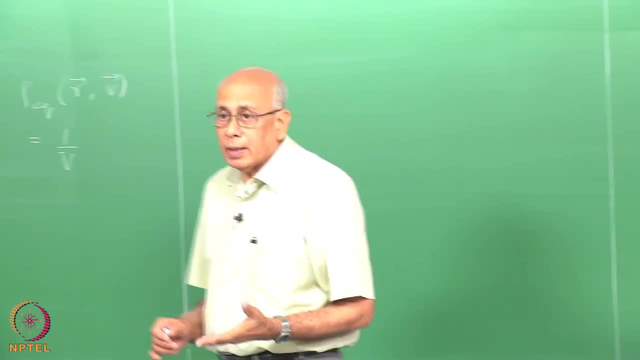 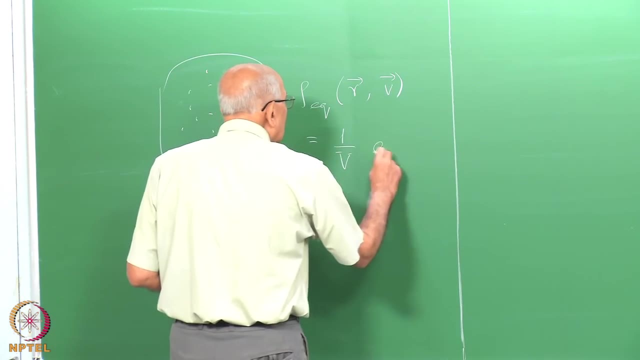 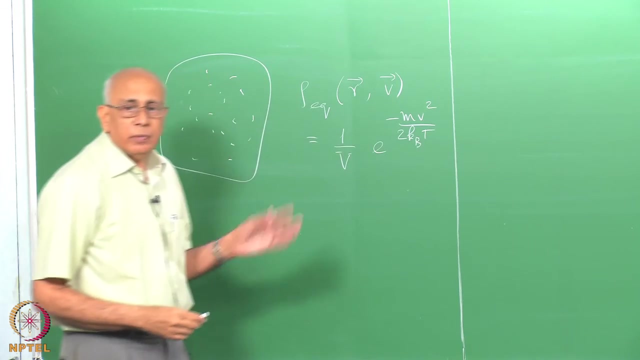 with anything else. The energy of this particle is just its kinetic energy. So it is just its kinetic energy. So it is just its kinetic energy. And the system is in equilibrium at some temperature, inverse temperature, beta. So this is equal to e, to the minus m v squared over 2 k Boltzmann times t, because 1 half m v squared is its. 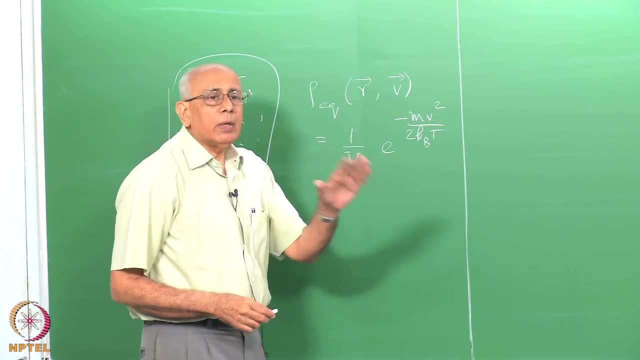 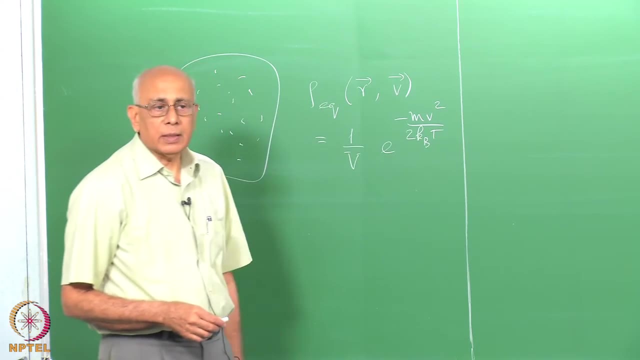 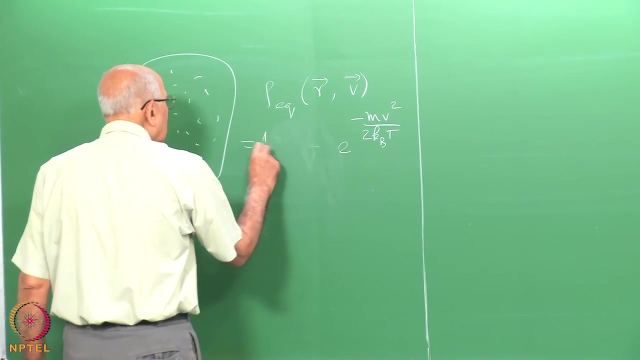 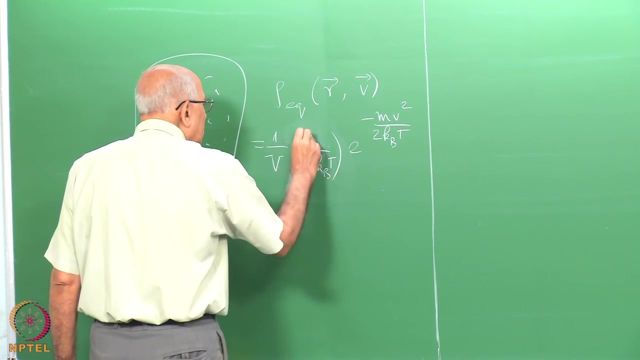 energy, just the kinetic energy, And the rules of equilibrium. statistical mechanics tell us that this is the density of particles, apart from a normalization factor, And of course we can write the normalization factor as well. So this is equal to 1 over v, m over 2, pi, k, Boltzmann, t, and there are 3 of these degrees. 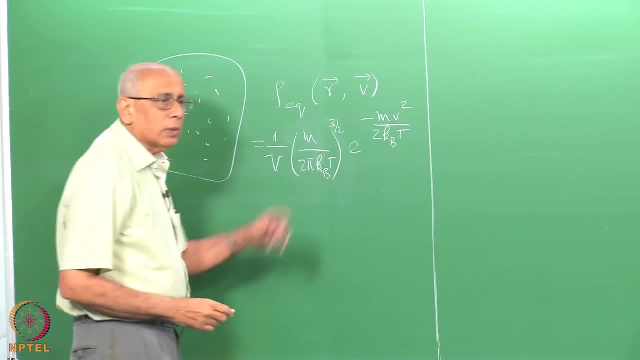 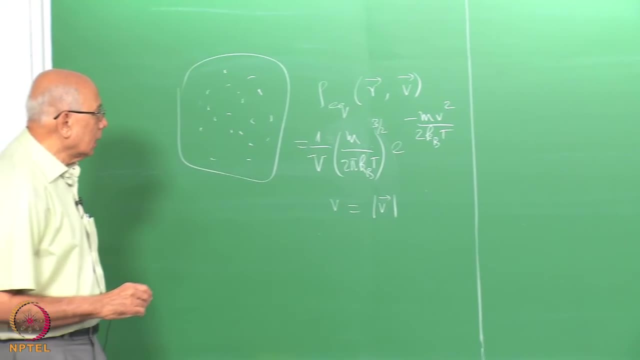 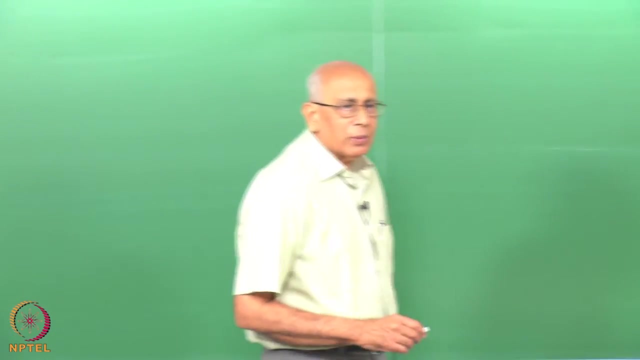 of freedom. so this is 3 halves times this quantity here where v stands for modulus of the velocity vector. Ok, So that is the phase space density in equilibrium. But right away we can ask a more complicated question. We can ask what happens if I take a single particle. 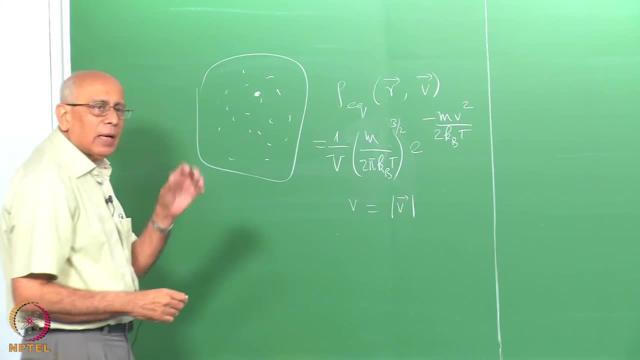 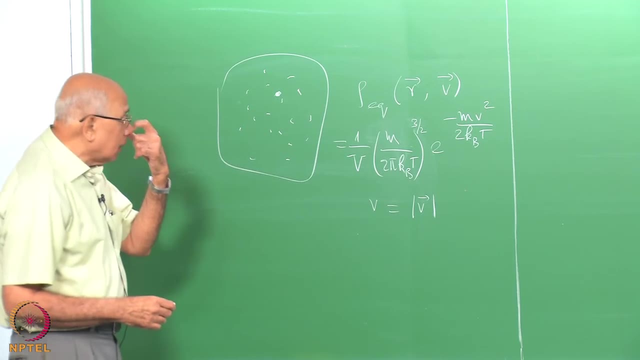 and I somehow manage to tag this particle. I am going to keep track of it and we are working in the level of classical mechanics. So I tag this particle and I look at it by saying, look at the instant of time when I take a look at it, it's got some position. 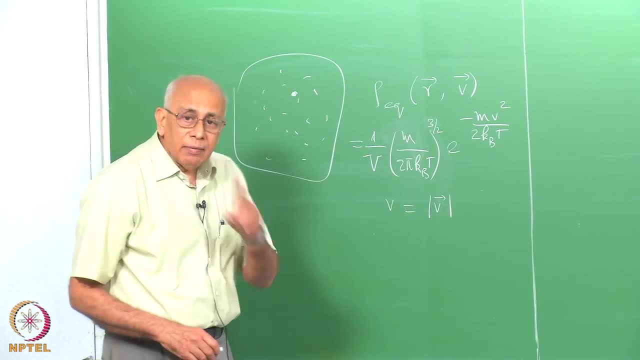 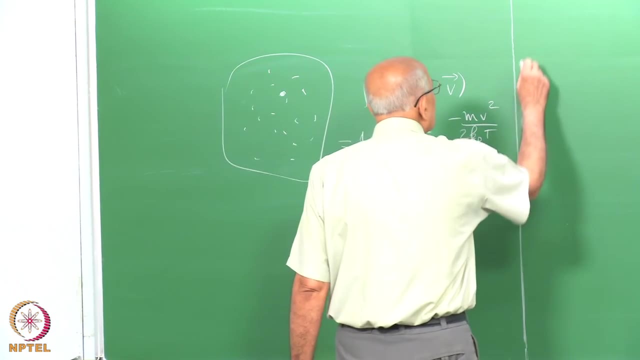 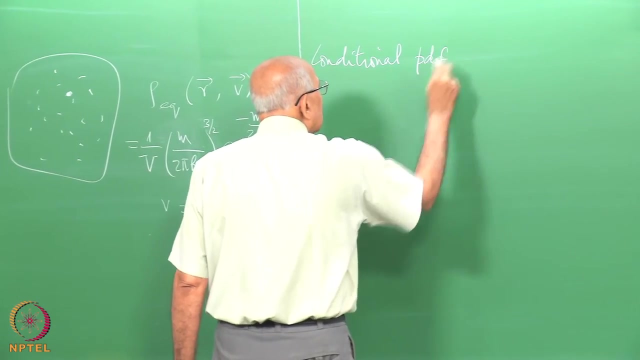 r naught, some velocity v naught, and then I, given that, I ask what happens to it As a function of time. Ok, So now I ask for the conditional probability density function, for which I will continually, let me, let me write it as capital- conditional probability. 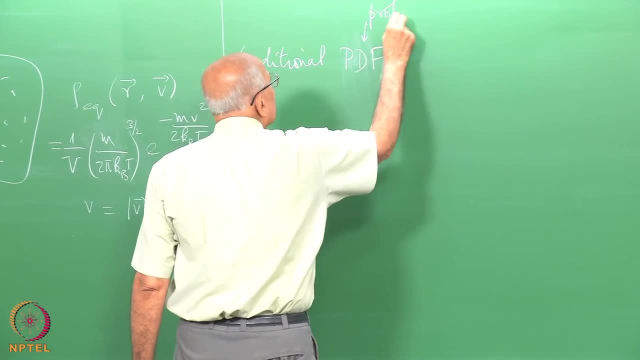 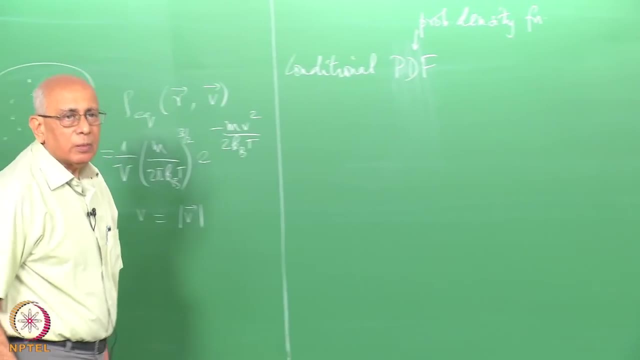 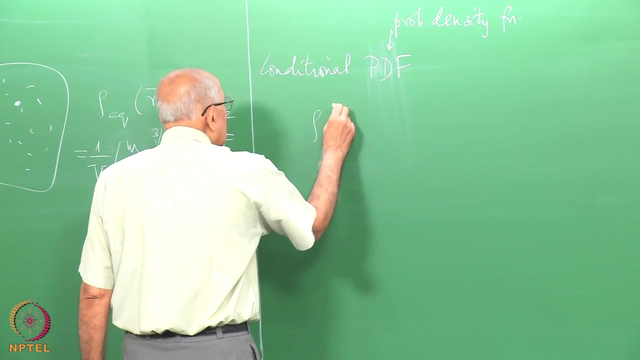 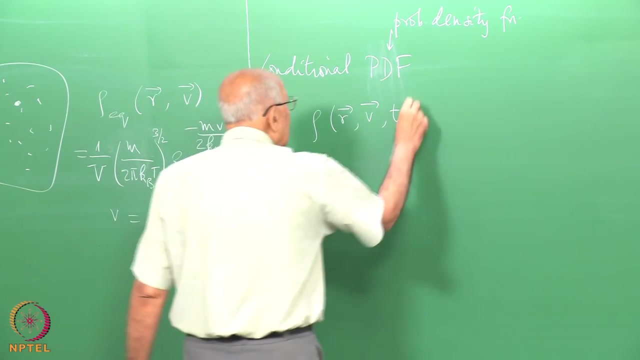 density function. I will use the abbreviation pdf for it throughout it- And I ask for the conditional probability density function rho, such that its position is r, its velocity is v, at some time t, given that it was some r naught, v naught and at. 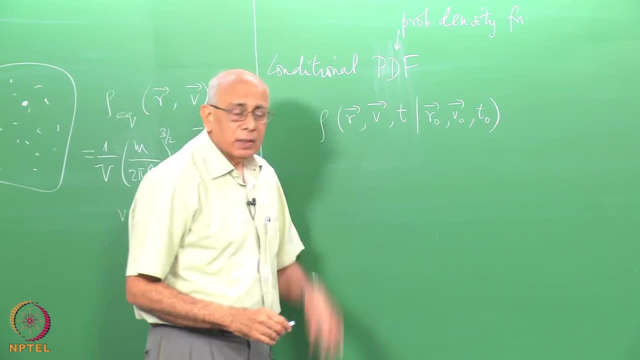 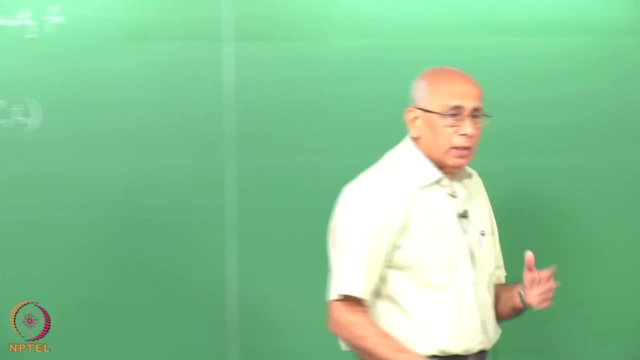 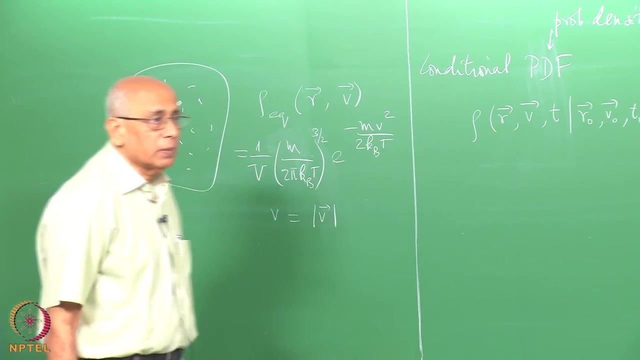 time t naught. So this is the conditional density and I ask: what's this quantity equal to? Ok? So r naught and v naught could be any arbitrary values which are allowed. And I say, given that condition, what is it going to do as a function of time? Well, what? 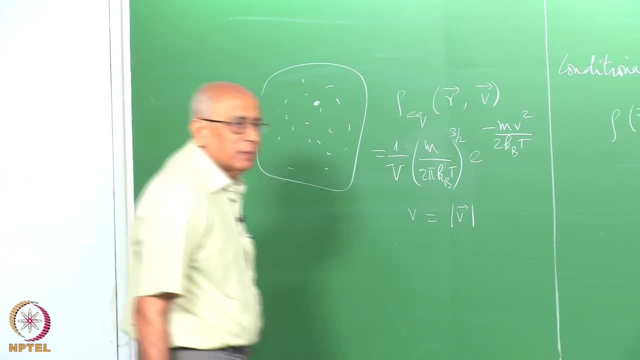 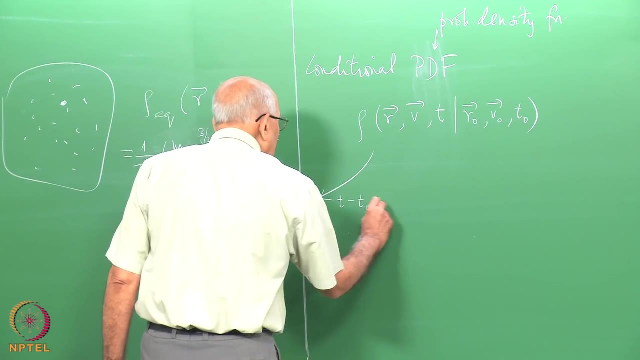 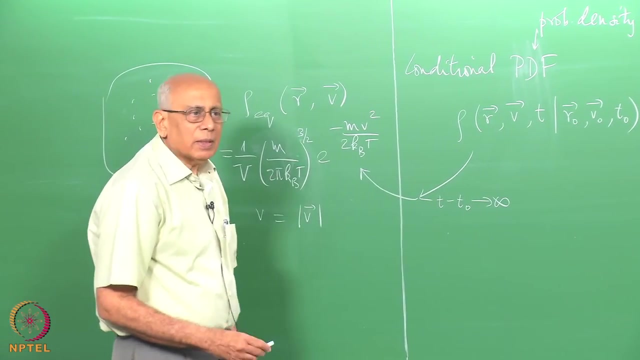 we do know intuitively is that as time elapses, as t minus t naught tends to infinity. so I expect that if t minus t naught tends to infinity, this thing will actually tend to the equilibrium density, because the system is not going anywhere, it's in equilibrium. 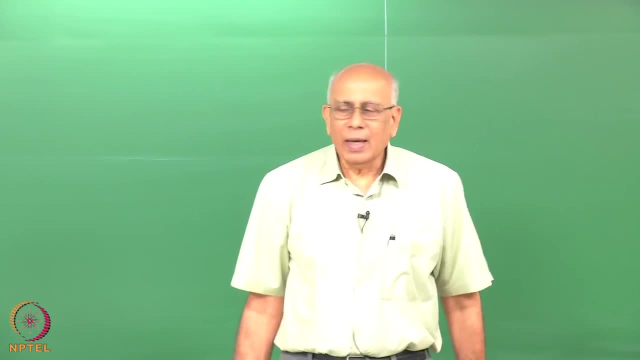 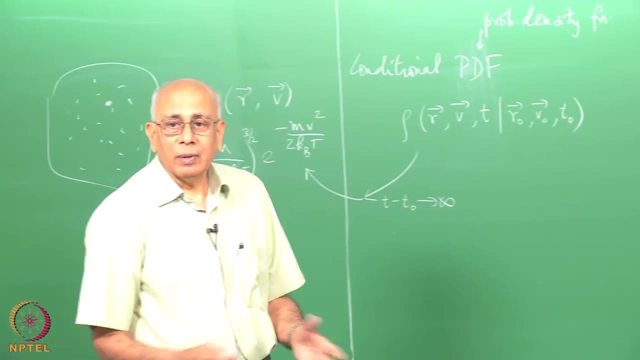 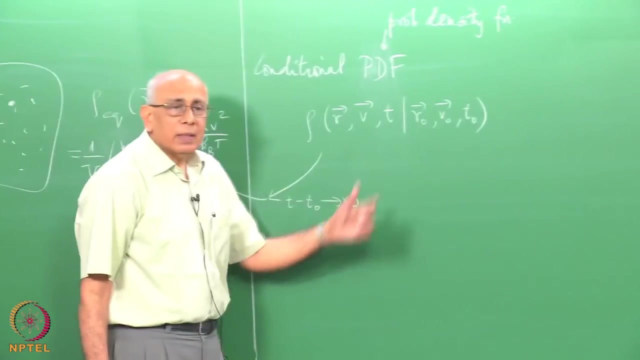 and I expect physically that, I expect intuitively that if enough time elapses since the time I measured the initial conditions, this particle will relax to equilibrium and attain the equilibrium density. It will lose memory of what its initial values were of these variables and it will tend to this quantity. 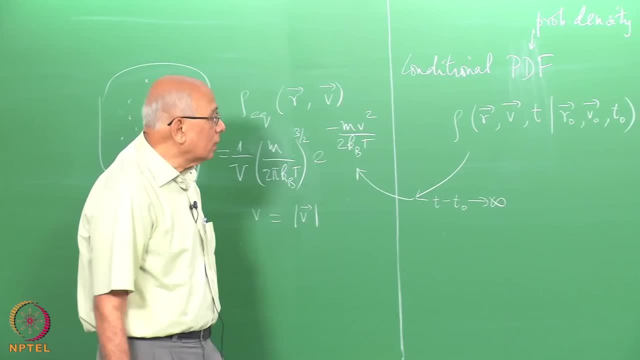 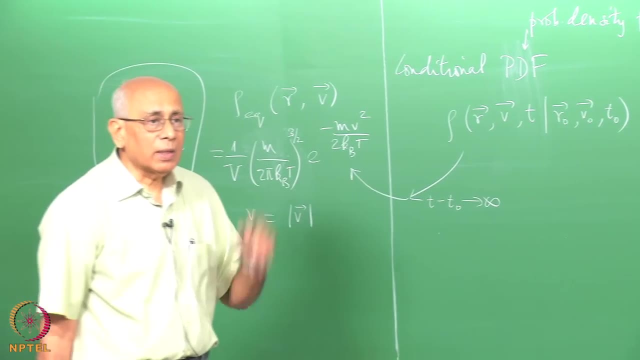 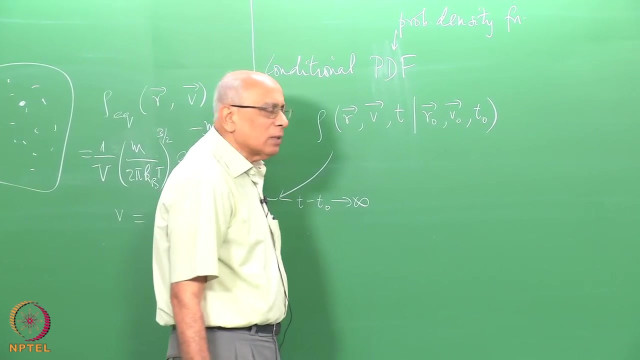 here, Ok, But the hard question is now: what is it, as a function of t, for arbitrary values of t, and not necessarily t minus t, naught into infinity? Ok? Well, it's again sort of clear, and we haven't established this, but it's again clear that 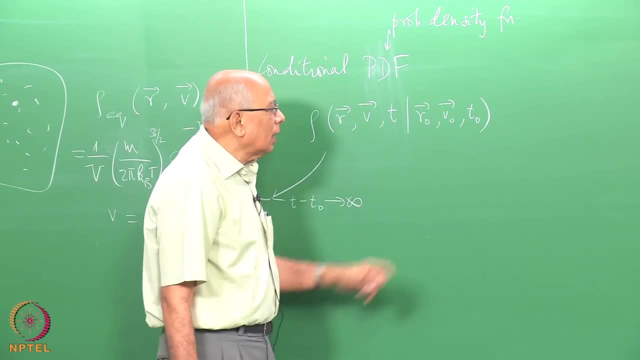 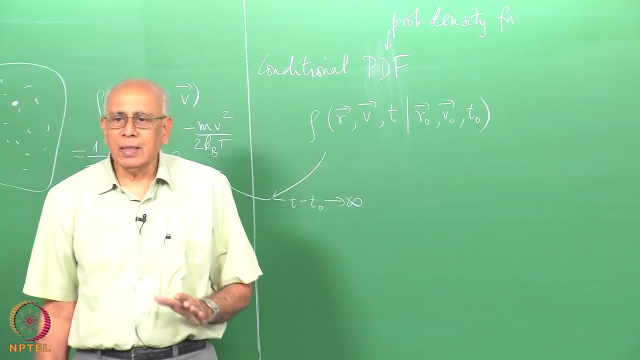 if the system is in thermal equilibrium, then it doesn't matter when I start this t naught and that this whole quantity will be a function only of t minus t naught, only the elapsed time, because when I start the clock is completely irrelevant since the system is already in. 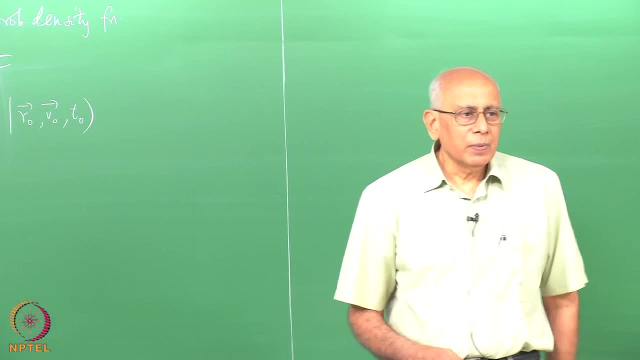 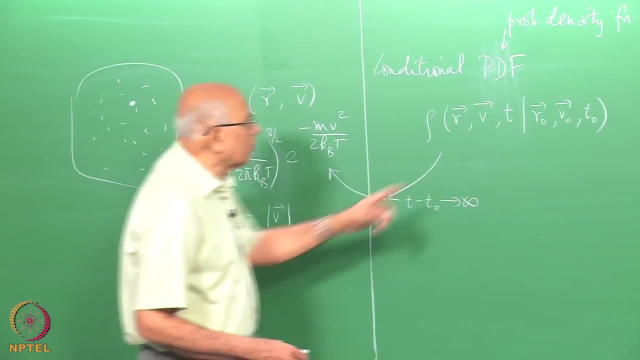 equilibrium and the process is stationary, So I don't really have to ask what is the system of t plus t If I specify? specify any particular t naught. all I have to worry about is the difference between t and t. naught the elapsed time, So I might as well set t. 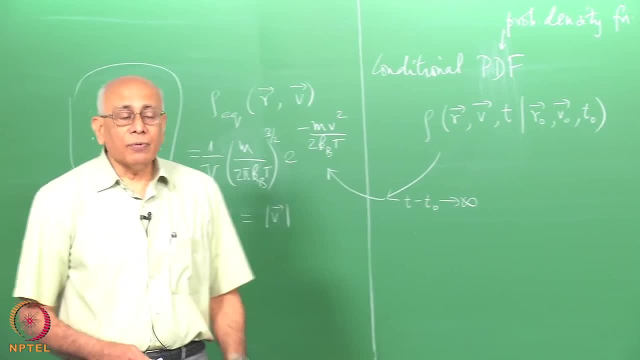 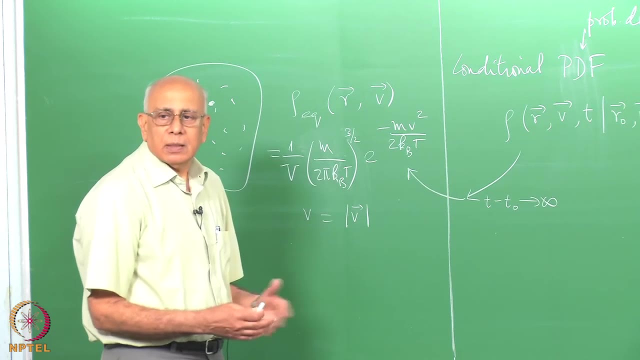 naught equal to 0, right, I'll often do that. we'll often do that, assuming this system, if it's in thermal equilibrium, has no time dependence of any kind. So the time when you start the clock and measure the initial condition is irrelevant. 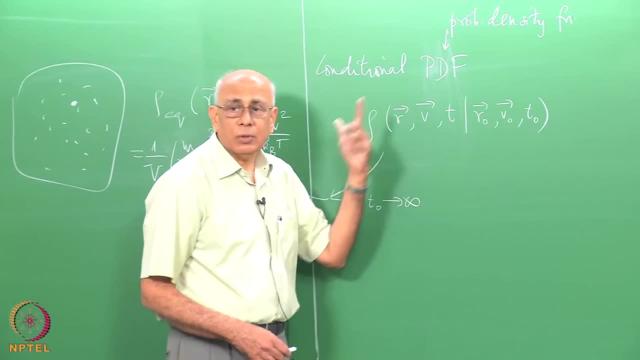 But the hard question is: what is this function as a function of t? How does it turned into a mass, to a mass? Is the mass the space, the rainbow? Basically, I gave it out because the mass I gave it out just for the means, But the main point out there is that we orheits 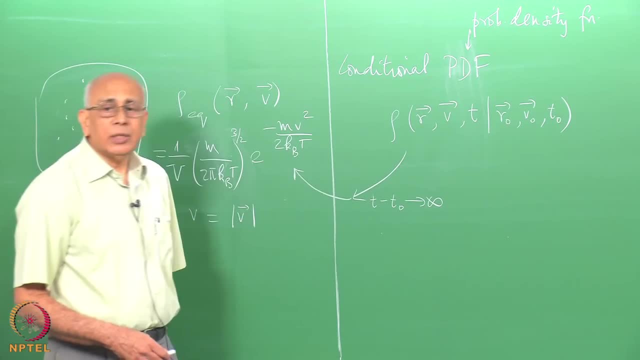 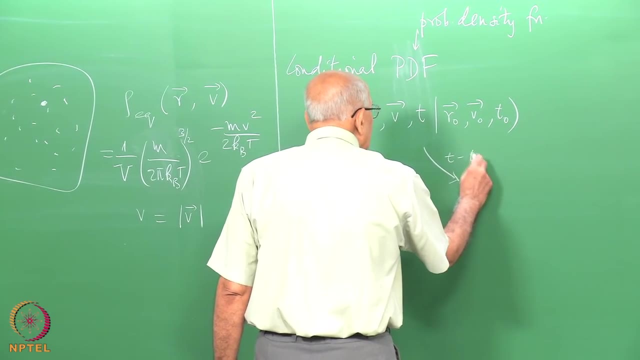 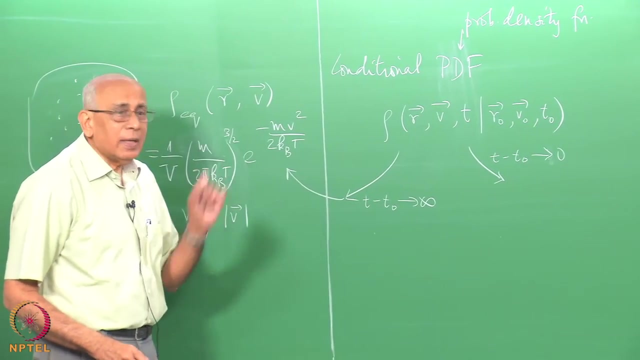 it reach this because I know what its value is initially. I know what its value is not as t minus t not tends to infinity, but as t minus t not tends to zero. In other words, at the instant, t equal to t not. what is this density? It is obviously equal to delta 3. 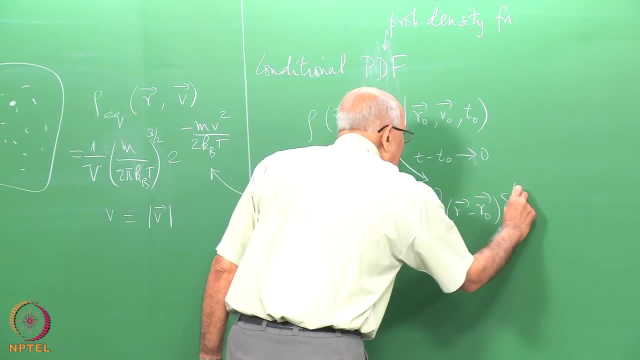 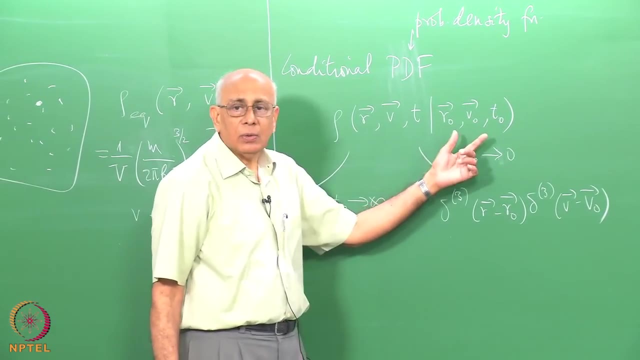 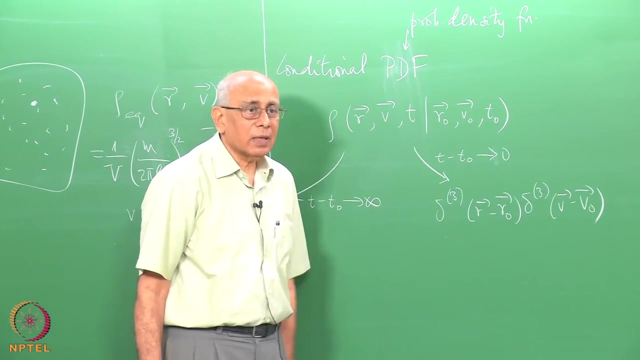 of r minus r, not delta. 3 of v minus v. not, because I am telling you that the values at t not time, t not, are these values deterministic values. So it starts off in this very spiked way, this delta function distribution, and broadens out or does something crazy: It becomes uniform. 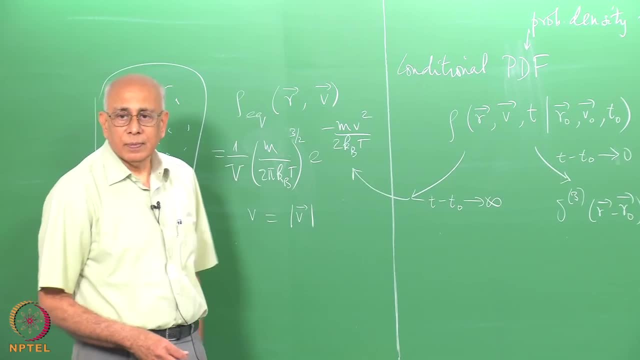 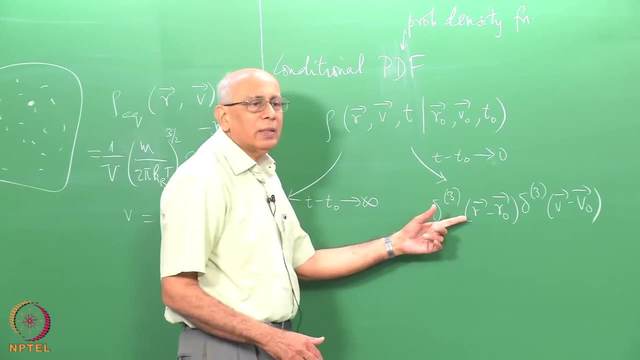 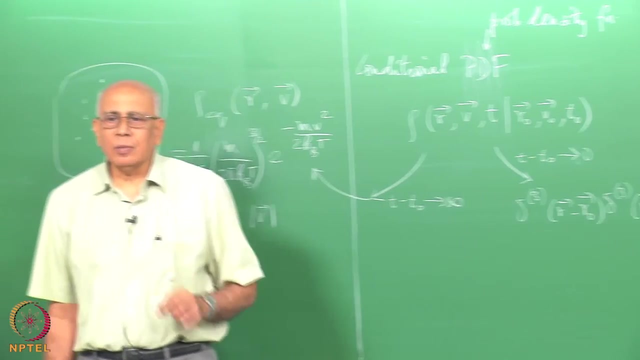 in space and in velocity it becomes Maxwellian, with the mean value of the velocity which is equal to zero. So I know the limiting cases, I know the initial condition on it and I know the limiting distribution, but I don't know what it is in between. Ok, That's a very hard problem. It turns out this: 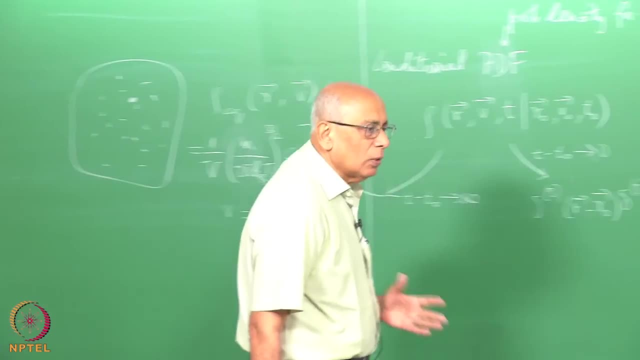 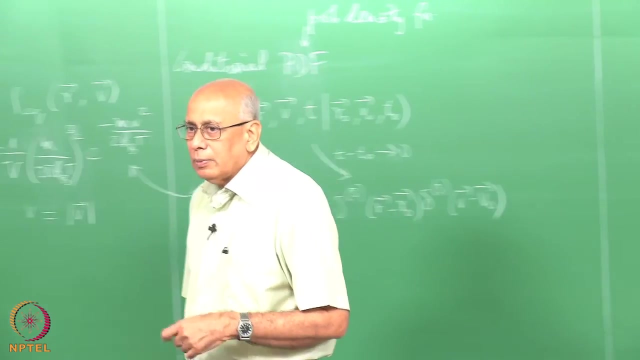 is a very, very hard problem. If you look at a realistic dense fluid, it's an extremely difficult problem to answer because these particles are in interaction with each other- to start with number 1- and they are correlated with each other, So there are all kinds of 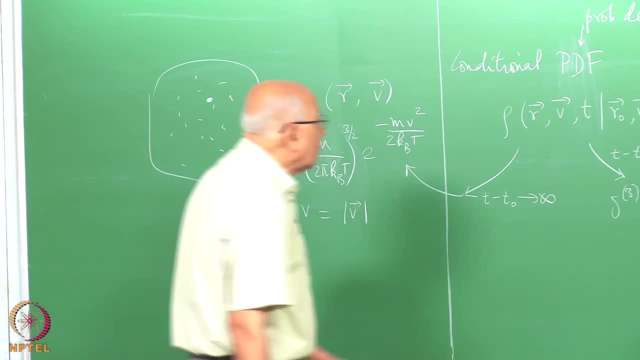 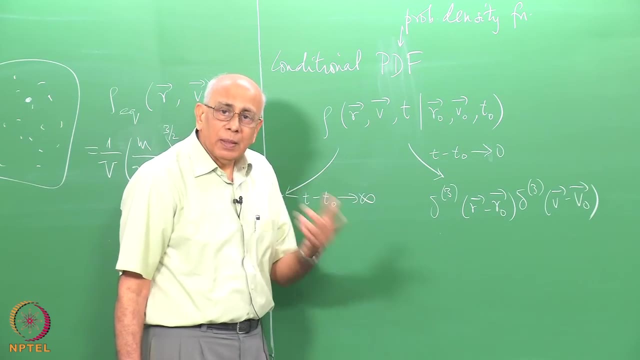 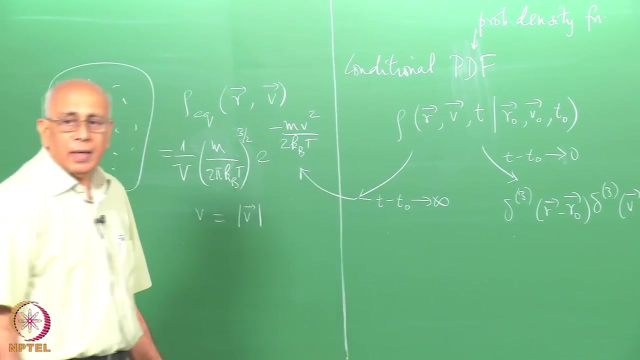 correlations. There are correlations between the particles in such a way that you cannot write a single equation, closed equation for this variant, this density. It gets coupled to two particle distributions, three particle distributions and so on, in a well-defined hierarchy. And this hierarchy is a never-ending, it's not an ending hierarchy, It doesn't for a finite. 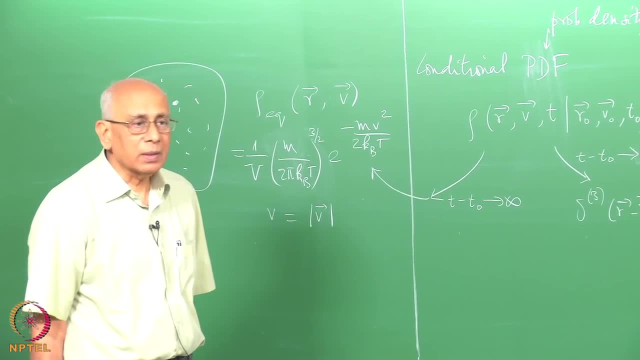 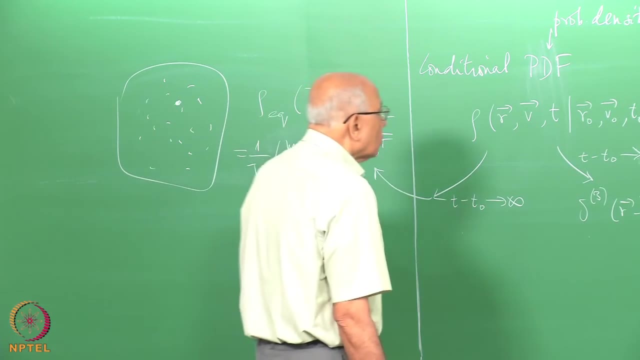 number of particles, it will end. but, of course, if you have an infinite number of particles in the thermodynamic limit, this hierarchy is not a finite set of equations. Ok, So I think it's a very hard problem. So already you begin to see that this is a very, very hard problem to start with taking 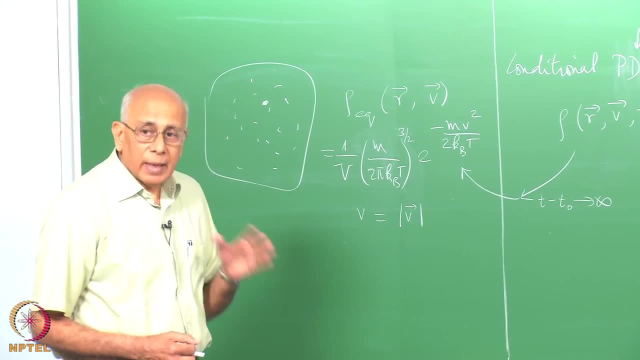 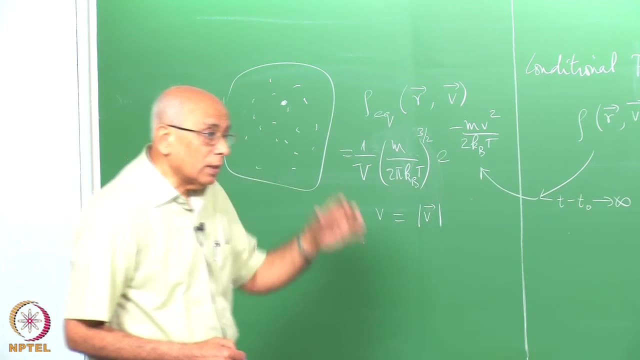 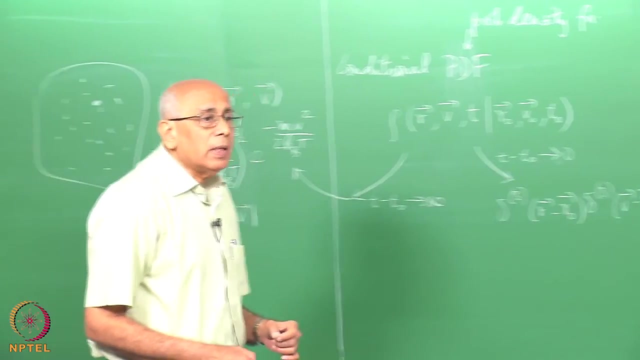 into account all the possible correlations. And if these are quantum mechanical objects and you have to impose, for example, symmetry or anti-symmetry in the wave functions, if you say that these are fermions or bosons which obey certain kinds of quantum statistics due to indistinguishability, then it becomes even more hard. It's a very hard problem. 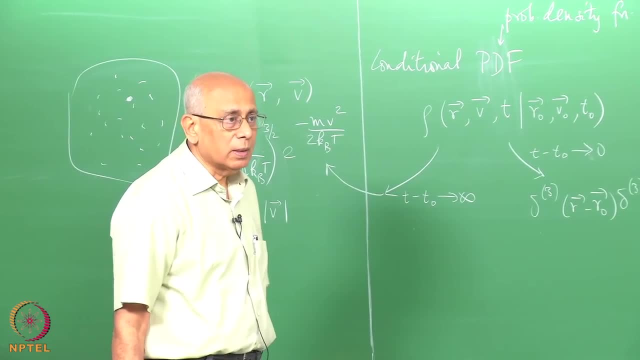 in many-body theory and we are certainly not going to get towards that. So I think it's a very hard problem. It's a very hard problem in many-body theory and we are certainly not going to get towards that. So let's look for a simpler problem to solve, a simpler model to solve, where we get some. 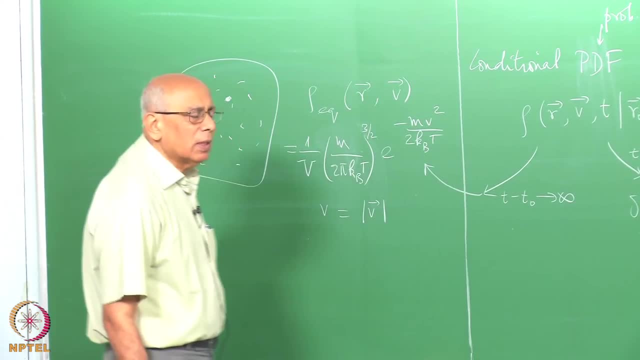 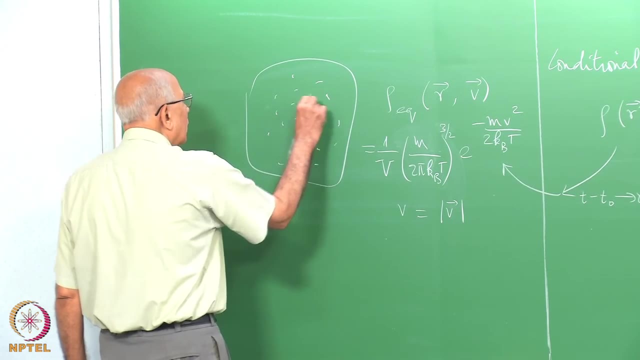 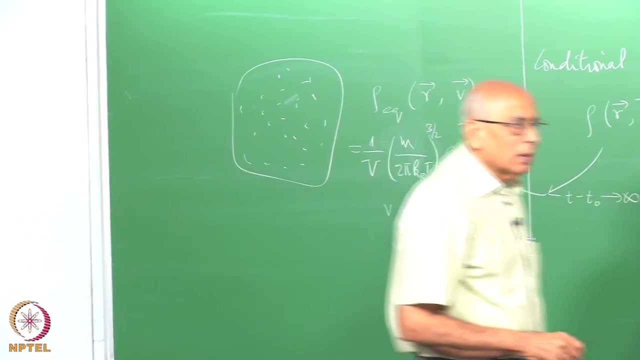 insight into how time dependence appears, And we will use physical guidelines to guide us through this problem here. So let's suppose that in this fluid, in this dense fluid, you have a few much bigger particles, a few tagged particles, colloidal sized particles. So these atoms, these particles are of atom. 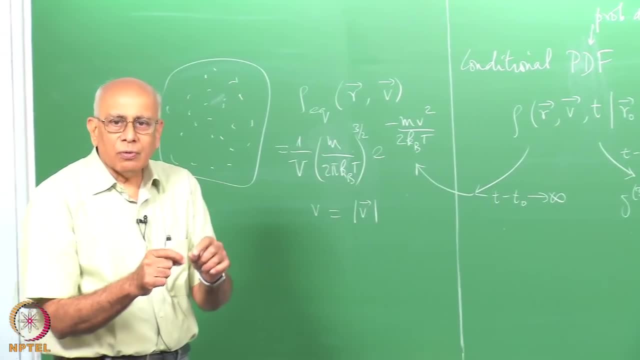 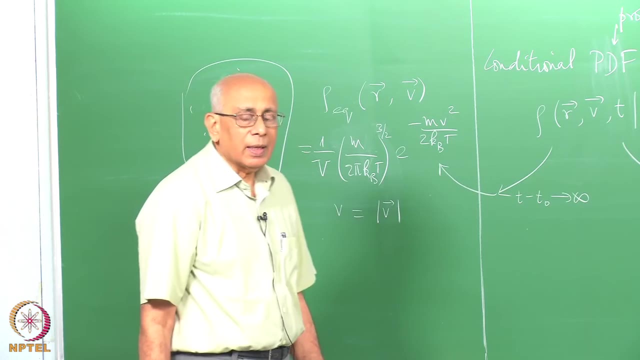 size, atomic or molecular sizes which are of the order of fractions of nanometers. But now let's put into it some objects which are, or a little smaller than that, but which are already several thousand times the size of atoms, individual atoms, right? So let's. 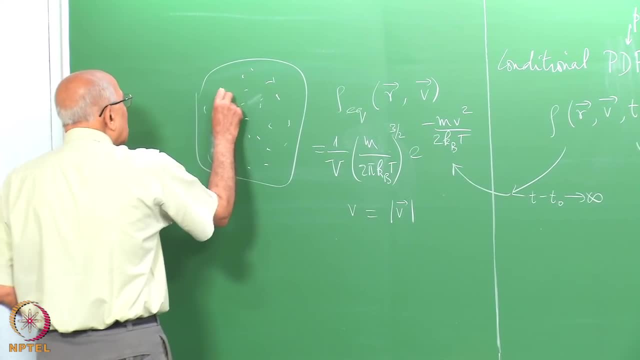 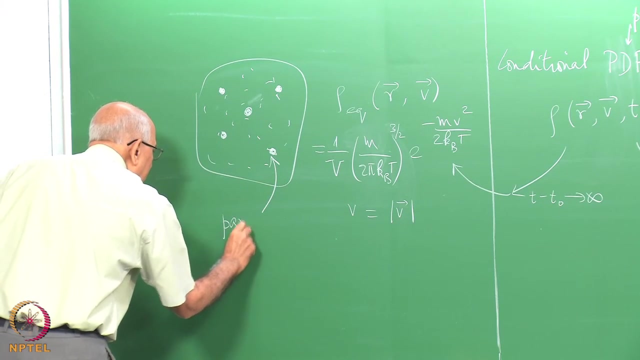 call those the tagged particles. I mean, let's call those the larger particles. I will use little circles for that- and let's put a dilute concentration of those things. So this is a much bigger particle. So these are much bigger particles with individual masses which 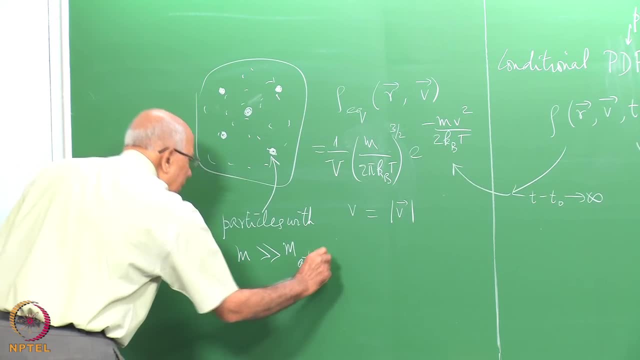 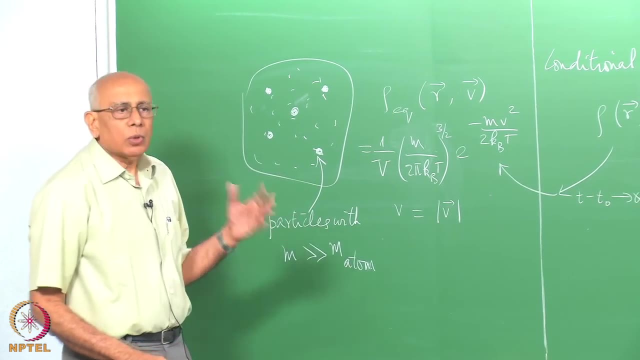 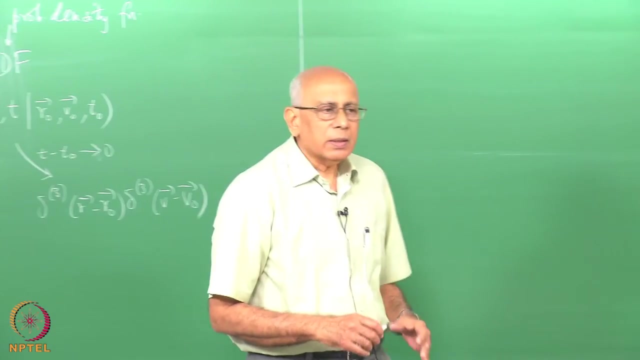 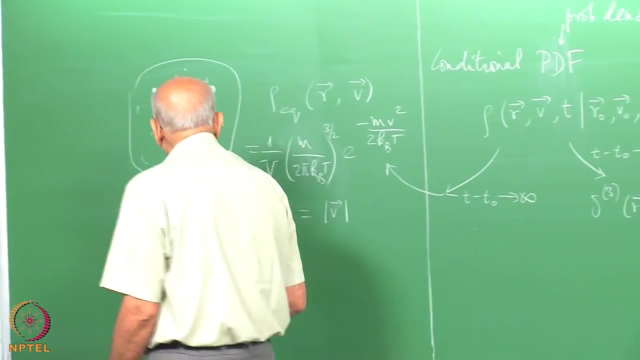 are much, much greater than m atoms. They undergo Brownian motion in this fluid. They have moved about from side to side, they jolted about, they have very jerky motion because they are being buffeted constantly By these little tiny particles, the atoms or molecules. Ok, We will also assume that. 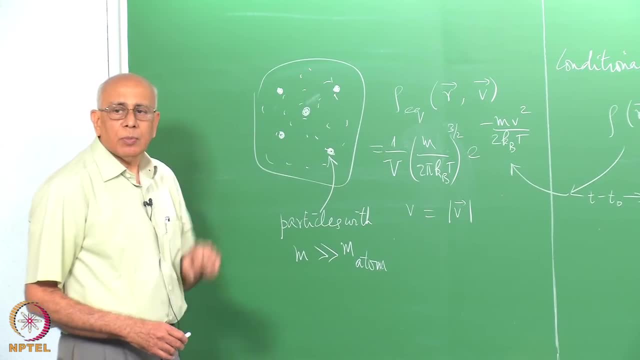 the concentration of these objects is sufficiently small that they don't interfere with each other. So essentially we can treat each one of them in isolation. So that's the second assumptions. The mass assumption will appear in a very subtle way and we will see exactly. 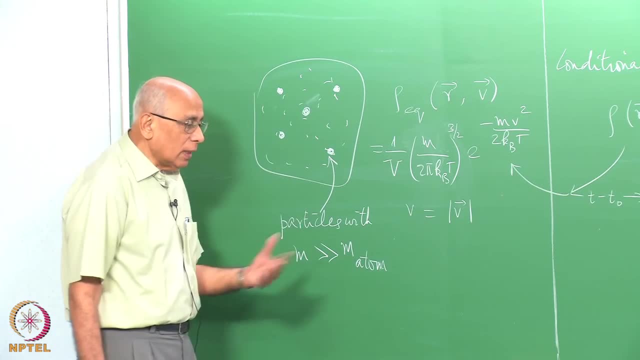 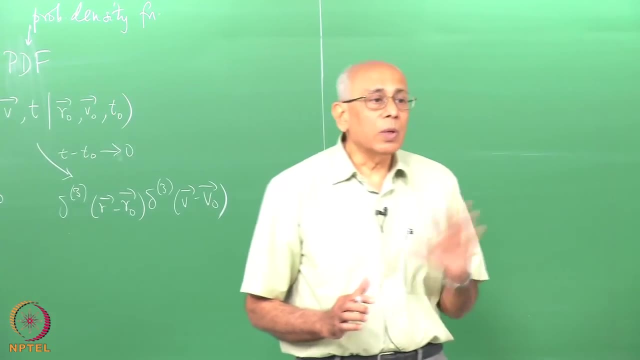 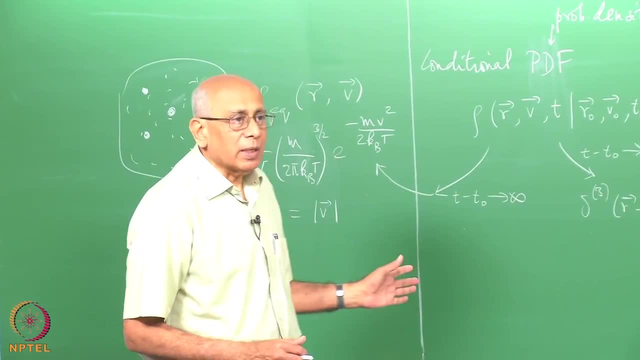 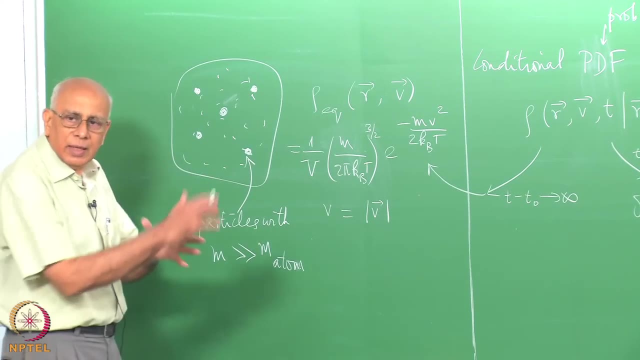 particles would be micron sized and the other fellows are angstrom sized. Ok, so many orders of magnitudes separate them. and the question is: will these particles get anywhere? obviously they're going to stay there, get bounced around, etc, etc. and let's see what happens to the 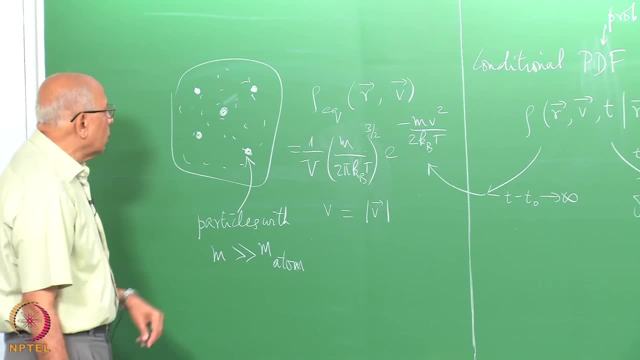 motion of these particles here. Now, what we can do is one of several things We could try and find out. of course, how do we get quite a lot of wyondble? Let's just forget the vidéos for my time today and good bye. 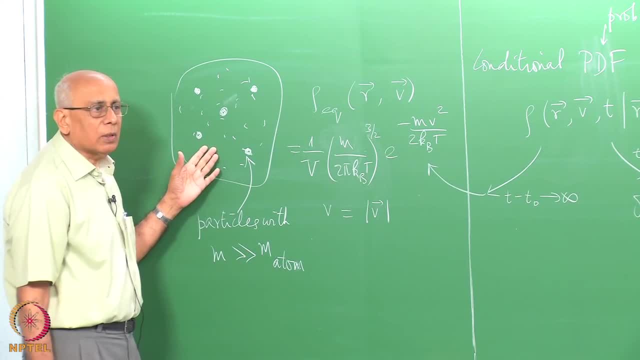 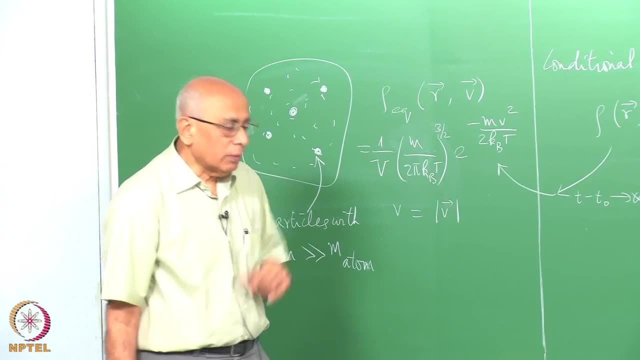 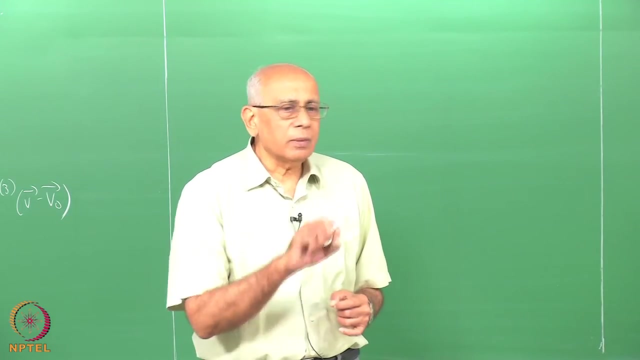 Since we want to know what the distribution and velocity in particular, of these particles is, we could try and find out what the actual probability density function of the velocity does as a function of time by writing a little model for it, making some assumptions about the way in which the atoms bombard this big object. Alternatively, we could start with 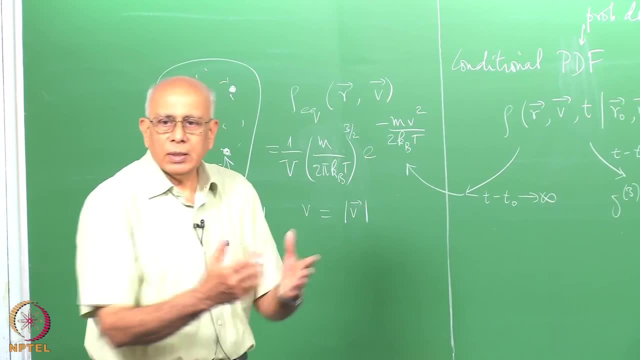 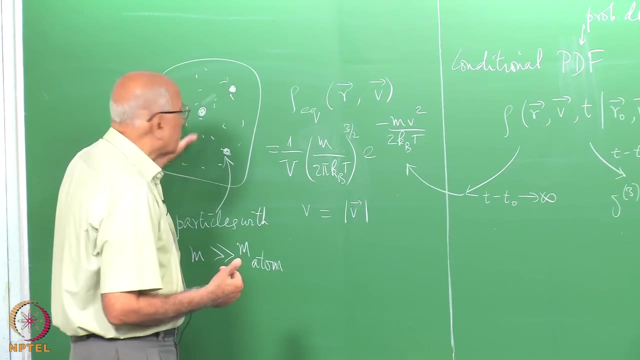 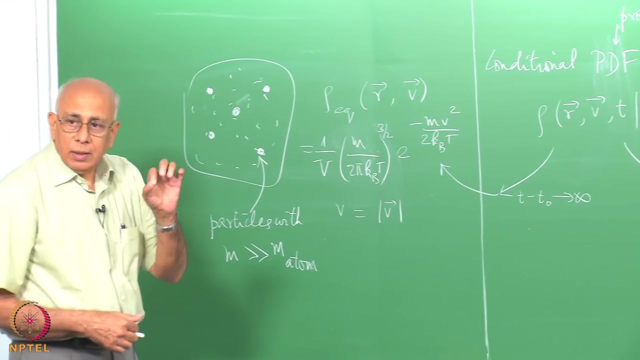 the equation of motion. We could guess an equation of motion. use Newton's equation for it, for instance. write down this equation of motion but take into account the random forces due to all these other particles which we cannot compute, which are completely random for all practical purposes, by using a stochastic equation for this particle and making suitable 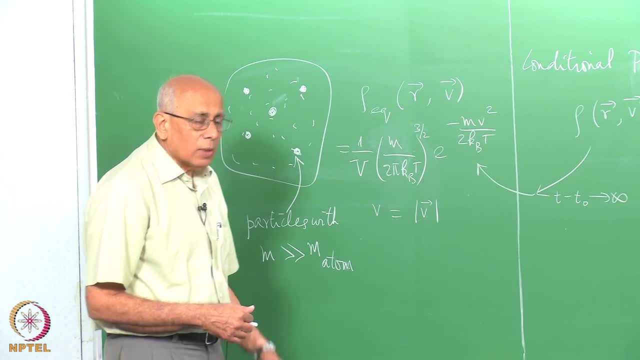 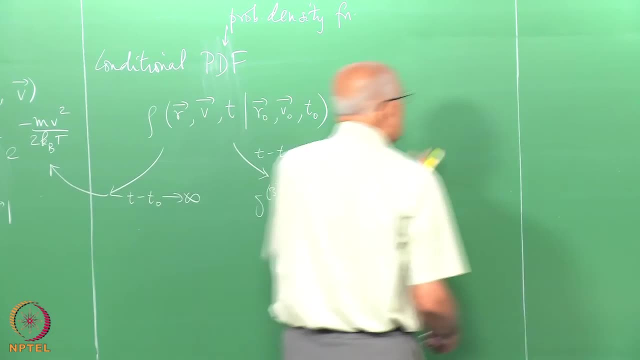 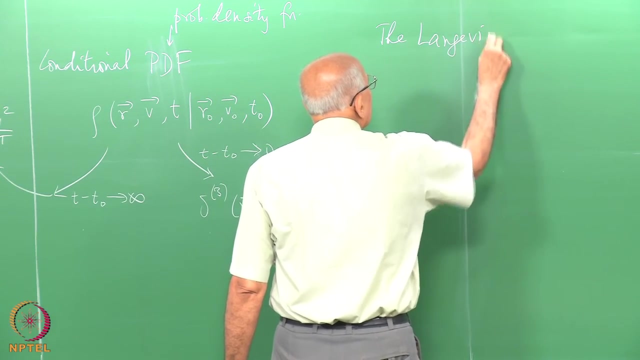 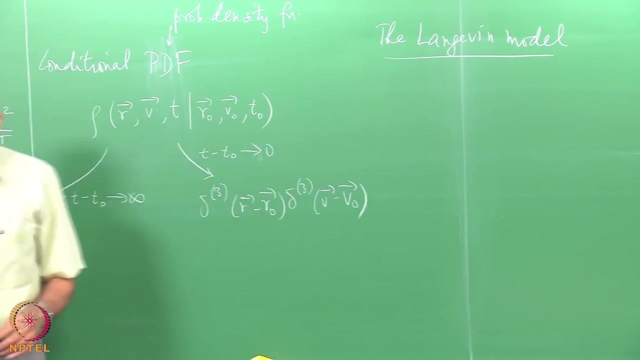 assumptions about the nature of the noise. Ok, So let's use that. We try to do both, but let's write this down to start with: the equation of motion, and this is called the Langevin model. It won't be apparent in the beginning where this assumption has gone in. That's a little. 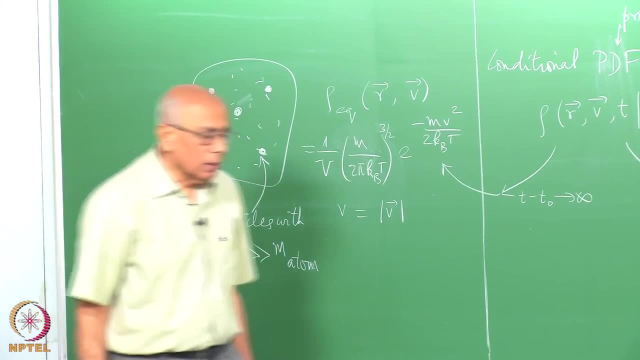 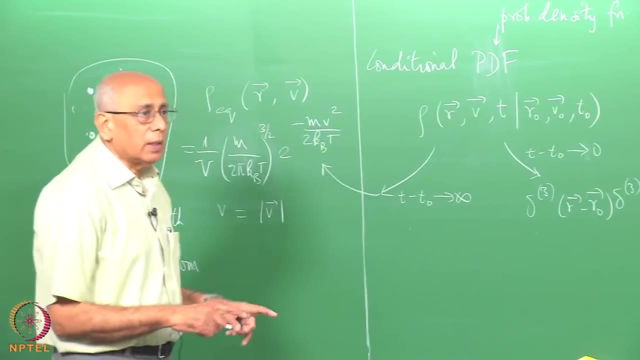 subtle, but we will see how this figures a little later. We will run various consistency checks and we will see that you need this assumption. Otherwise, it's not true, for the reasons I mentioned earlier, Namely if you are looking at the atoms themselves and 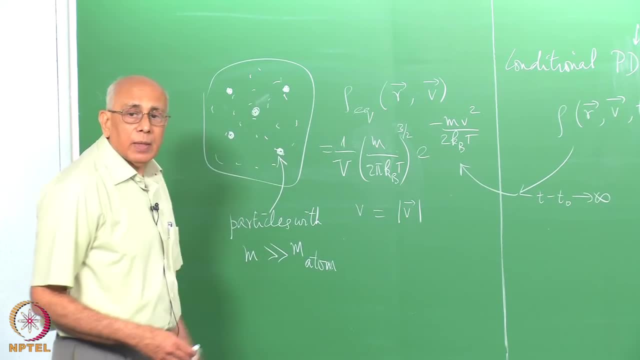 one of the reasons why I mentioned earlier, namely if you are looking at the atoms themselves. one of these particles is one of the atoms themselves, then it's got all kinds of correlations with the other particles and you can't write a simple one. body phase, space distribution. 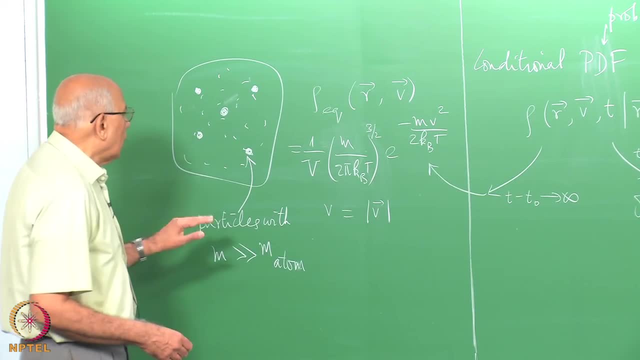 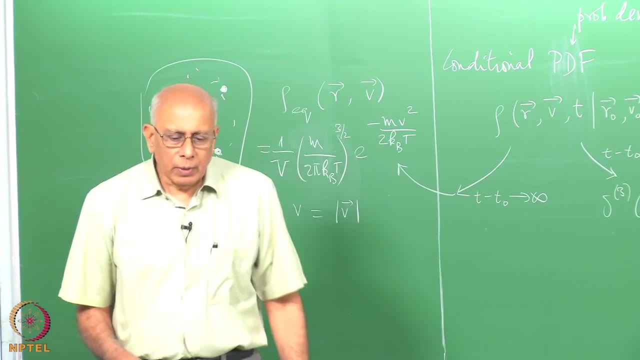 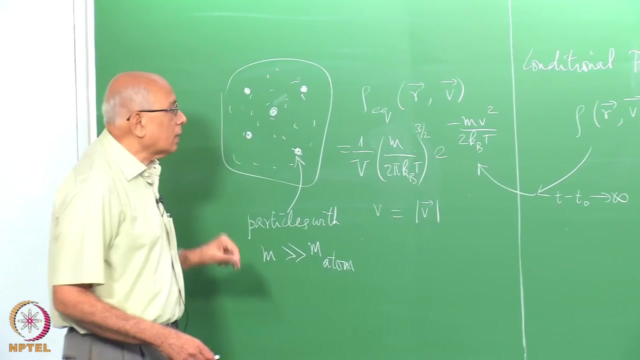 function. Ok. So we keep that in our mind and we now write down something for this equation of motion, for this, And let's make life very simple. to start with, We will assume that this system is again in thermal equilibrium, So these particles are also in equilibrium at the same temperature, except that they are. 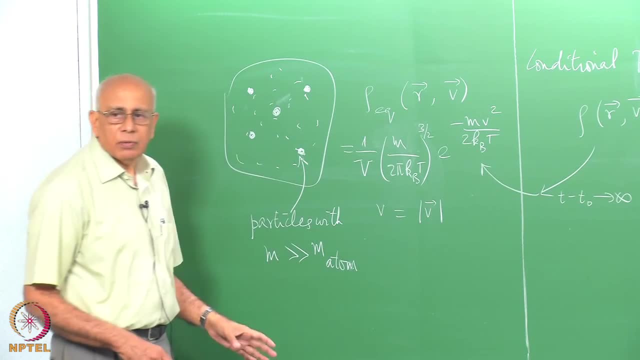 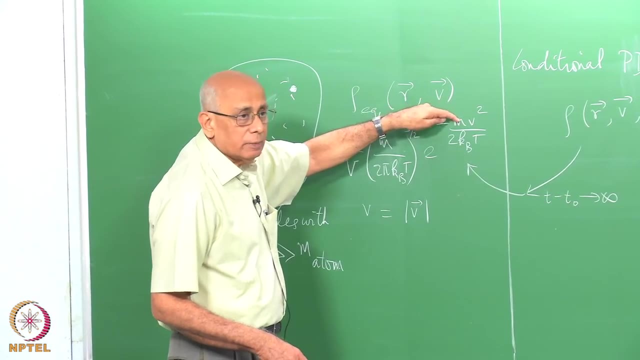 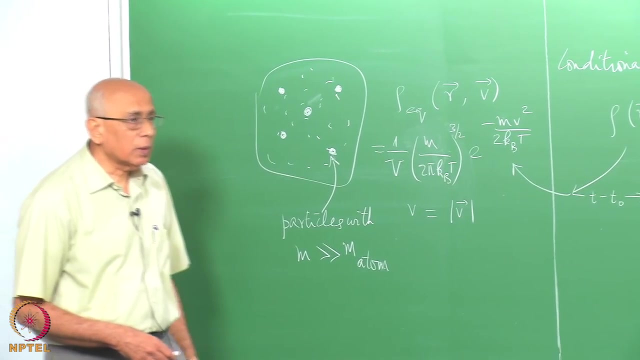 also uniformly distributed. We will neglect the effect of gravity for the moment, and the velocity distribution is Maxwellian, with this m here, where m represents the mass of one of these particles here, one of these large particles. Ok, So the heat bath is provided by the fluid which ultimately, 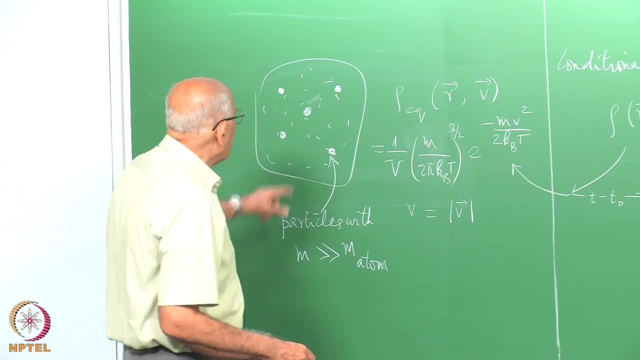 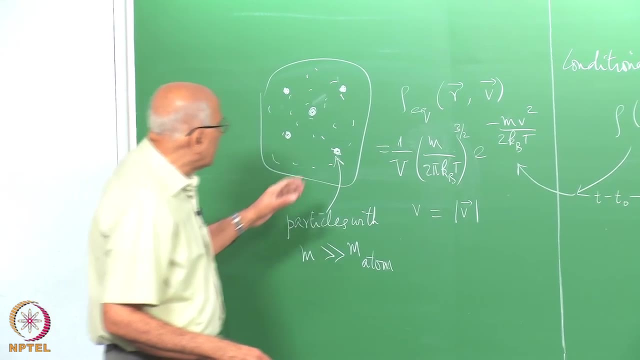 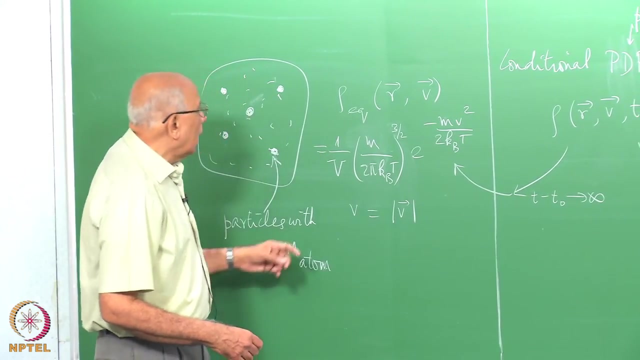 is in contact with the external world at some fixed temperature and these particles are in thermal equilibrium. So in this fluid and their distribution, function and velocity in equilibrium is the Maxwellian distribution. It's precisely this, And in equilibrium the position is also uniform. so 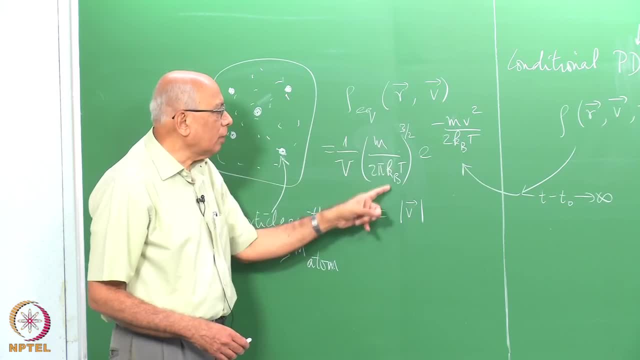 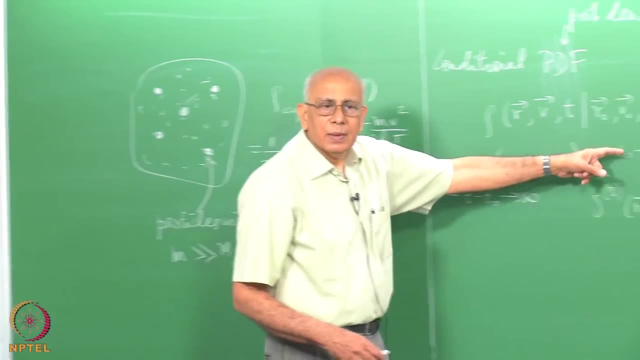 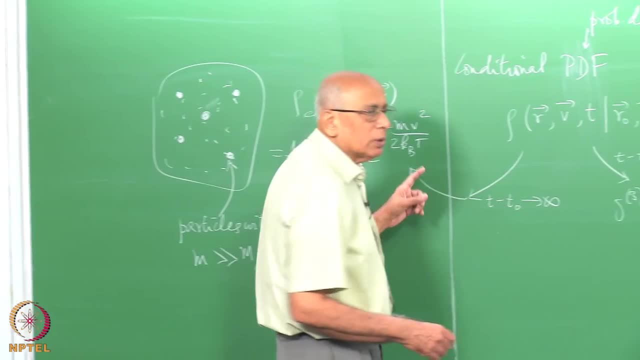 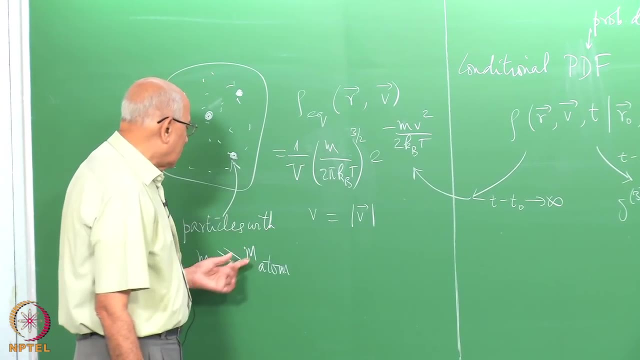 of t. How does it attain the Maxwellian distribution eventually? So it's exactly the same question: by little slate of hands. instead of writing m atom, I wrote this m for the large particle, and this is exactly the problem we have to solve. Yeah, 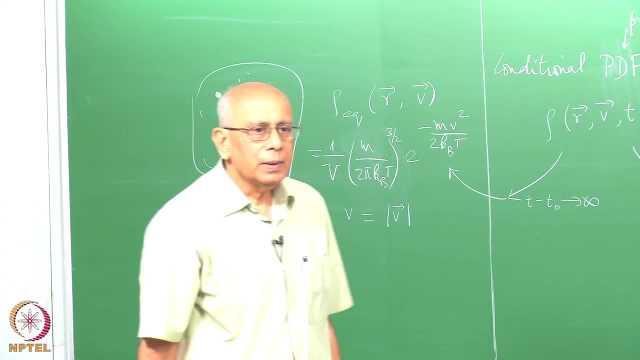 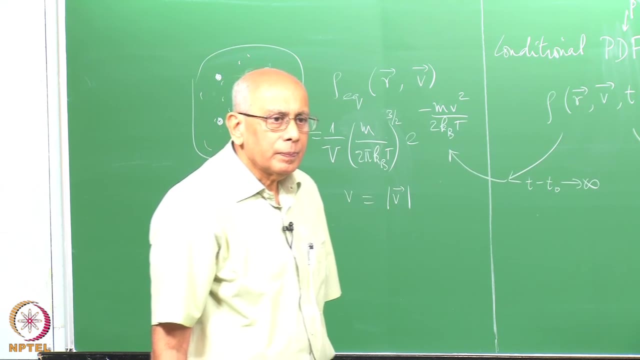 Since the density of the larger particles are very small compared to the bar, how do we define the temperature for such a low density matter? Yeah, A dilute gas. I can still define a temperature for a dilute gas. This is a good question. 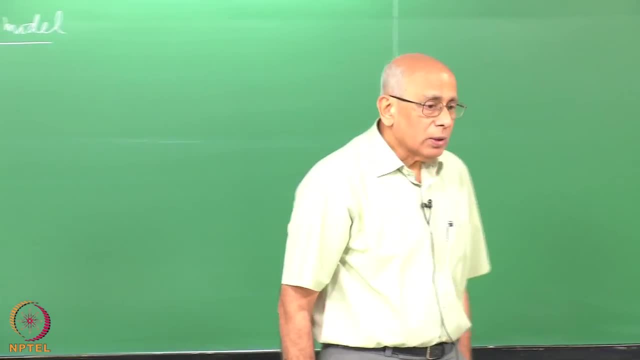 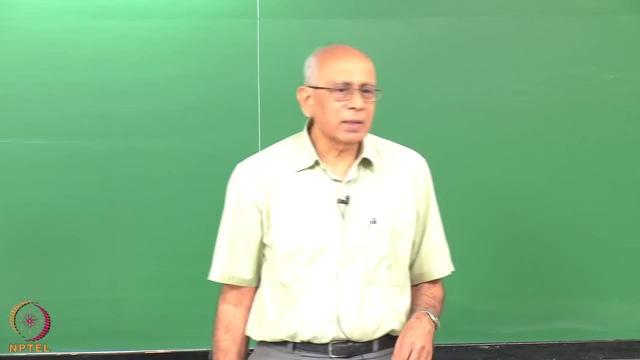 How do I define a temperature for one object, right? I am going to assume that its average kinetic energy defines its temperature, which it does In an ideal gas. that is precisely how temperature is defined, right. Temperature is a sort of wrong, is a sort of irrelevant. 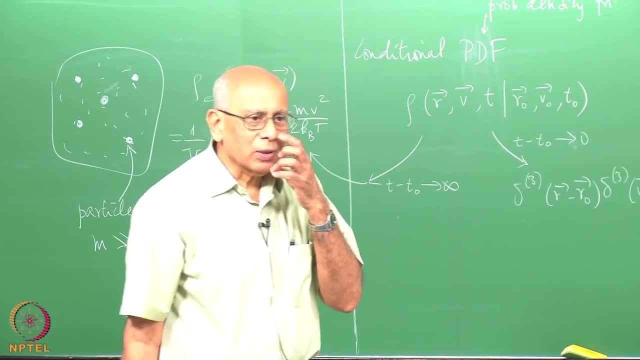 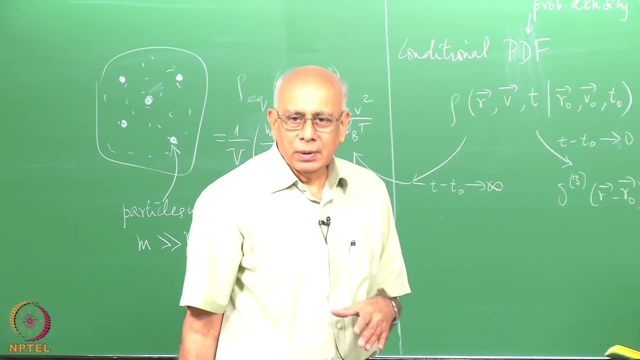 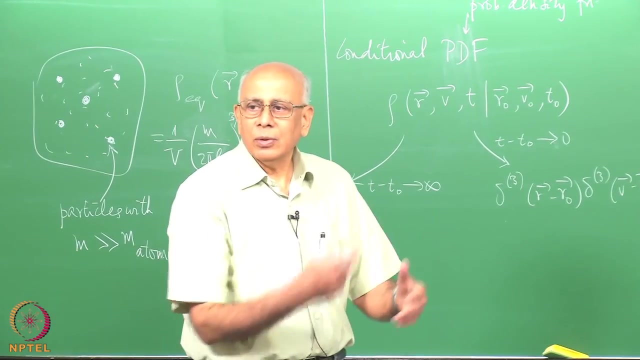 notion that we unfortunately introduced for historical reasons. Before the nature of what heat is was known, they didn't know that heat was random molecular motion, the energy of random molecular motion. Had we known that, we wouldn't have used another unit called temperature at all, and then introduced a Boltzmann constant to convert from one to the other. 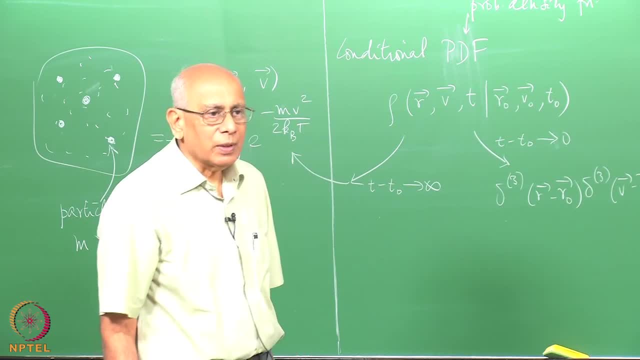 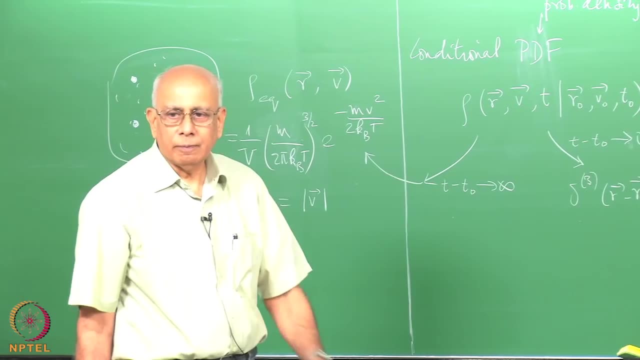 They have just called it average energy, and that would have been the end of it, right? So in that sense, I am going to say that the average energy of this particle, each of these particles, is 3 halves k T. Ok, right. 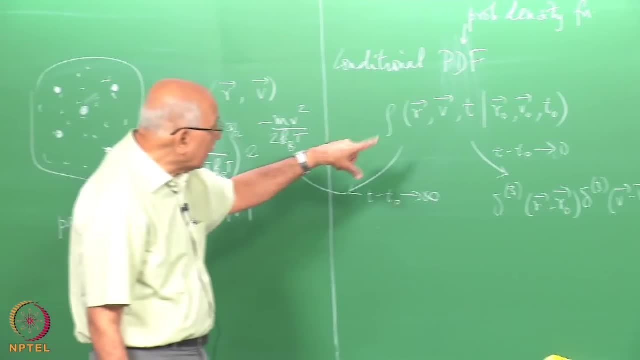 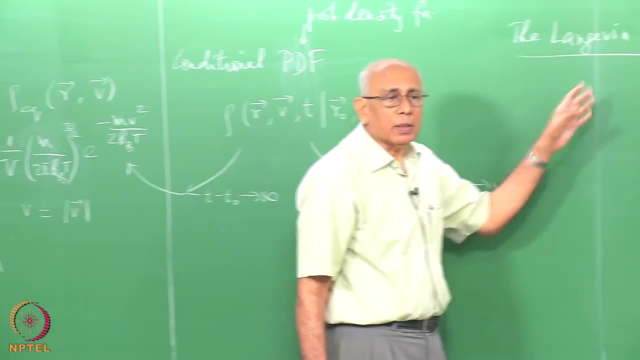 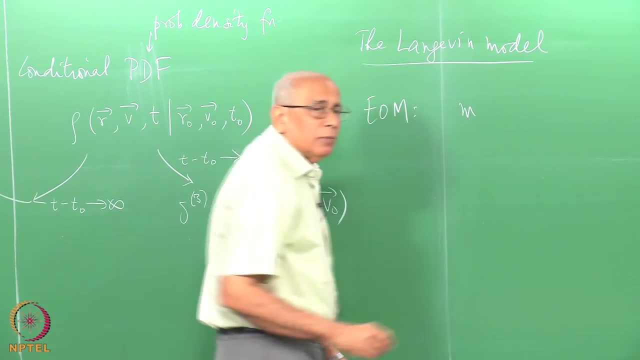 Now I ask this question here And for that purpose we are going to aim at that. but to start with, let's do the following. Let's start with an equation of motion for this particle. So what is its equation of motion? It says m, and for notational simplicity, for the moment we will put this in complication. 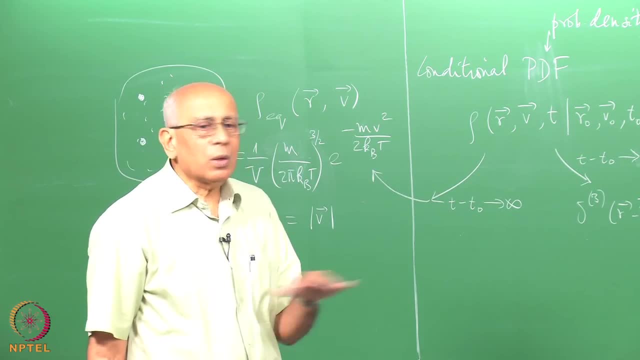 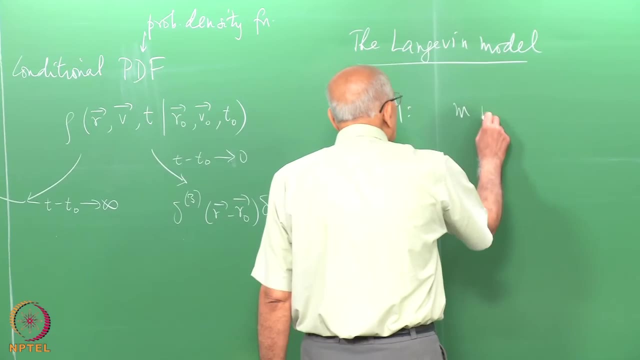 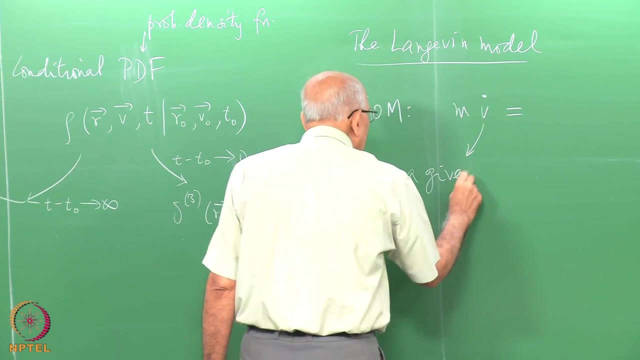 in a little later. For notational simplicity, let's look at one Cartesian component, of the velocity x component, for instance, And let me just use v. I need to simplify it. the notation m v dot. this is a given Cartesian component of v. 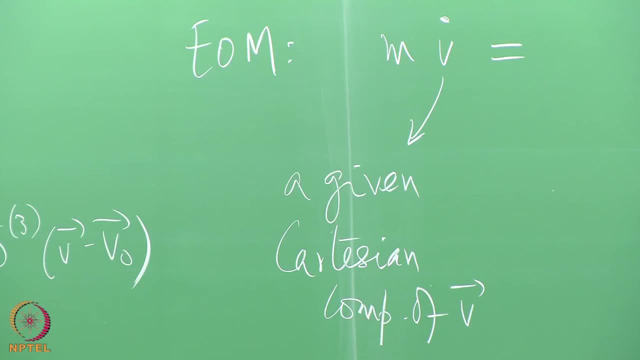 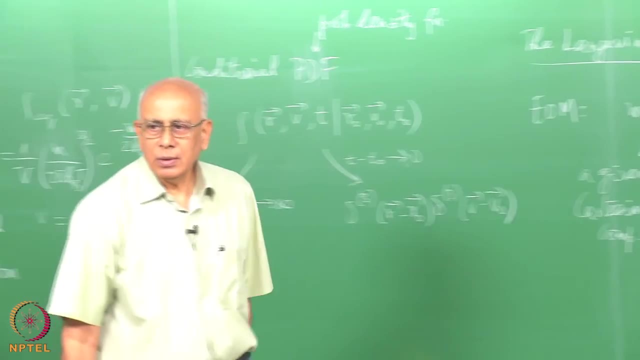 It's a little abuse of notation because I call v the magnitude. but forget about this now. I will just use this. I should have. otherwise I should write v 1,, v 2 or v 3, which is a nuisance to carry on. 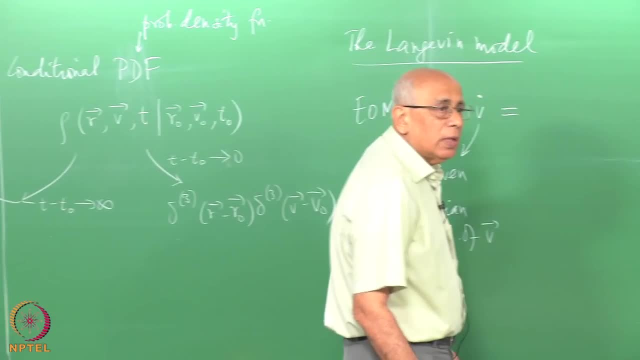 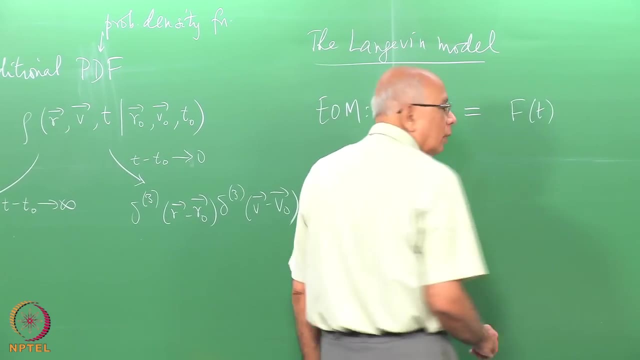 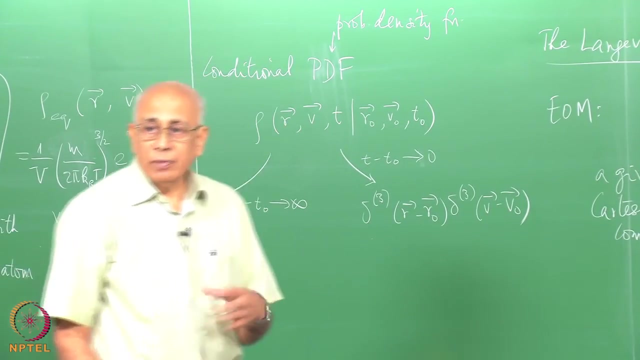 Ok, And what is this m v dot equal to? It's equal to the force on this particle, instantaneous force on this particle, Which is varying as a function of time, because the force is caused by the collisions of the molecules around and it is varying very rapidly, and 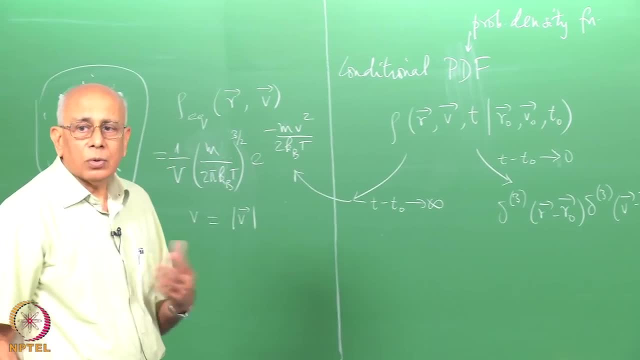 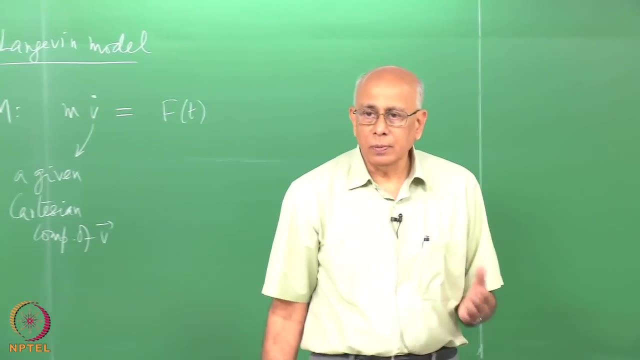 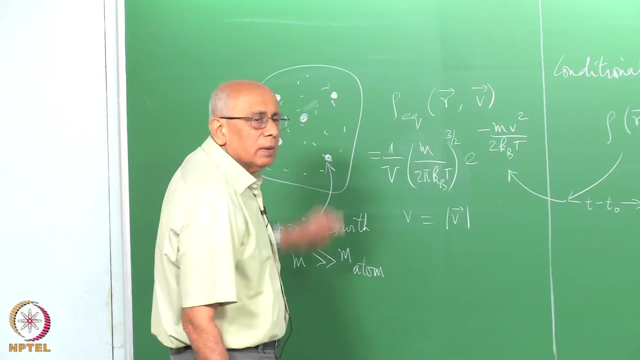 very randomly. In fact, in the in the gas in this room, for instance, on the average there are about 10 collisions per picosecond or so for the molecule. So it's really happening very, very fast and this is being buffeted by these particles very randomly in a fluctuating 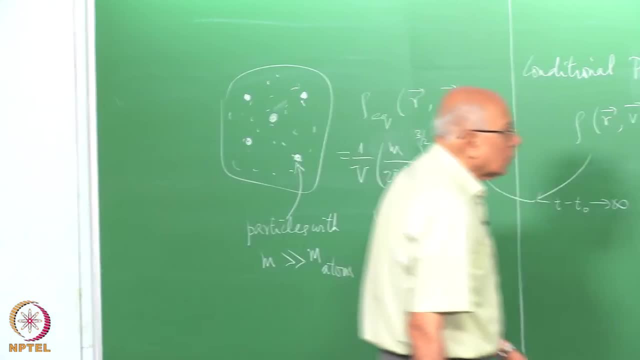 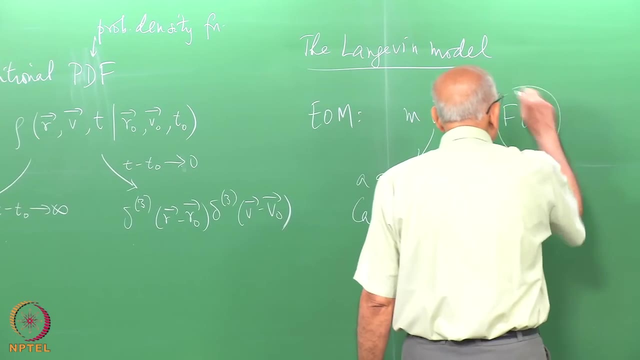 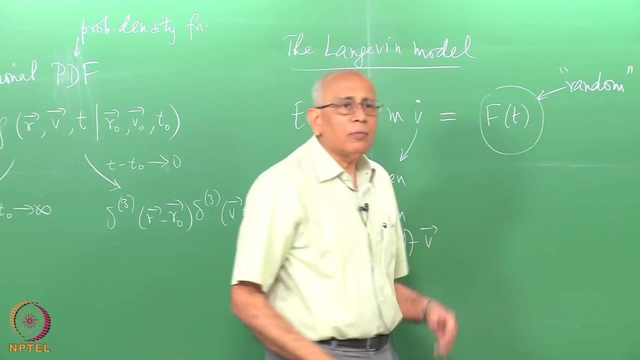 manner. So this is the total force and it is supposed to be random. This fellow is supposed to be random. It is random in the sense that it is random for all practical purposes, because if I were able to actually write the equation of motion down for all the particles in the 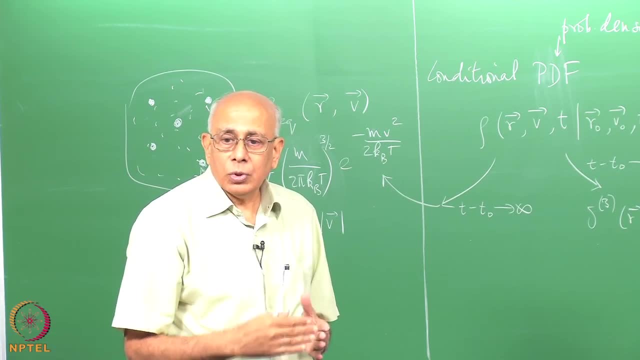 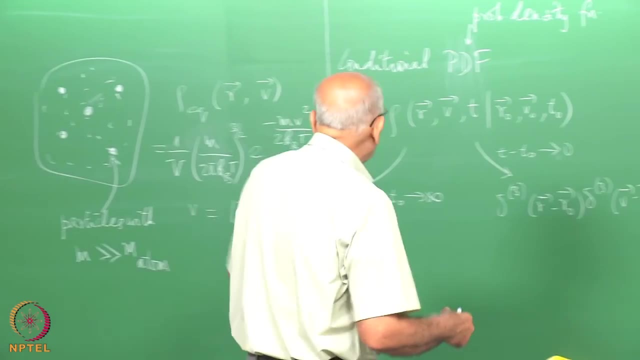 system, then of course I know where they are going, what they are going, who is going to hit which other particle and so on, and then there is nothing random about it in that sense. But of course, once you have a very large number of particles, for all practical purposes this: 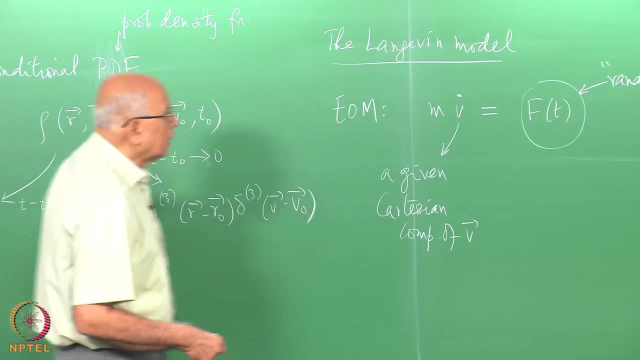 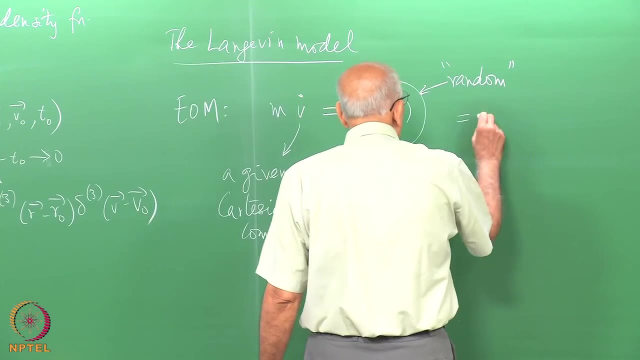 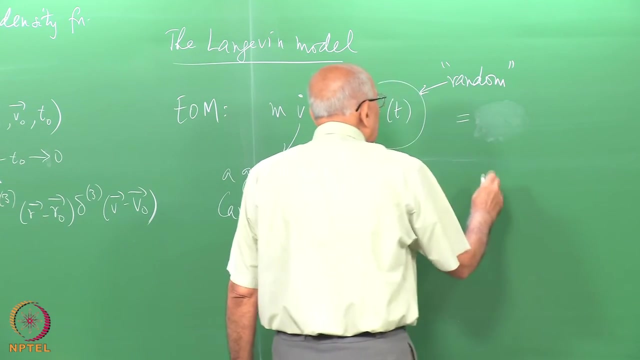 force is totally random here, right? I want to use a symbol for this random force, So let's write it as equal to some eta of t. I want to use proper notation, So let me write it as a quantity: gamma times eta of t, where. 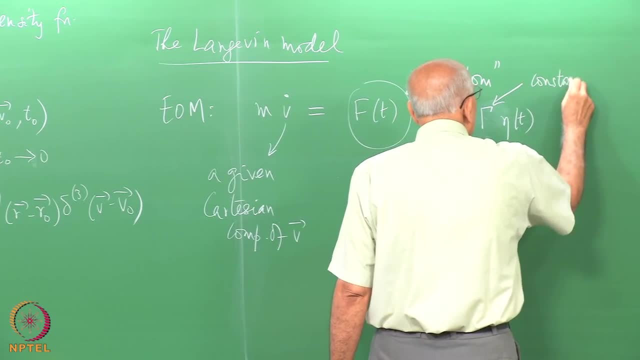 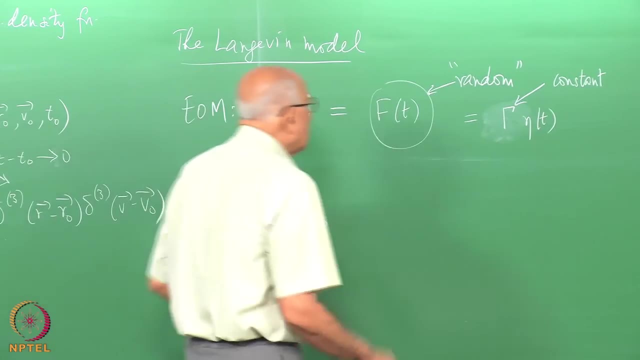 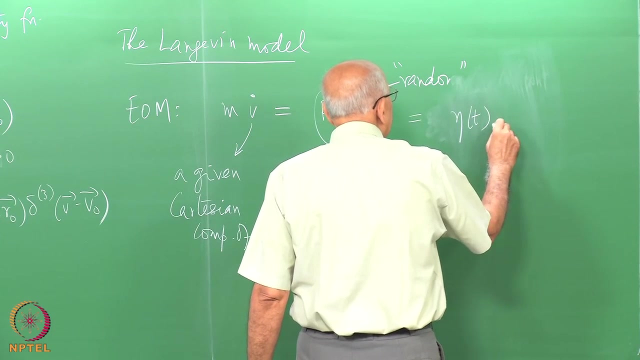 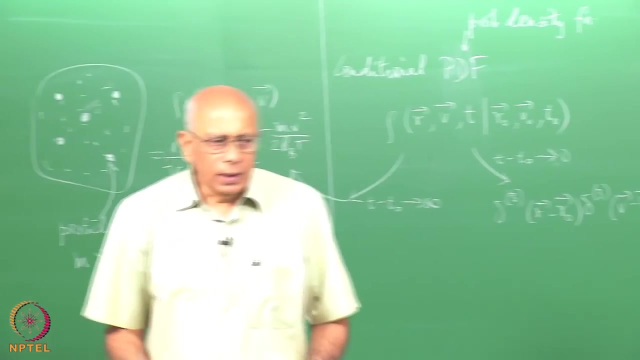 this is a constant. Well, I want to simplify this notation as much as possible, So let me just write it as eta of t, and we will come back to what this means. Okay, The randomness that I am going to put into it is to say that this eta of t is what? 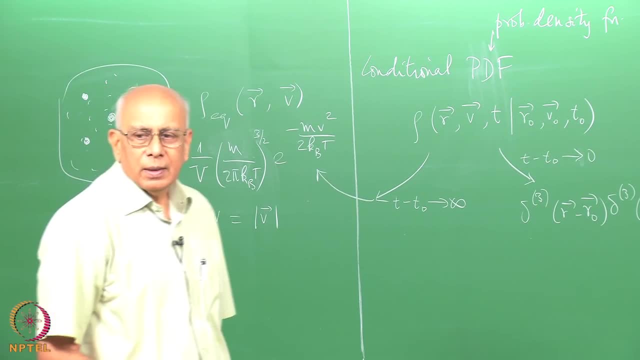 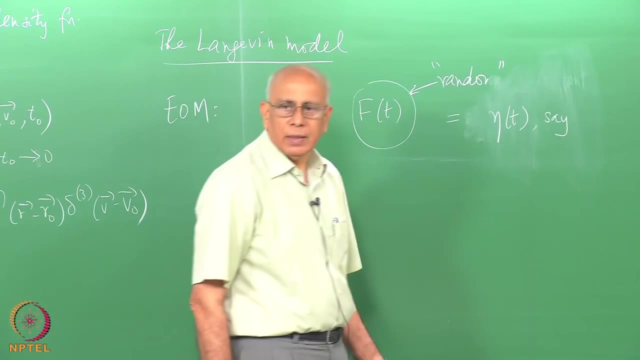 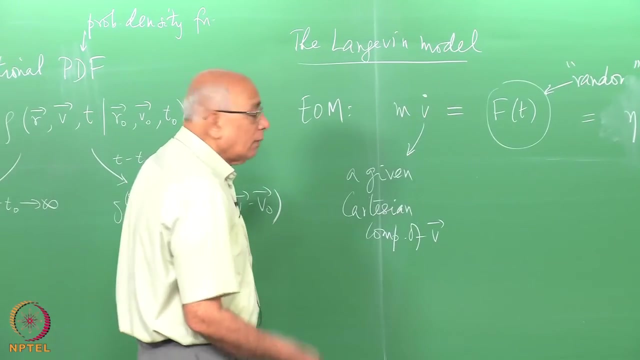 is technically called a Gaussian white noise. So I will explain these terms. what is meant by that? as we go along, but it is some random force of this kind. It has physical dimensions of force as it stands here. okay, So I have this simple equation and the matter is over. 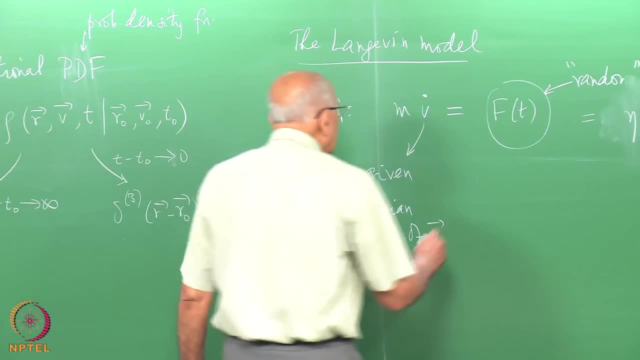 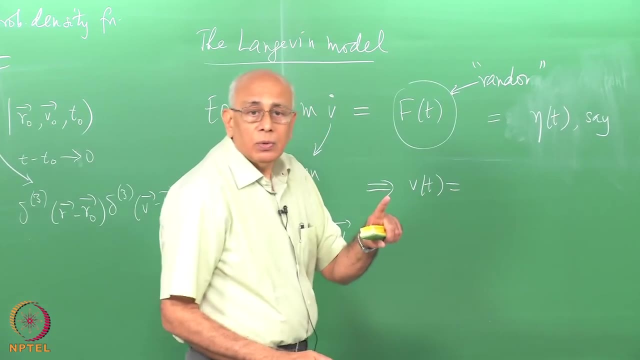 in the sense that I can integrate it formally. So once I integrate it, I have v of t equal to an initial value of the velocity, because I want to find out this quantity here. So I am going to start by saying: to solve a differential, 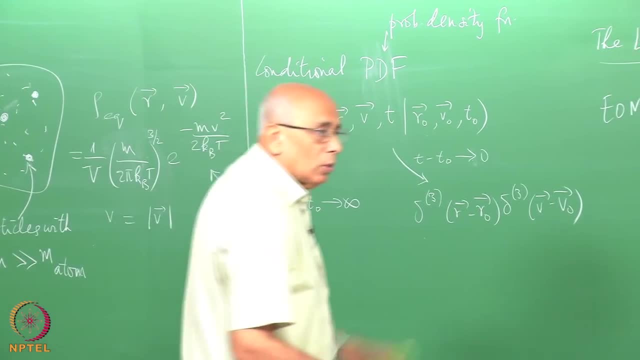 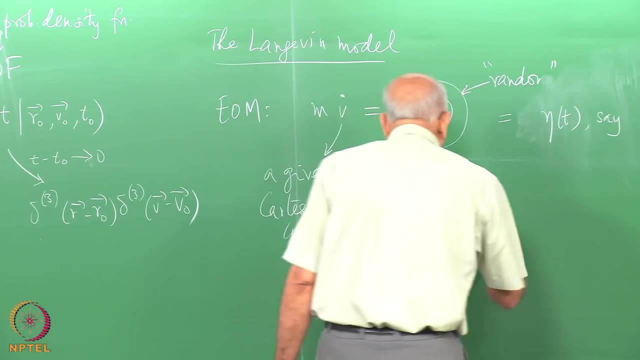 equation you need to specify an initial condition. So I am going to say: at t equal to 0, the value of the velocity was of this component, was some number, v naught, okay, So v of t equal to v naught, that's the initial value. 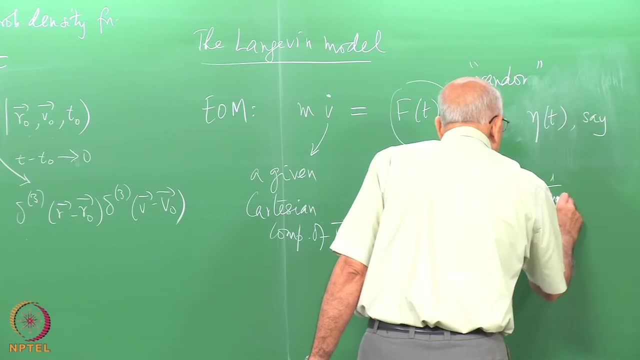 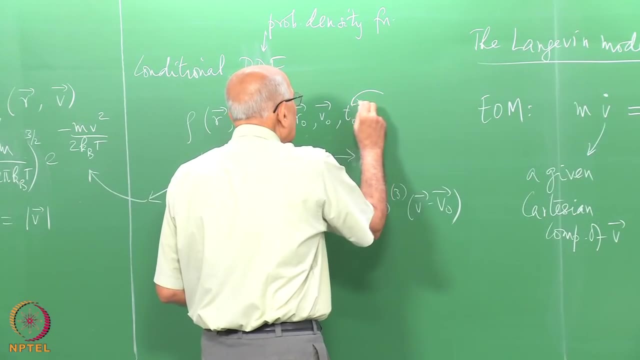 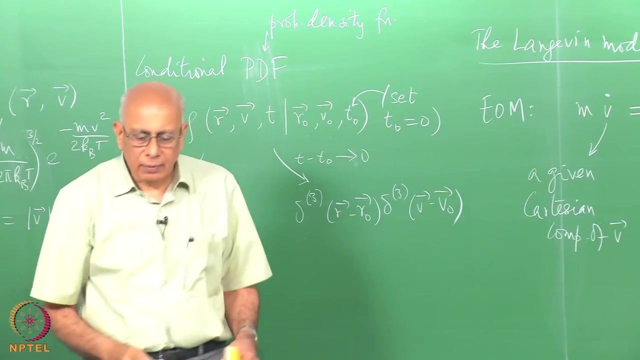 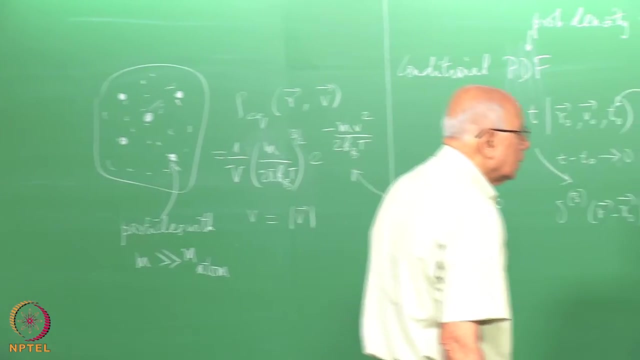 Okay, Plus 1 over m integral. I might as well choose the initial time. t naught to be equal to 0.. Set t naught equal to 0 because, as we have said, as I have argued, this whole thing is in equilibrium, So it doesn't matter when I start the clock. So this integral runs from. 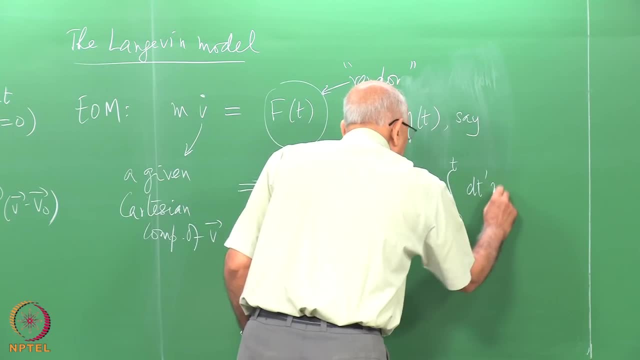 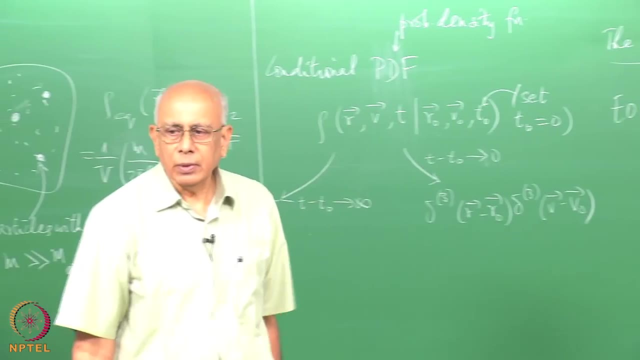 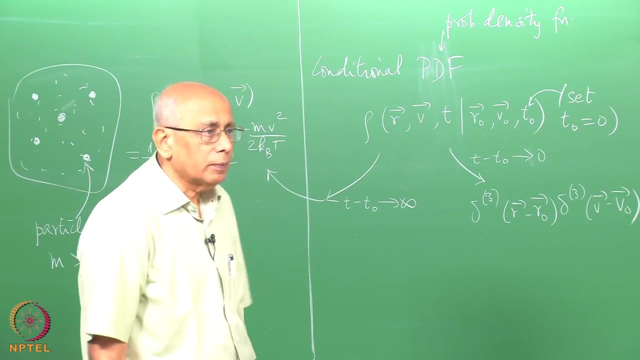 0 up to time, t dt prime. Okay, Okay, That's the formal solution to this first order differential equation, this triviality itself, and it satisfies the condition that at t equal to 0, v is v. naught here, But this is a random. 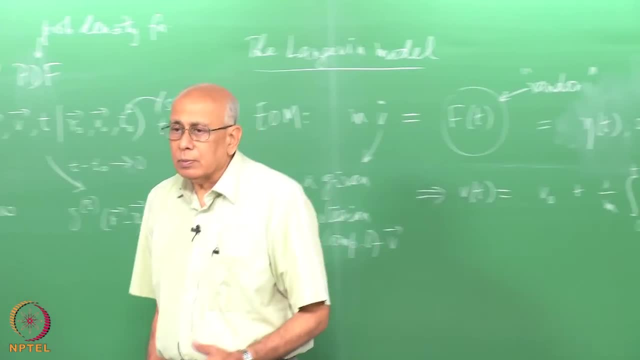 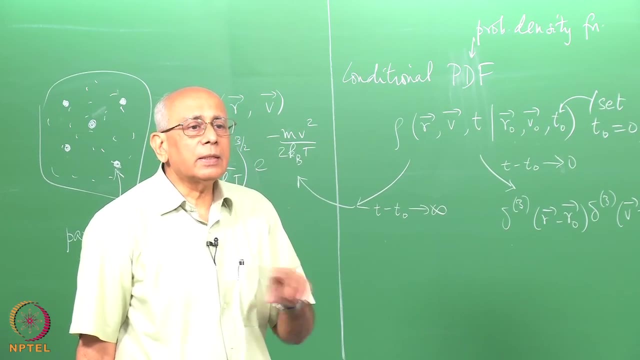 force, and what I want is averages, because once I have a random variable, what I am interested in are its averages of various kinds, averaged over all realizations of this force, So all the force histories that are possible, and each time there is a different history. you. 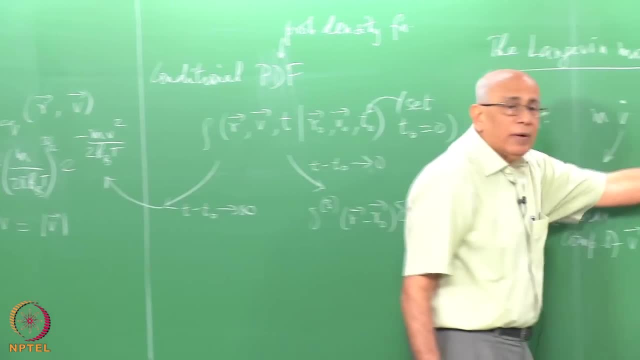 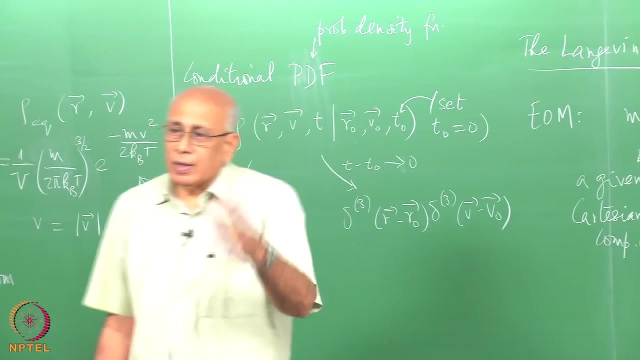 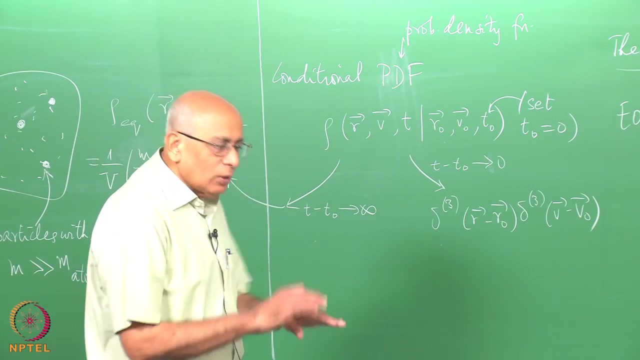 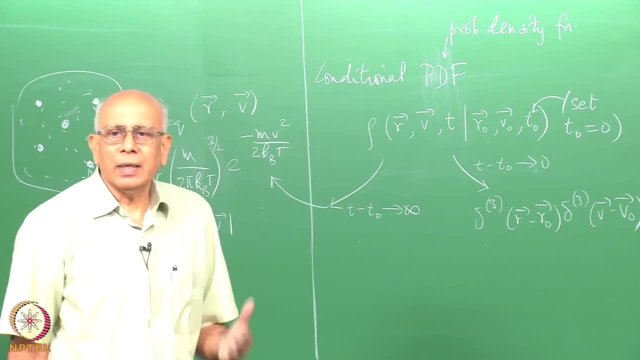 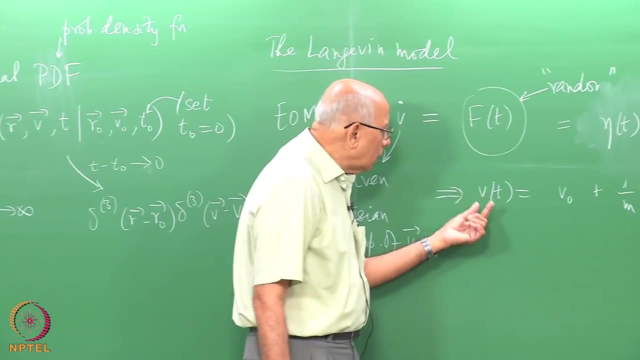 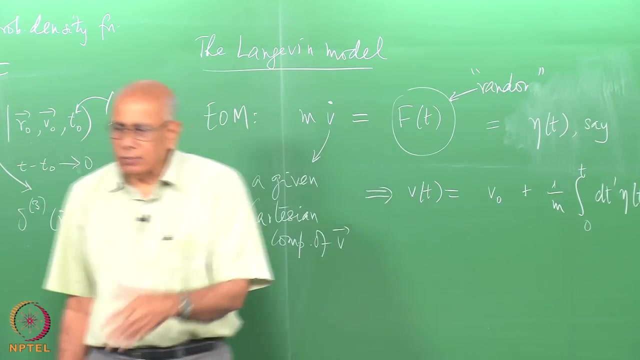 I mean? What do I mean by averaging over realizations of the noise? What, what? what is the input variable here? Well, we will do this averaging in two steps. When I want any quantity which is an average, of referring to this particle's dynamic variables, such as its velocity or 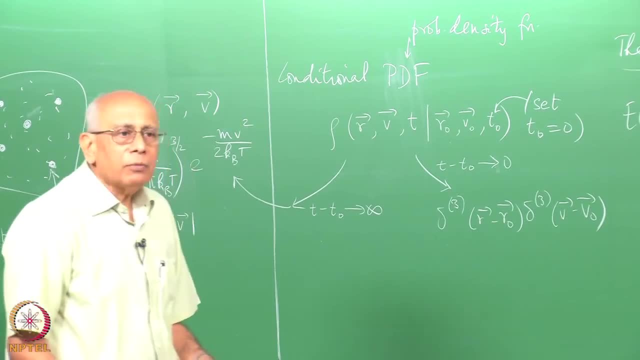 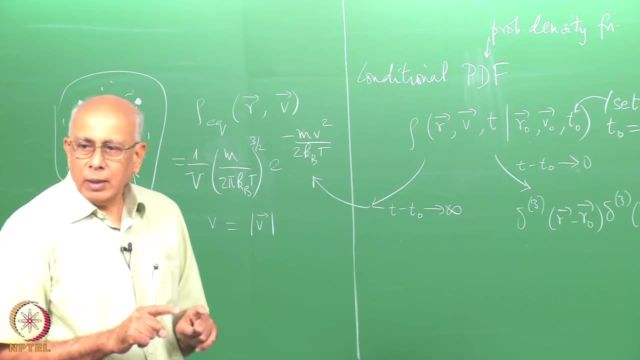 its mean square velocity, and so on. I have to tell you, what am I averaging over? Not only should I average over all realizations of this noise, but I should also average over over all possible initial conditions, because there is no reason why I should have chosen. 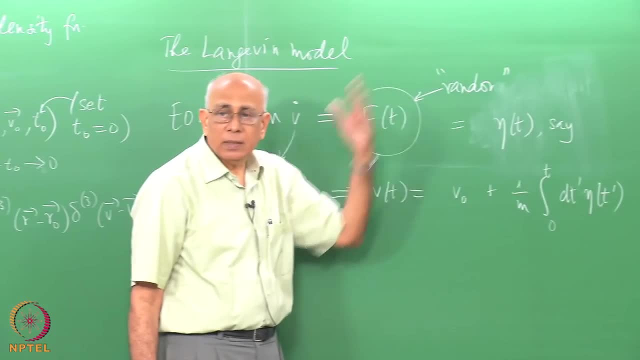 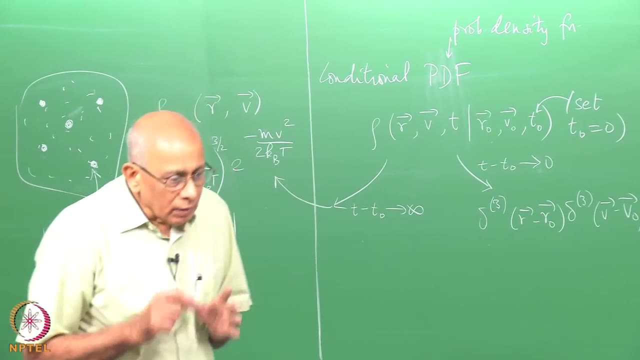 v naught as the initial value. I could have chosen something else as the initial value. So there is a double average involved here. First an average over a for a given v naught. you average over all realizations of the noise for a given initial condition, and then you. 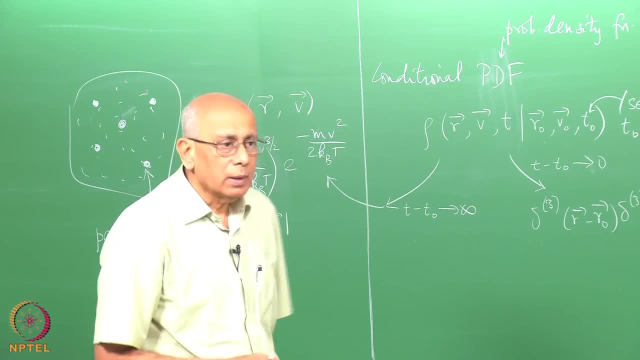 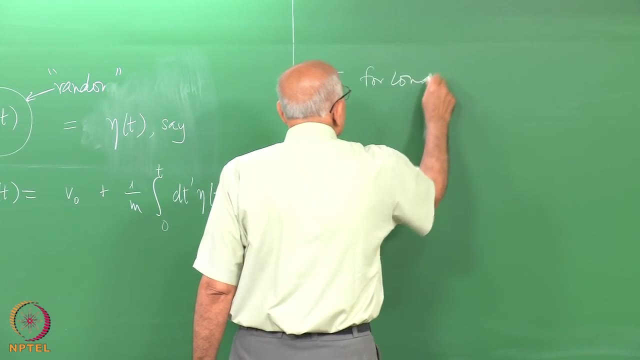 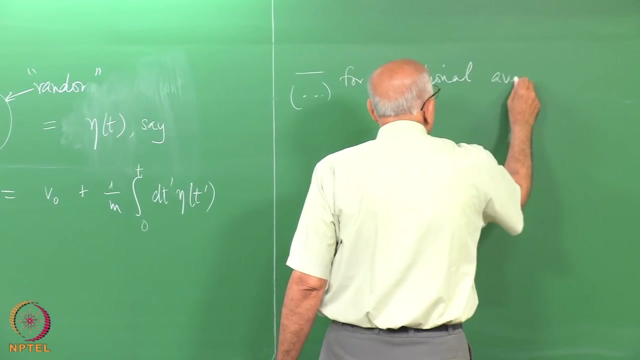 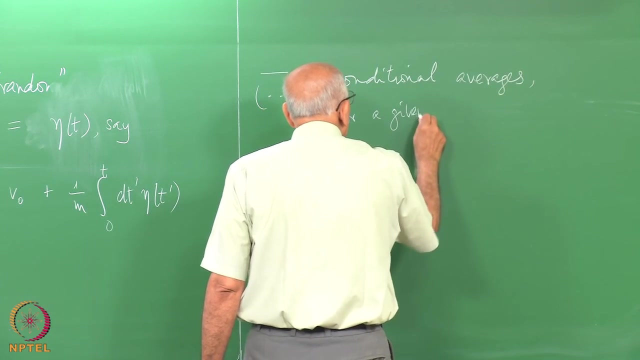 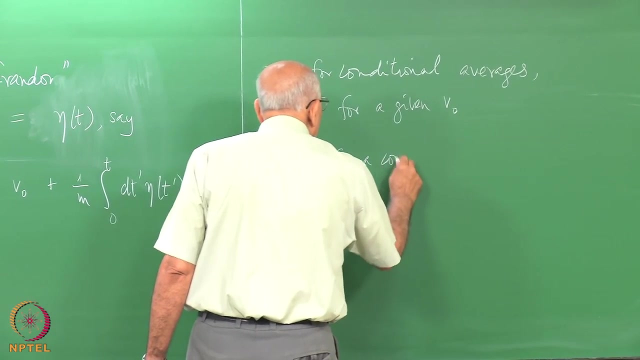 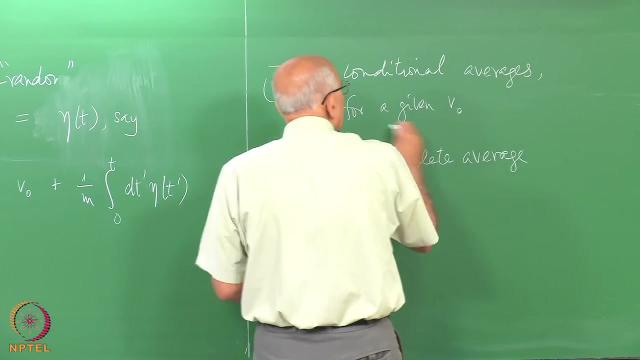 average over all possible initial conditions as well. So I am going to use overhead bar for conditional averages- Whatever is inside here- for conditional averages for a given v naught, And I am going to use this for a complete average For a given v naught. 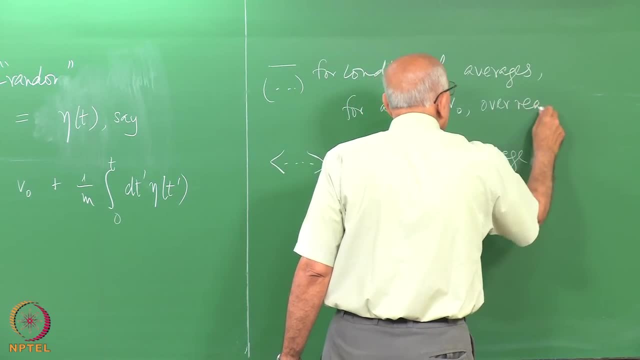 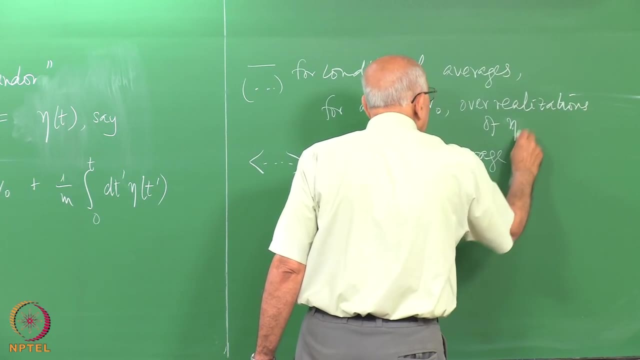 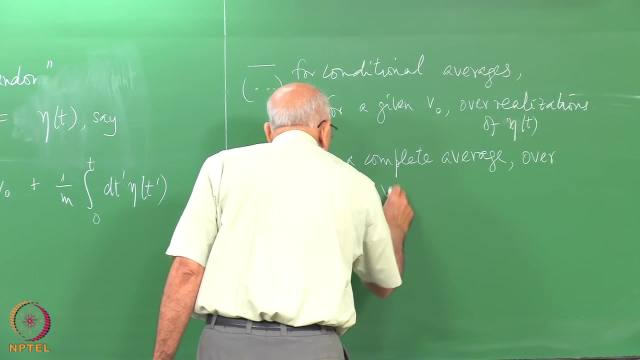 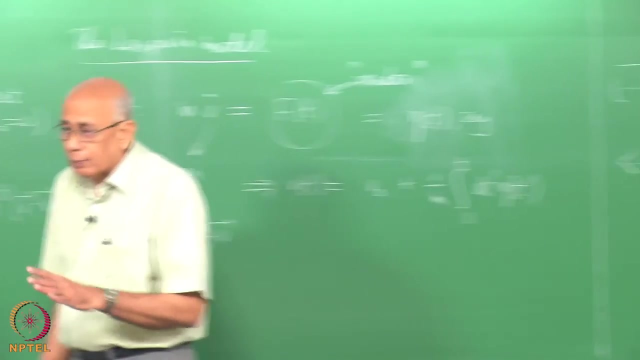 Over realizations of eta of t complete average over all v naught as well. Ok, So we will do this average in 2 steps. First we average over start with a given v naught. So we look at the ensemble. 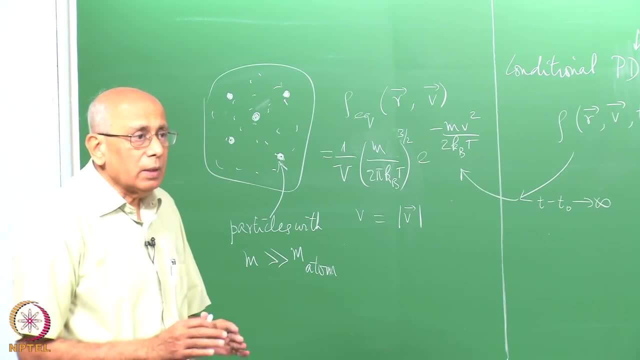 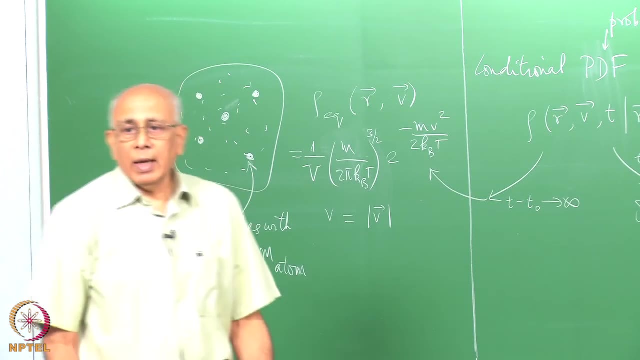 The ensemble of these particles, such that the v naught is given, and we repeat this experiment with different eta of t each time. Take the average, and after that we will average over the initial velocity as well. Ok, Now, implicit in this is the fact that these averages should: 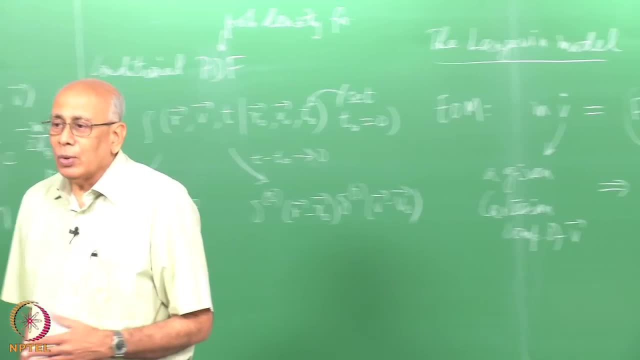 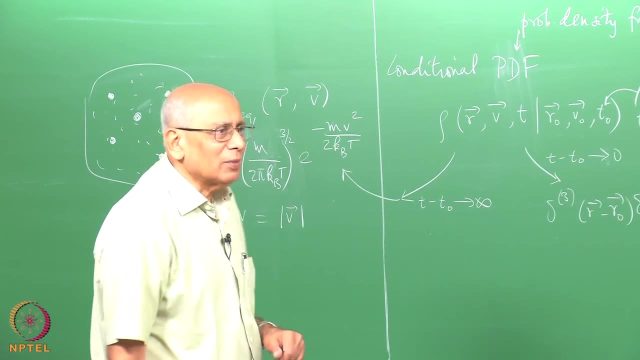 commute with each other. Whichever order I do it in, I should get the same final answer, And that's more or less obvious, with a little subtle assumptions involved here. First of all, averaging is an arithmetic. It is an arithmetic. It is an arithmetic, It is not. 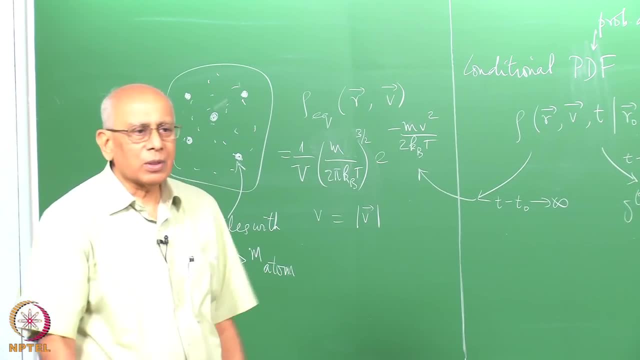 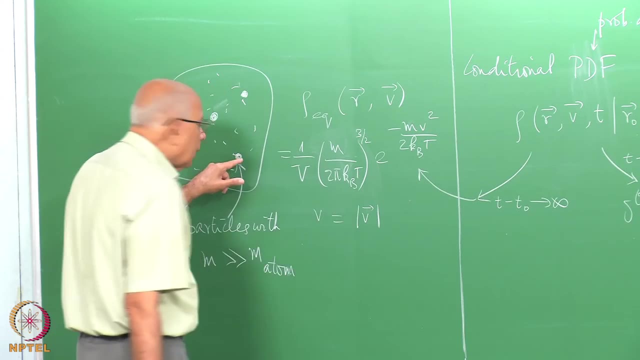 arithmetic, averaging, It is just adding numbers, And addition is always commutative. But more than that. there is a deep assumption here that whatever is the fate of this particle doesn't affect the bath, the heat bath. So the assumption is the heat path's properties. 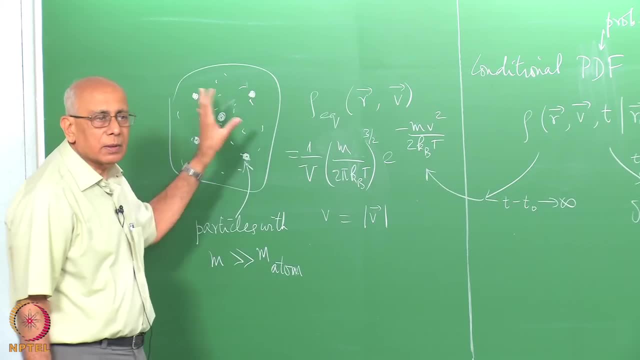 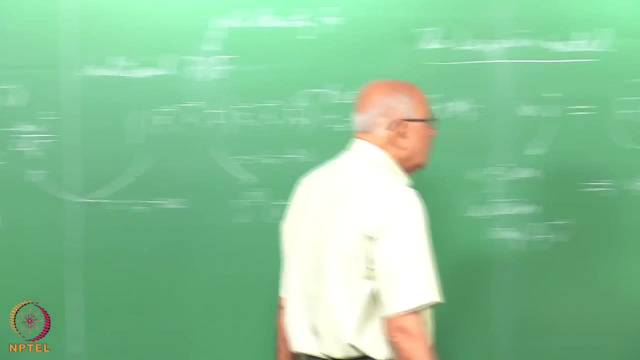 do not change as a consequence of the motion of these particles. That system remains in thermal equilibrium at temperature t. Ok, So this noise it's. let us take a look at this. The electrical properties are not affected by what an individual Brownian particle is. 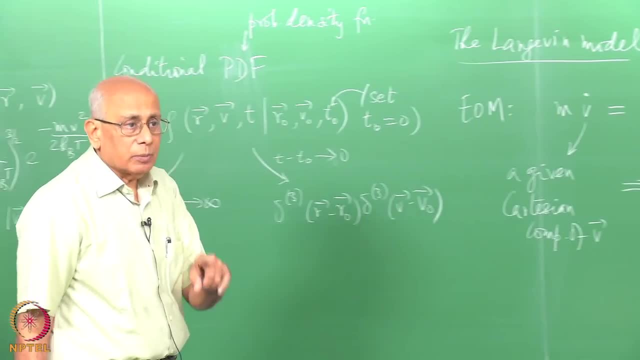 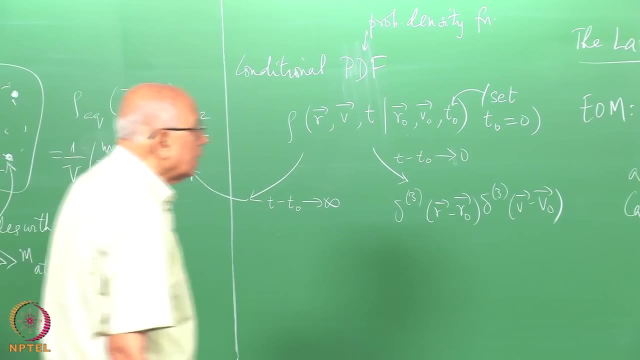 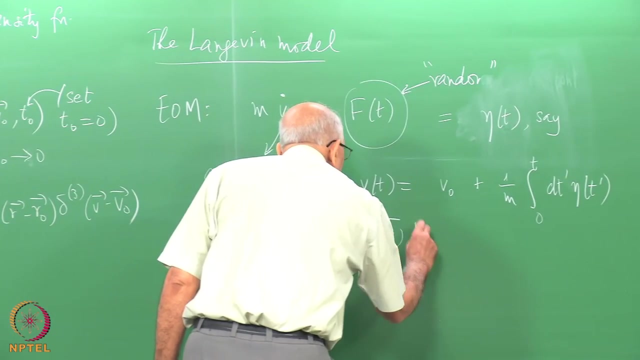 doing. Ok, So that's a physical assumption, And you have to make sure that that's really satisfied before this model becomes realistic. So, given that, let's take the average over this. No, So what is v of t equal to? There's nothing to average here, because this bar is. 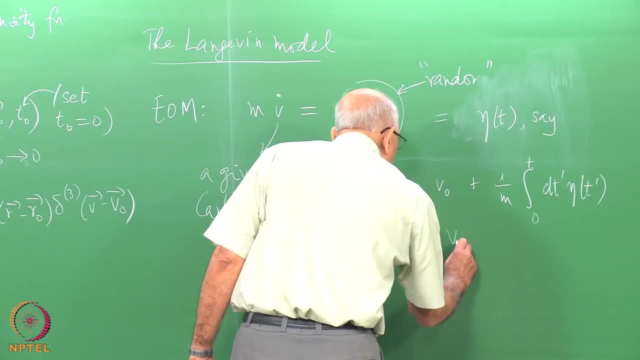 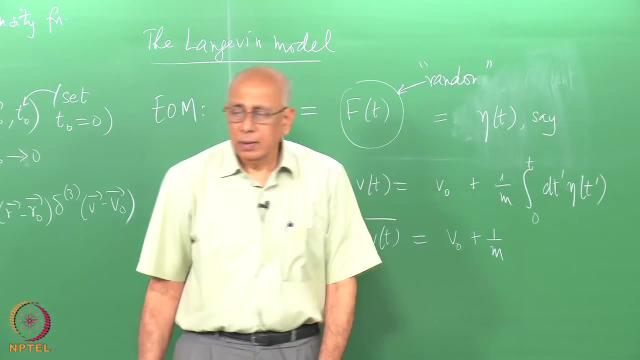 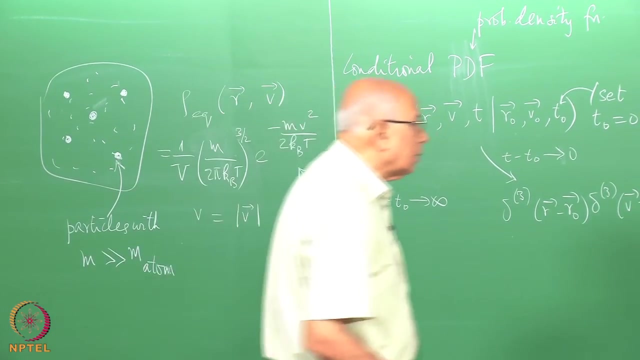 for a given v naught. So this is a deterministic number and you get just a v naught, So you v naught plus 1 over m, the average of this integral. Ok, But an integration is a summation and the average is also an additive operation, right arithmetic average. So this is equal. 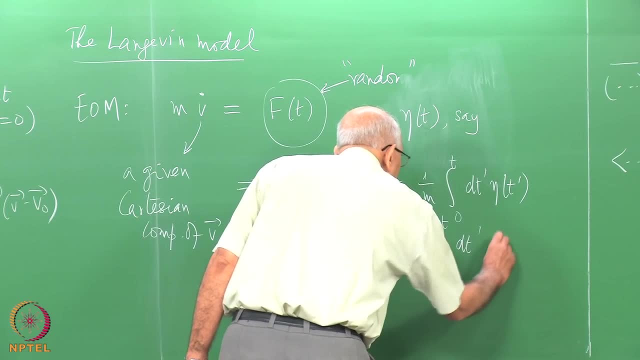 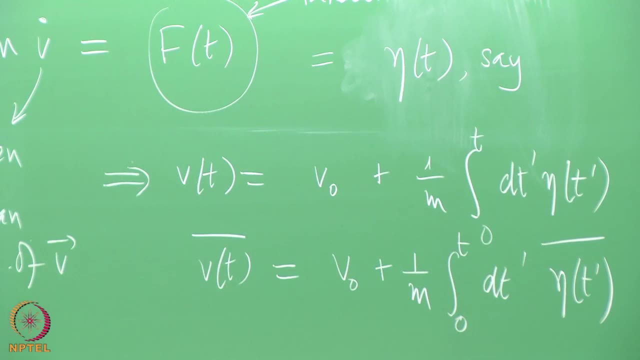 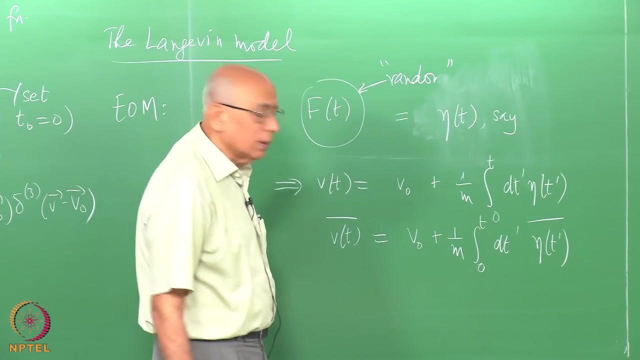 to integral 0 to t d, t prime, eta of t prime. So notice how carefully we are proceeding step by step, so we know what the assumptions are at every stage. So every one of these operations has to be justified. Ok, So you agree that this is indeed the average value? 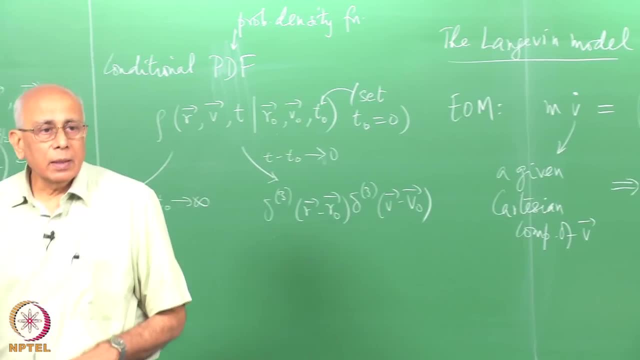 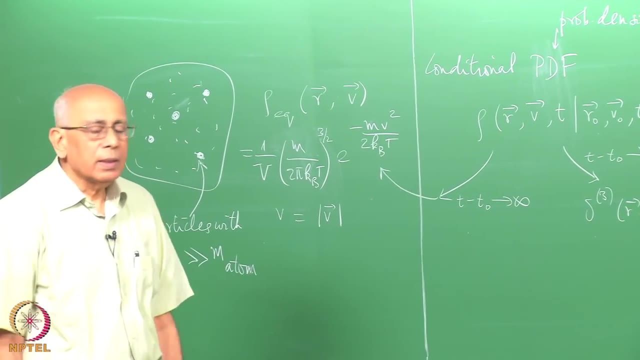 of the velocity. but now I argue, saying that this particle is not going anywhere. It is staying inside the container and it is hit as much from the front as from the back and the average value of this force, it's very reasonable to assume, is 0.. The average force: 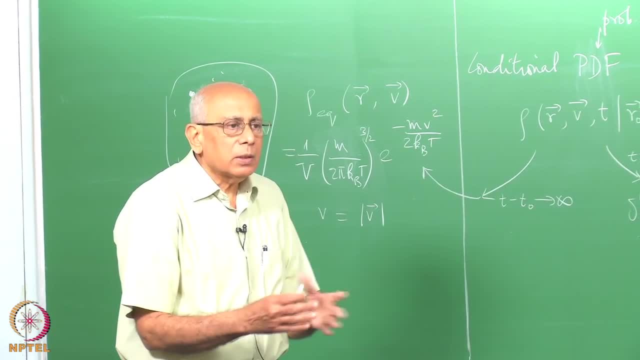 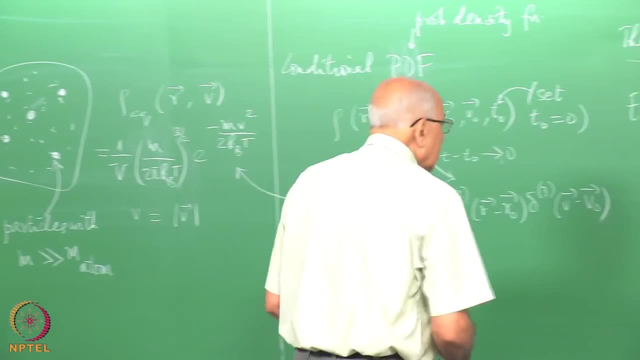 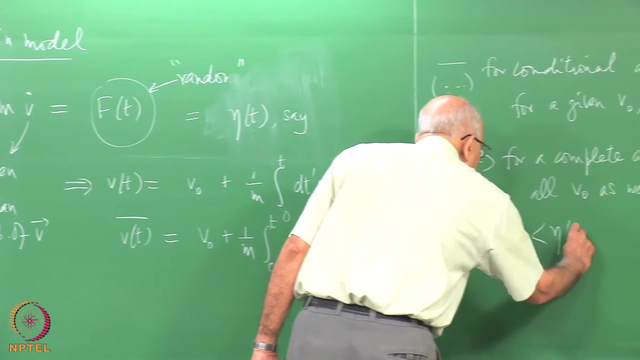 exerted on this Brownian particle by all the other particles is, on the average, zero, because its average velocity is in fact zero. Ok, So we will make the assumption that eta of t average, which indeed is equal to eta of t as well, because even if you change all the 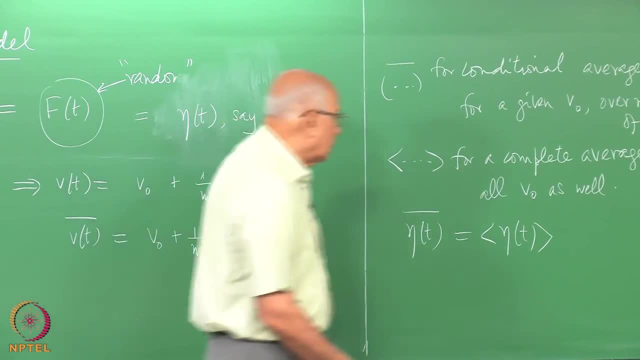 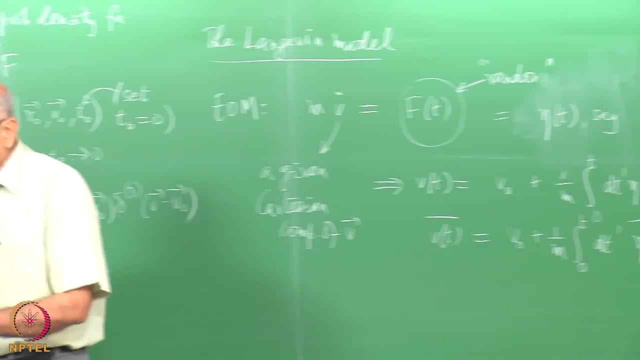 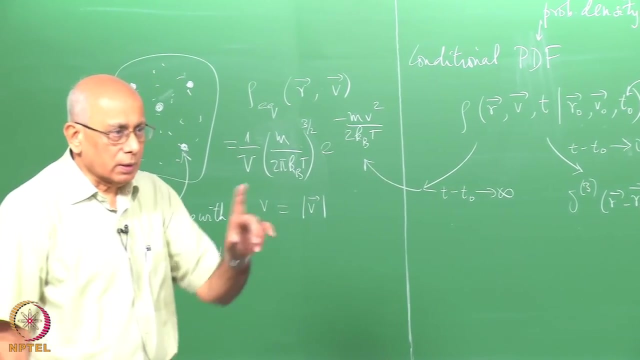 initial conditions, it is still true. This is equal to zero. So, as far as the properties of eta are concerned, it doesn't care what the Brownian particles are doing, and its average value is zero. That's the first thing that it's a noise with zero. 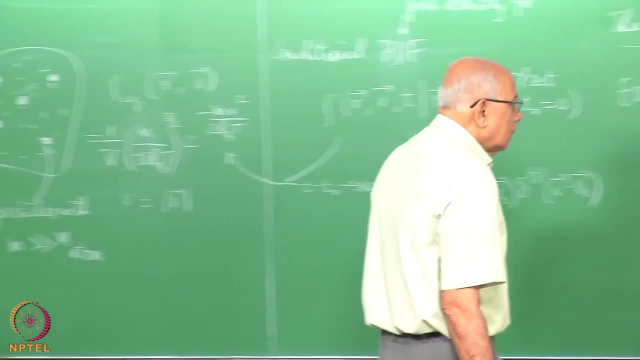 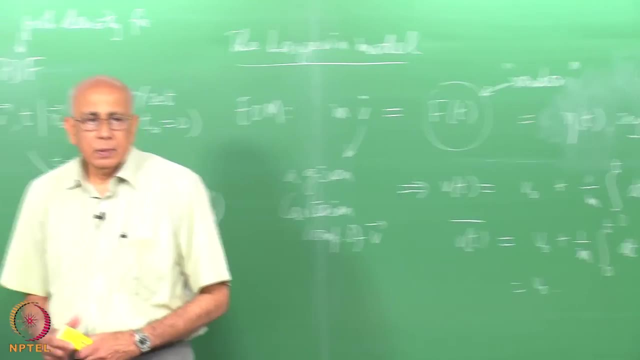 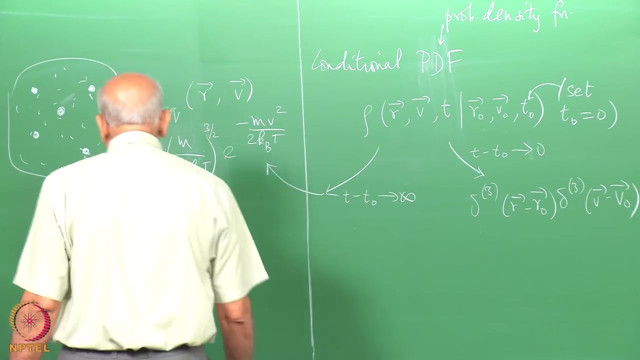 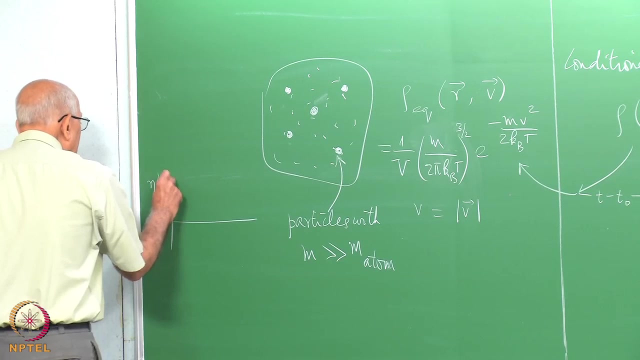 mean Ok, So this term vanishes and this is equal to v naught, Yeah, No, no, no. Realization is: if I plot this eta of t, If I plot this eta of t, which is the x component of the force, if I plot this eta of t versus. 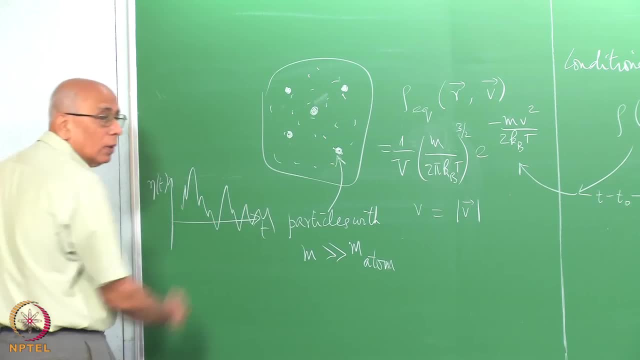 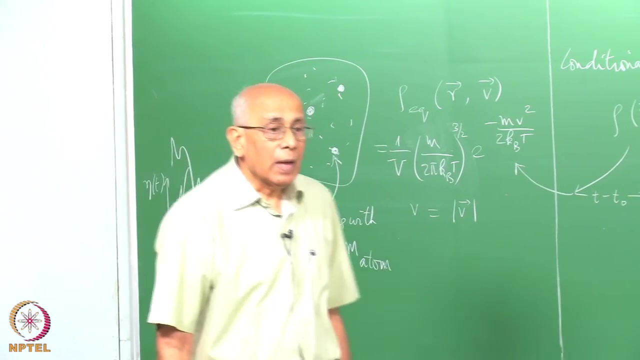 t. this might be one realization of the noise, But it could equally well have been this. It could have been this. So I am going to average over all these realizations. Pardon me: Average. average on the average, Because if it were not zero, this particle would move. 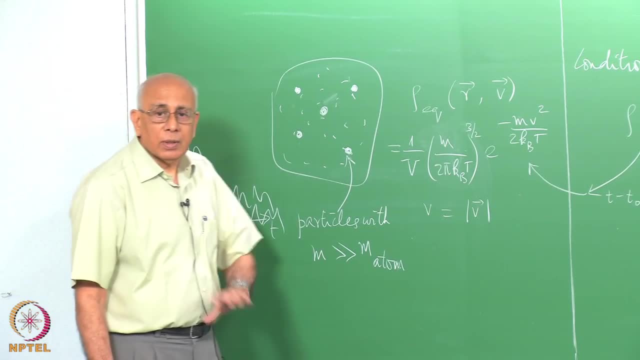 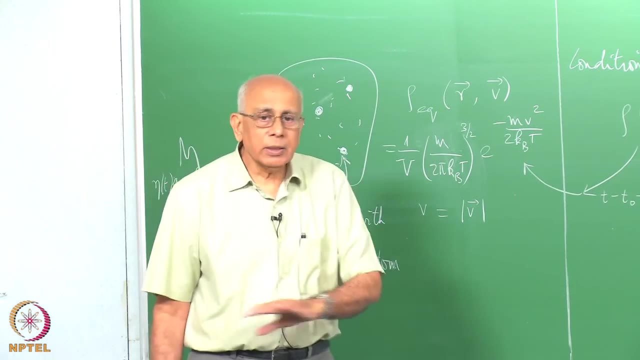 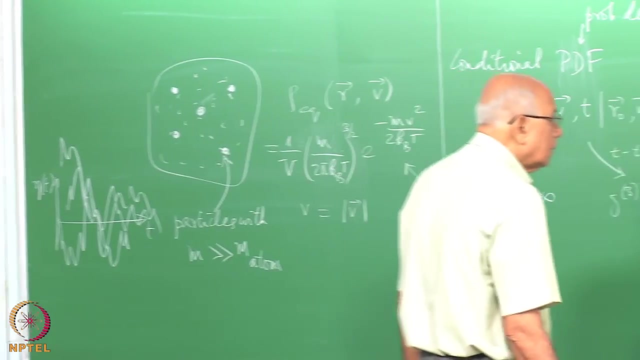 vertically in some direction. So it's clear, on the average it is zero. This, these are not. these fellows are not going anywhere. They will have a fluctuation about their mean position, but the mean itself is zero. to start with, Ok, We've already said that these Brownian 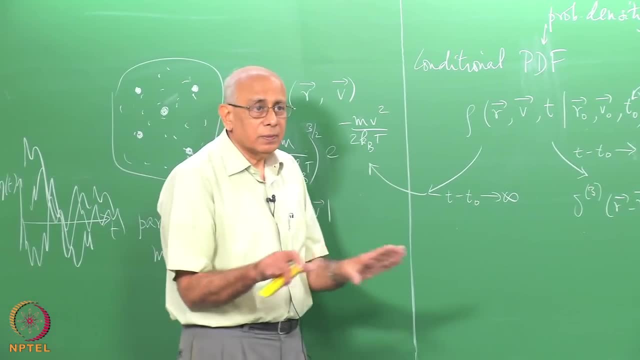 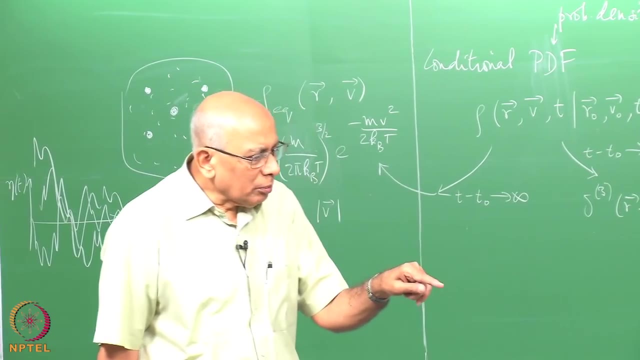 particles are in thermal equilibrium and the mean value is zero. completely. We're not going out of thermal equilibrium. We're just saying I focus on a particular particle and look at its initial condition and ask for conditional. 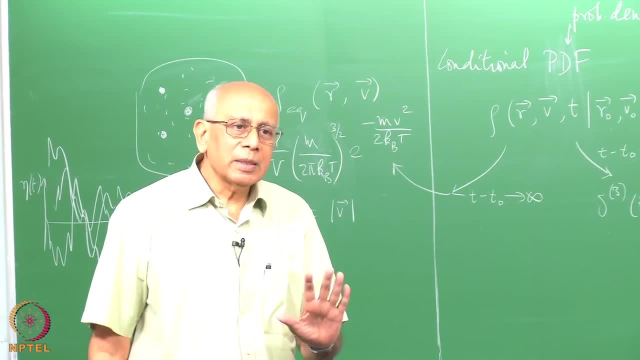 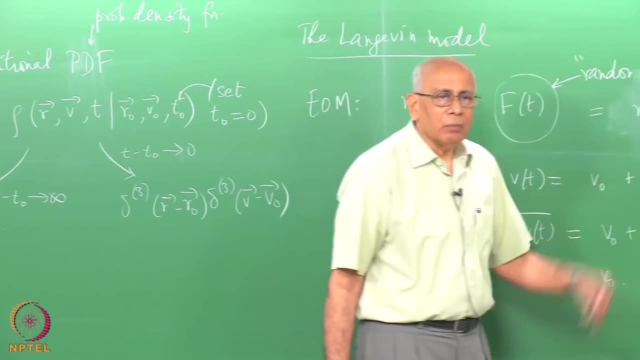 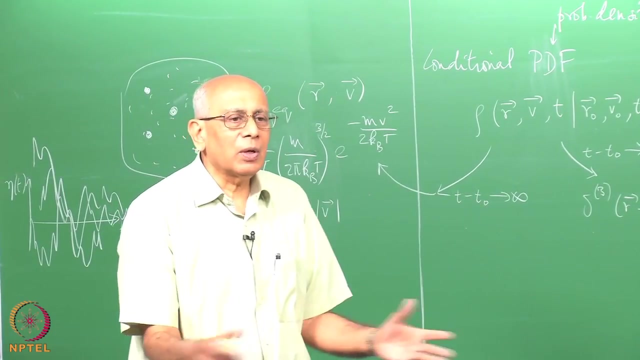 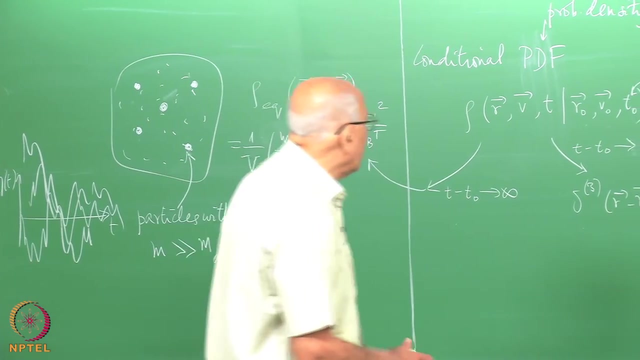 averages, subject to the condition that the system is still in thermal equilibrium, right. So we are asking a time-dependent question because we chose an initial condition that breaks the the fact that this velocity is zero on the average. It starts with some v naught and I ask: what is it doing? Or to put it yet another way: in pictures you can see: 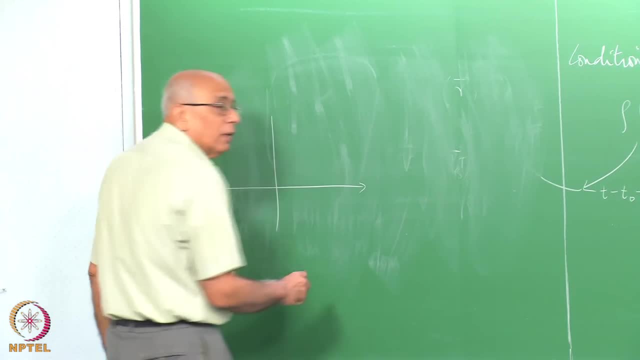 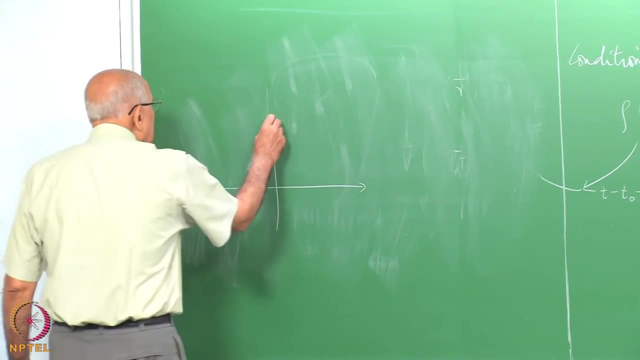 it's doing. let's do that. If I plot the velocity distribution- because the position is irrelevant here- that remains uniformly distributed throughout. but if I look at this rho of v, t given, v naught, this is the quantity I really want for this tag particle, And I plot v here, Then at t equal. 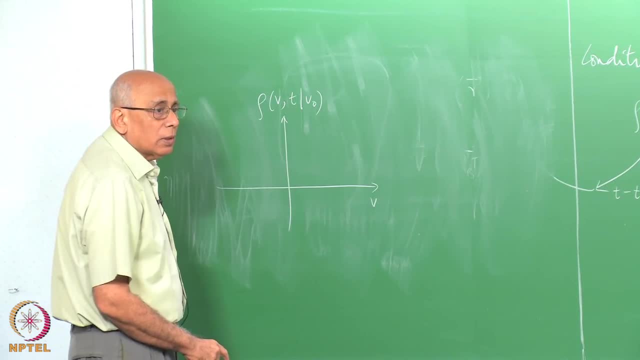 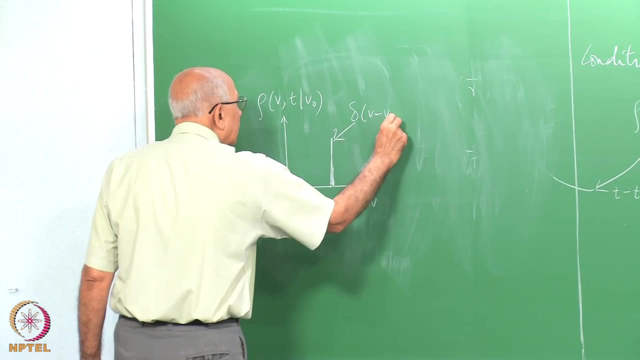 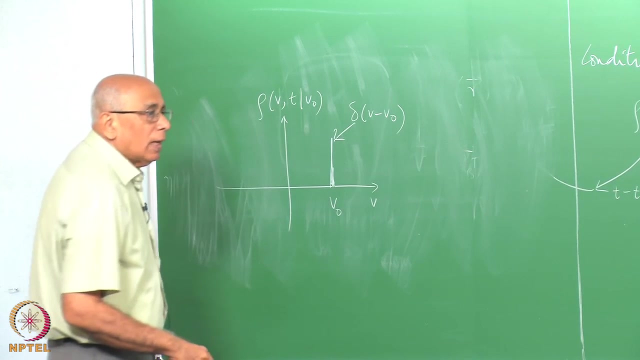 to zero, it is starting with a delta function at v naught. So it's clear that this is the distribution. where this is v naught, It is starting with a normalized delta function. as the distribution And as t becomes infinite, the value of this distribution here becomes. 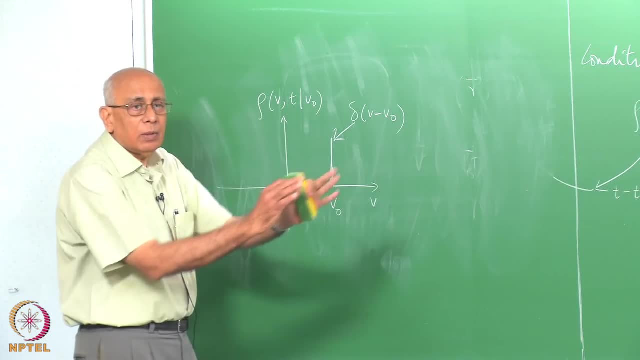 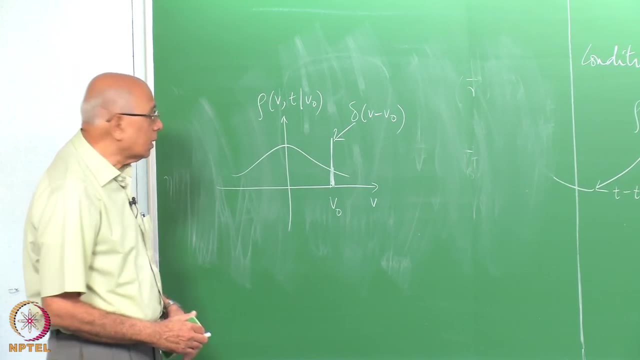 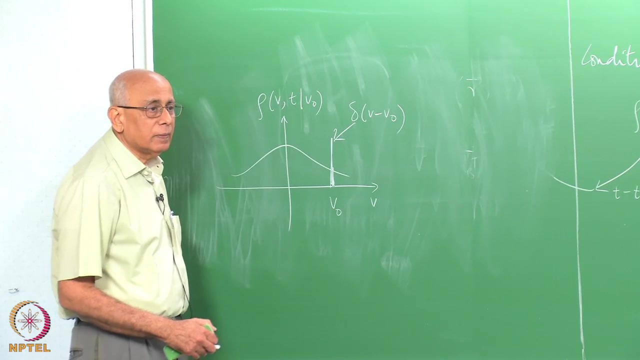 independent of the initial condition. It loses memory and it gets into the Maxwellian distribution. So it's finally like this, And the question we are asking is: how does a distribution manage to start with a delta function there and end up with a Maxwellian here, as t goes to infinity? 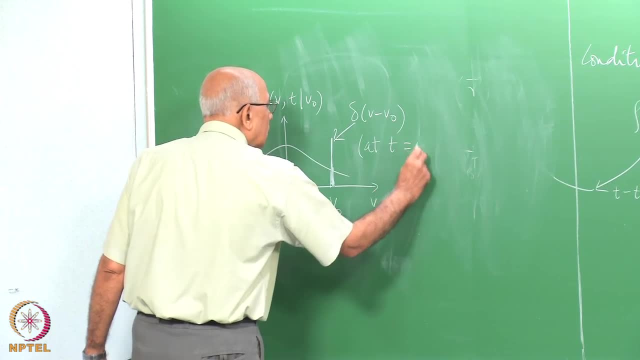 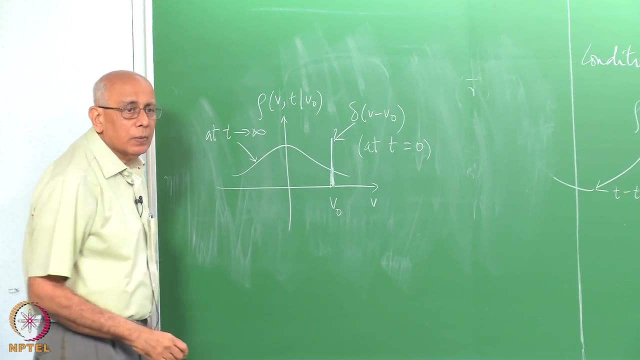 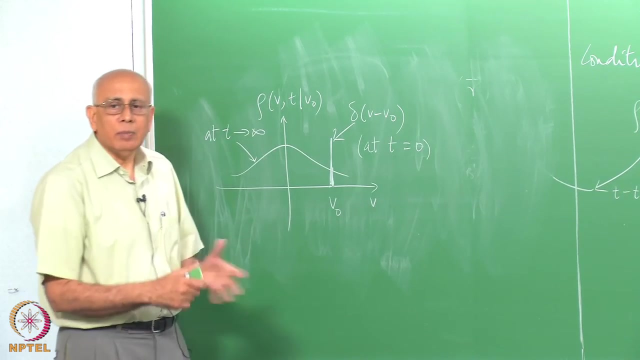 So this is the distribution. This is at t, equal to 0, and this is at t, turning to infinity. So that's the question we are really trying to answer: How does this distribution do this? What does it do In between? Not very surprisingly, you will discover that this mean value starts drifting. 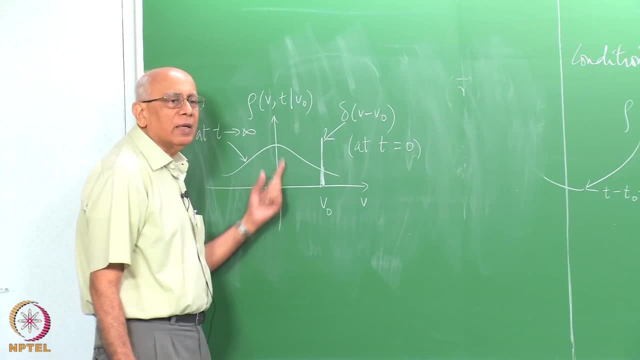 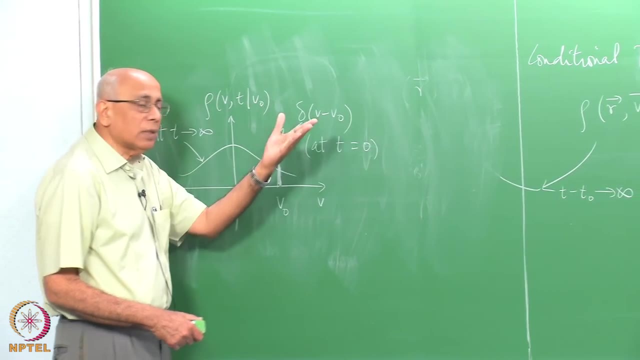 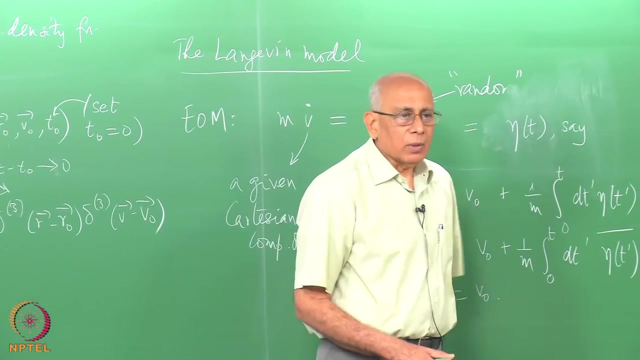 to the left until at infinity. it becomes 0 here, But in the meantime it's also broadening, because this has zero width and this has a width dependent on the temperature: k, t over m, square root of. So that's the kind of question we are trying to answer, But we are doing. 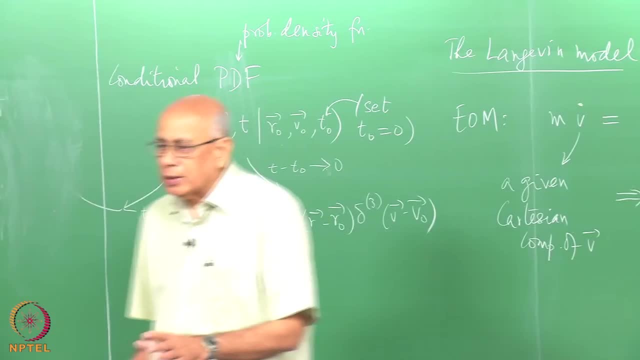 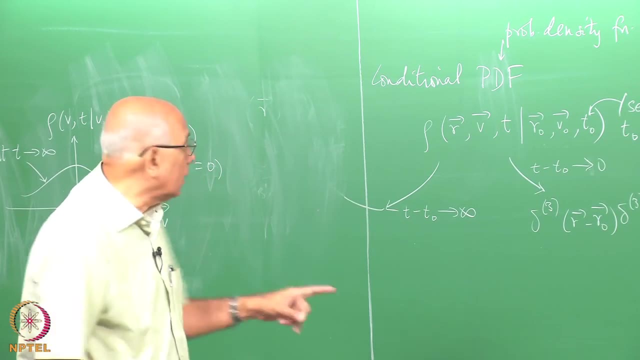 it through the equation of motion. So we will first get information on the mean, the mean square, the correlation, The correlation function and so on And then work backwards using that information to try to get a functional form for this quantity here And perhaps even write an equation down. 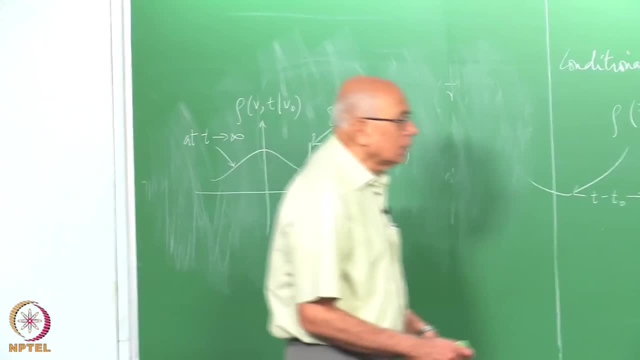 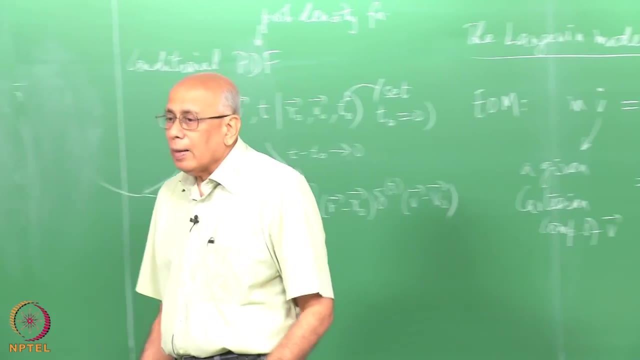 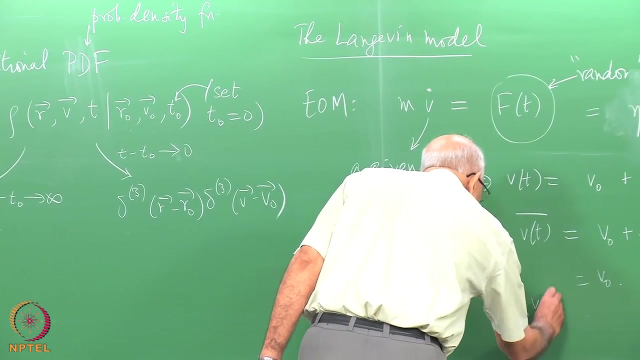 for it and maybe even solve it. So this was the first step here, And now the next thing to do is to ask what happens if I average over initial conditions as well. So we can do that right away. v of t, v of t. 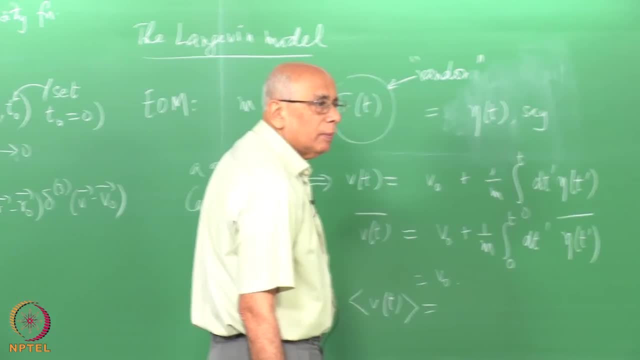 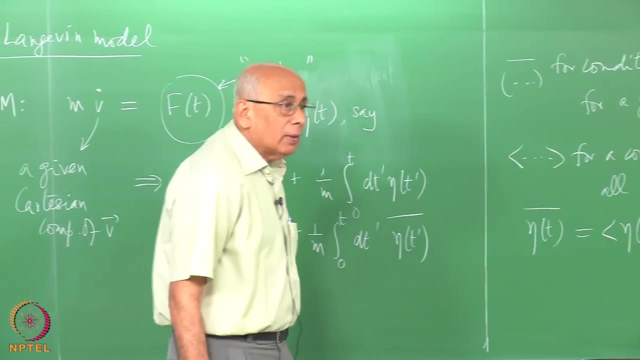 v of t. Yes, But the problem is, you would have wanted v naught to be 0,. right, Pardon me, The average should go to 0 eventually. right, Yeah, This is not working. No, no, it will. it will work. You will see This. this will work, Because now I am going. 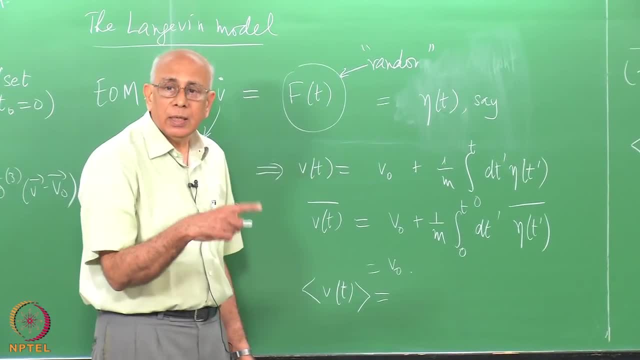 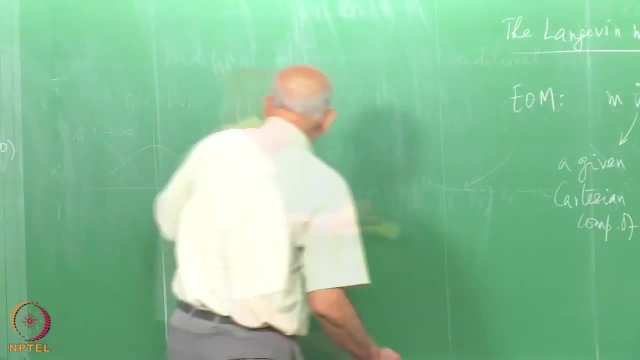 to ask what is the average value if I now average over all initial conditions? But remember, this particle was in equilibrium. So we know the following is true: We know that rho equilibrium of v, the equilibrium decimal, is 0.. Yes, So that is an equation. 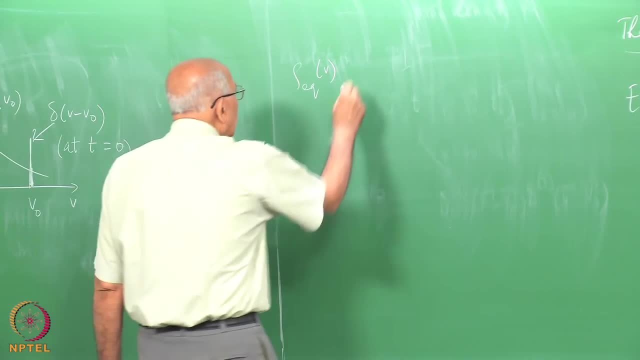 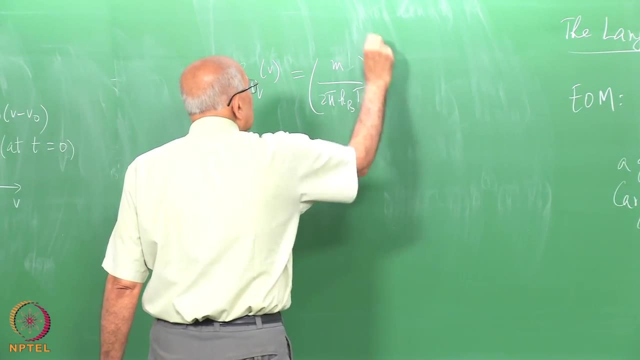 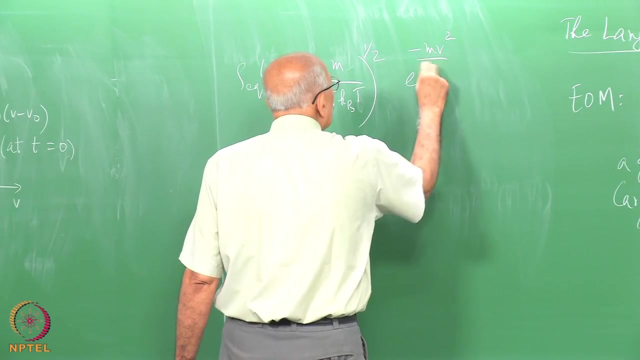 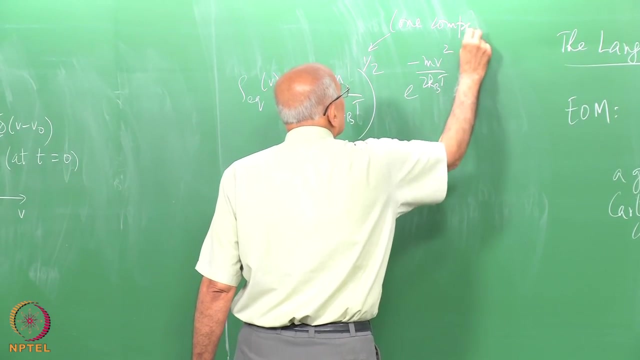 0.. distribution is the Maxwellian distribution. So we know that this is equal to m over 2 pi k Boltzmann t to the power of half. This is one dimension, one component only. so it is just a power half e to the minus m v square over 2 k Boltzmann t. One component v is denotes: 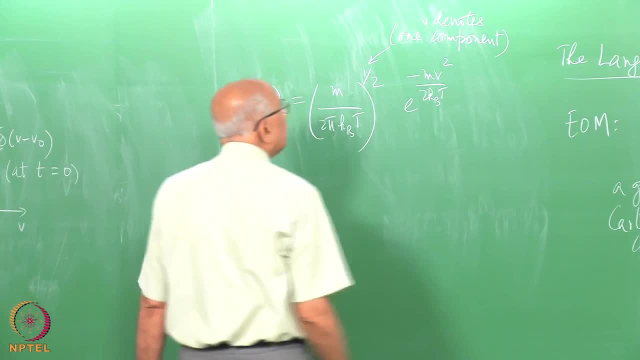 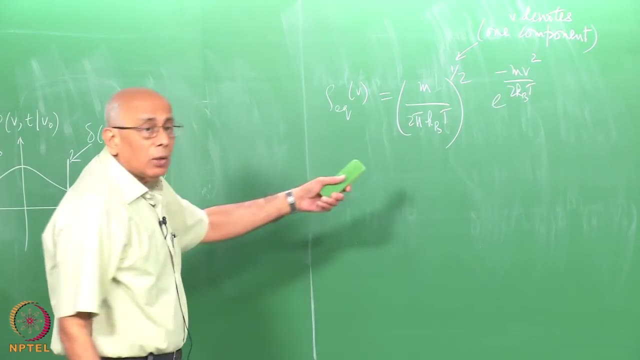 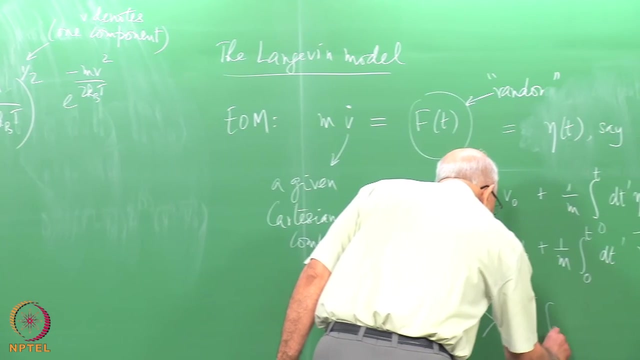 this. So that's the reason for the half here instead of the three halves. But that's a Gaussian symmetric about the point zero. So if I now do this, this v of t, this is equal to an integral from minus infinity to infinity. d v not times v not, which is this. 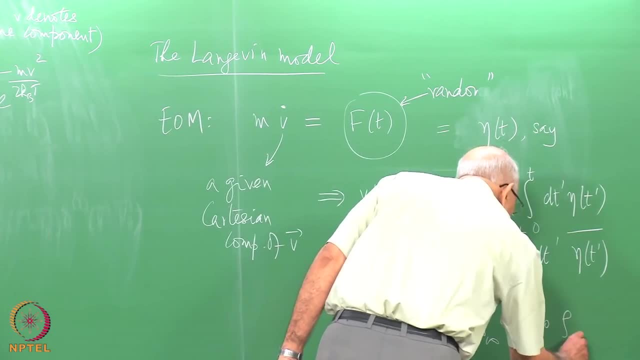 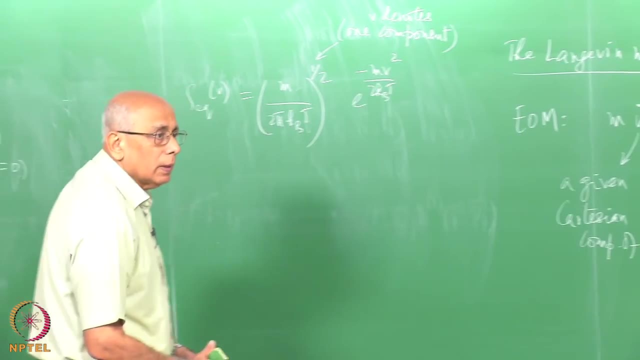 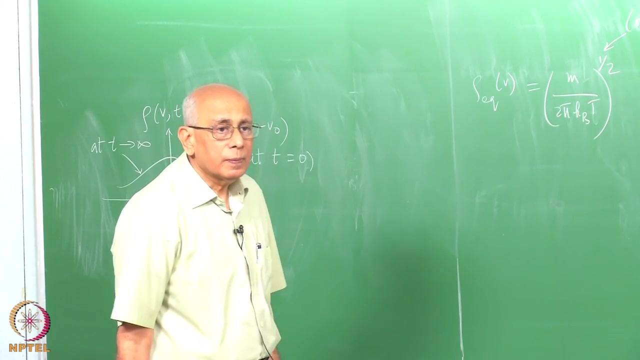 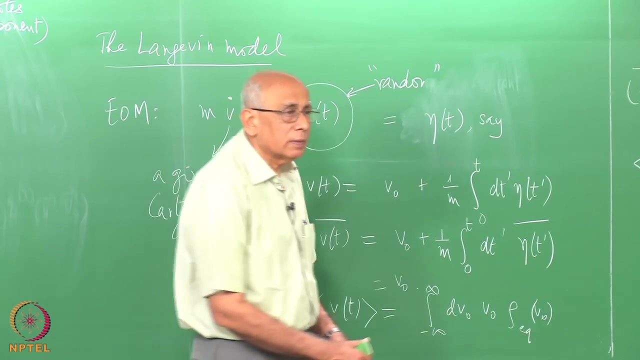 quantity, here multiplied by rho. equilibrium of v, not. And what's the value of that integral? It's zero. And why is that so? Yeah, because this is an odd function and that's an even function, this distribution. So it vanishes, which is: 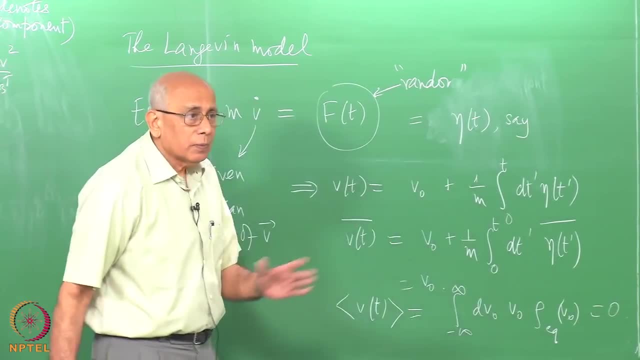 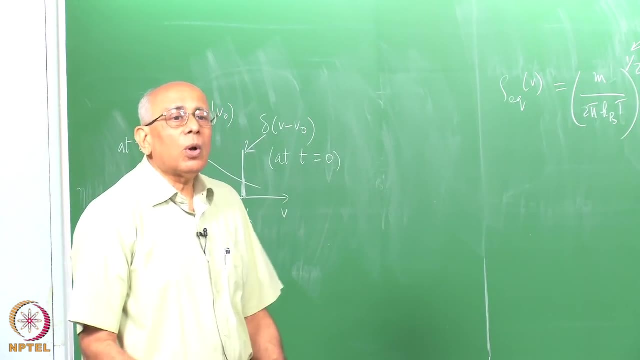 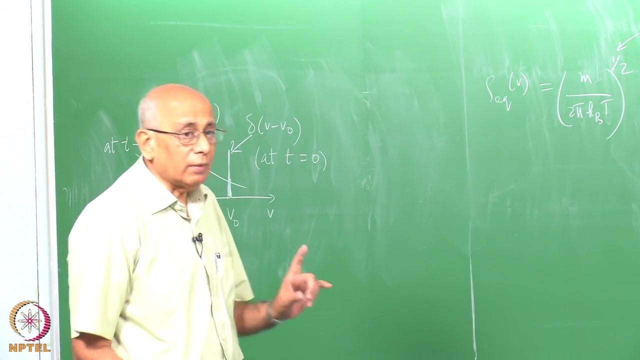 completely consistent. We know that the average value has to be zero in equilibrium And it remains zero at all times. So we are completely Ok, because at no time is it actually moving off anywhere or in a different cells like that. the full average, The conditional average, of course, will start. 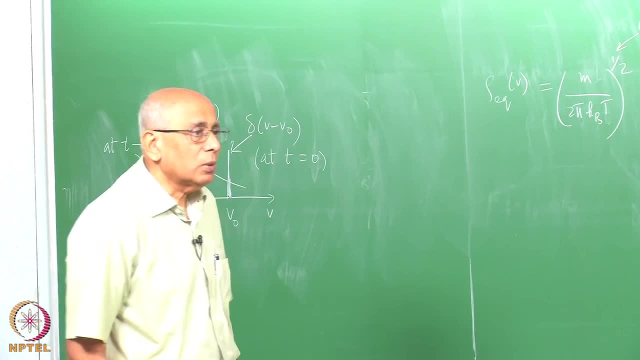 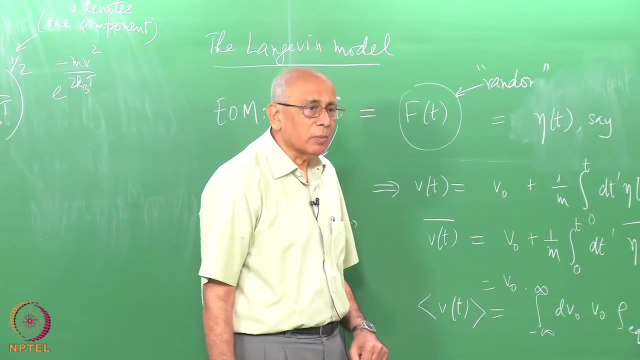 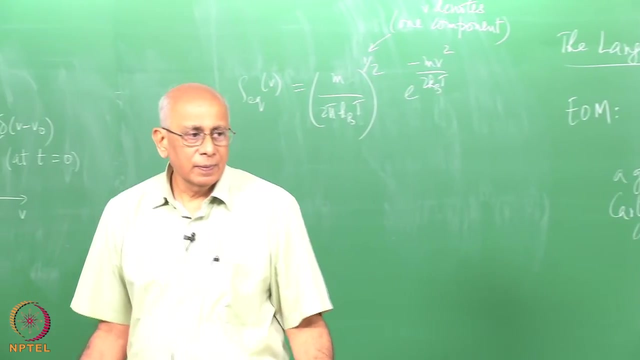 at v, not at t, equal to zero, and perhaps drift towards this, But the full average. since the system is in thermal equilibrium, the velocity is a stationary, random process. It, the mean value, cannot depended on time, Because then it is not a stationary process. Ok, The 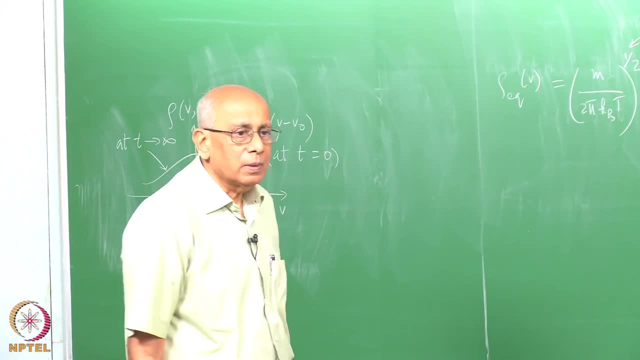 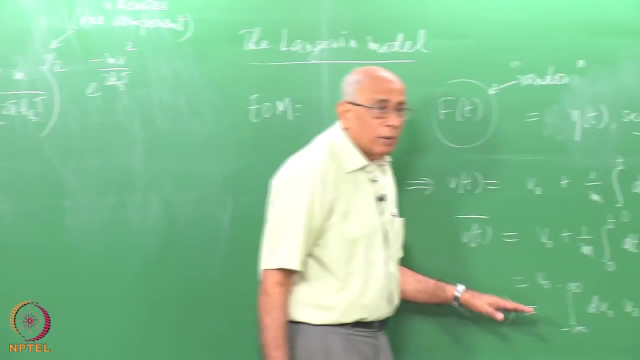 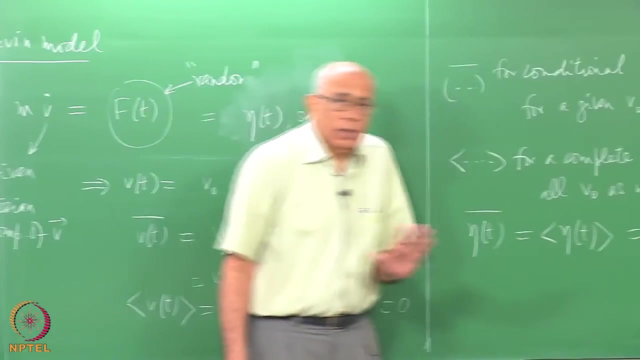 the mean square, mean cube. none of them can depend on time, no moments, and we must check that. So you agree, so far, that this has been perfectly alright so far. In other words, what this has tested is that this assumption is not leading to any contradiction. so far It's. 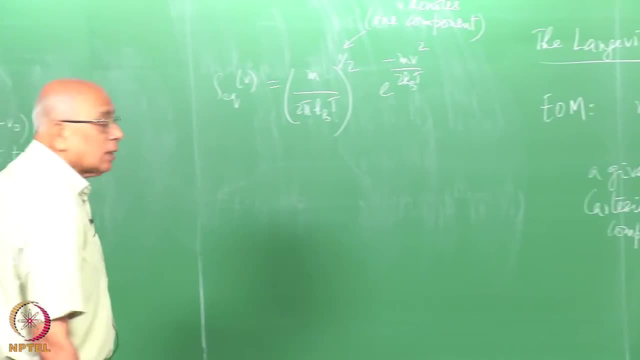 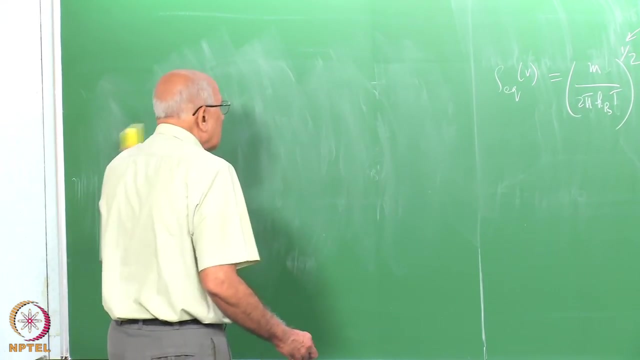 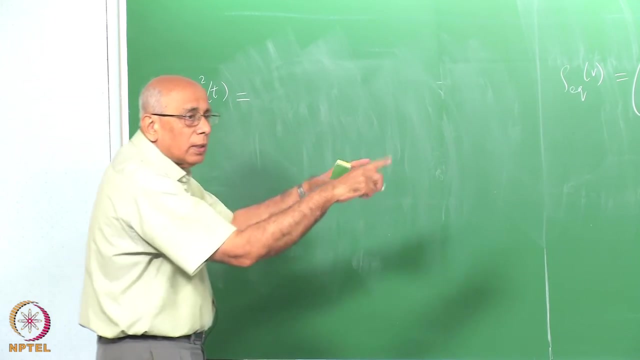 a physical assumption and it seems to have worked. Now let's find the mean square and see what happens. So the next step is to ask what happens to v squared of t. This is equal to: I take this quantity and I square it, so I get v naught squared plus 2 over m times. 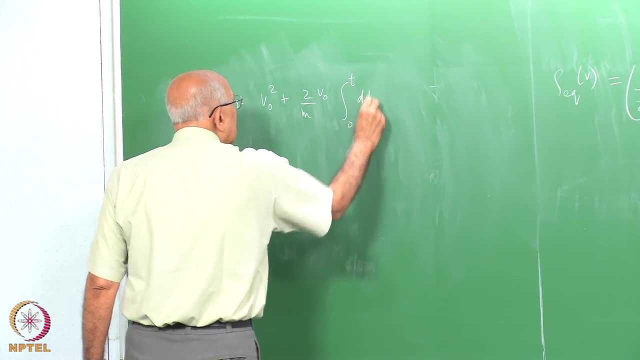 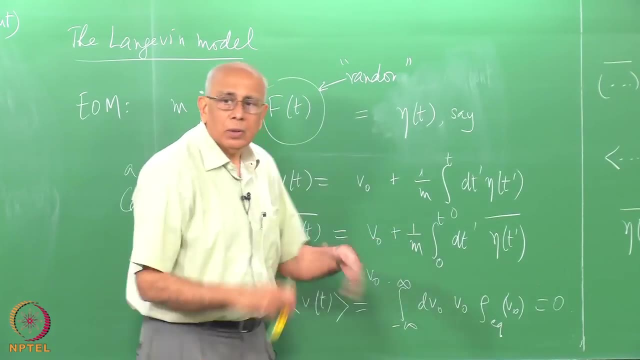 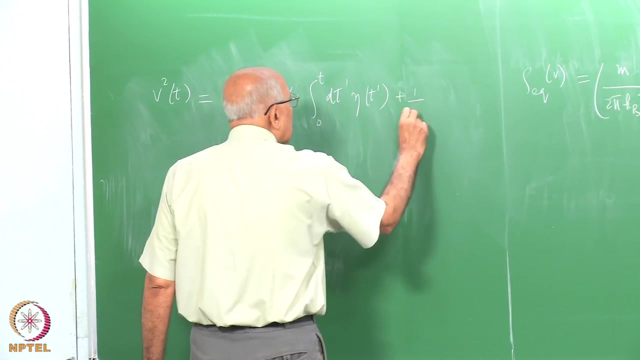 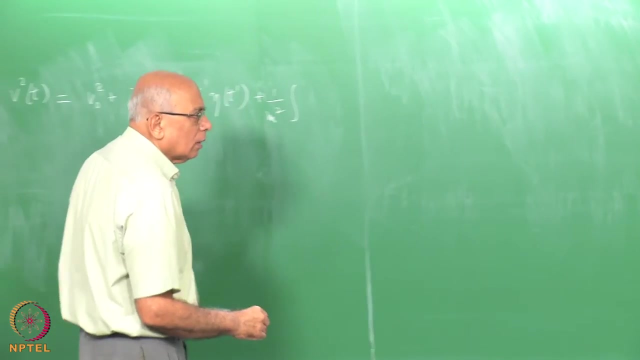 v naught. integral 0 to t d t prime, eta of t prime. So I take this integral and multiply it by v naught. You get twice that, plus a term which is 1 over m, squared an integral. now let's get. 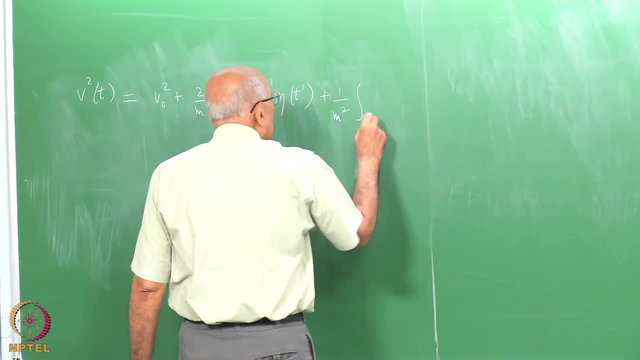 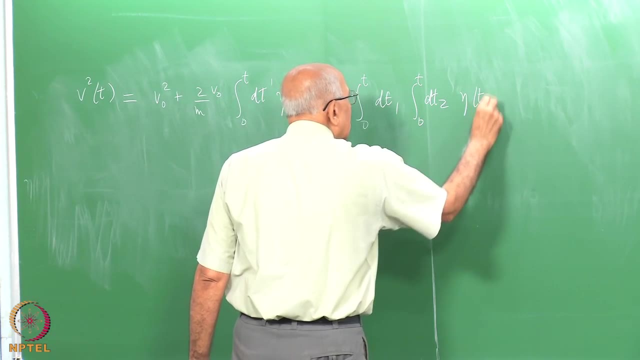 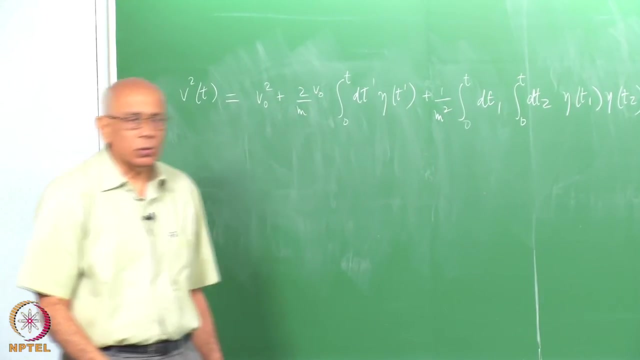 rid of this prime notation and write something sensible: 0 to t d- t 1. integral. 0 to t d- t 2. eta of t 1. eta of t 2.. That's the value of the square. because it's a definite integral. I really have to use two symbols of integration when I want to square this. 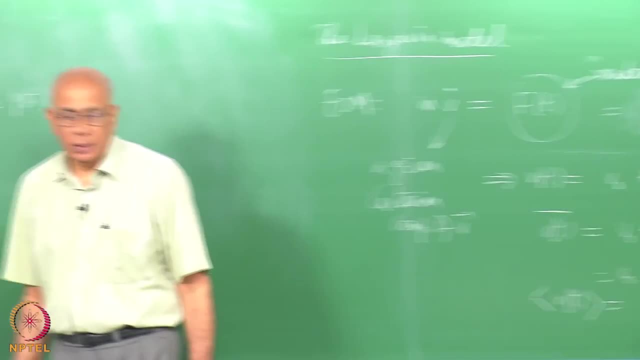 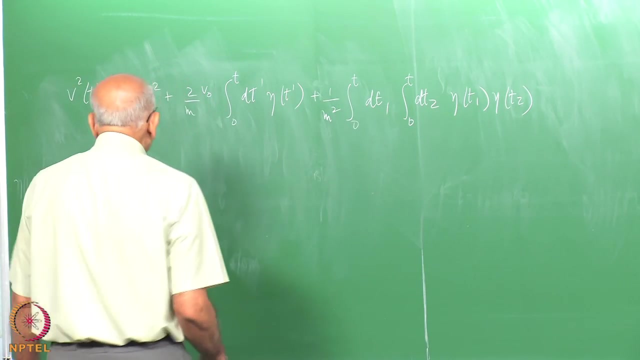 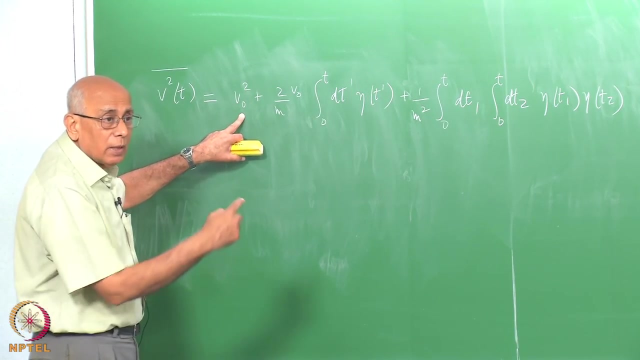 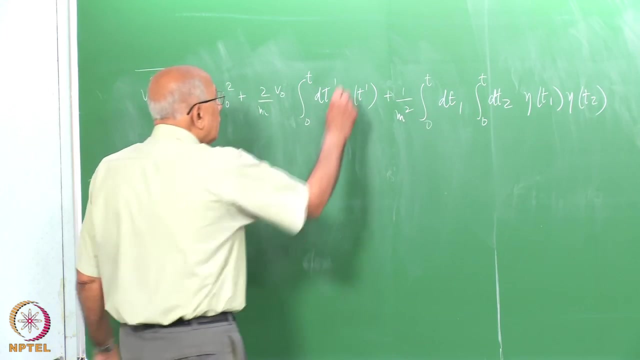 term. Ok, Right Now let's take average, conditional average. So this implies that this quantity, this thing, here there's nothing to average over here, because it's given, v, naught squared is given, And then I average over this. nothing to average here. it averages over eta. But 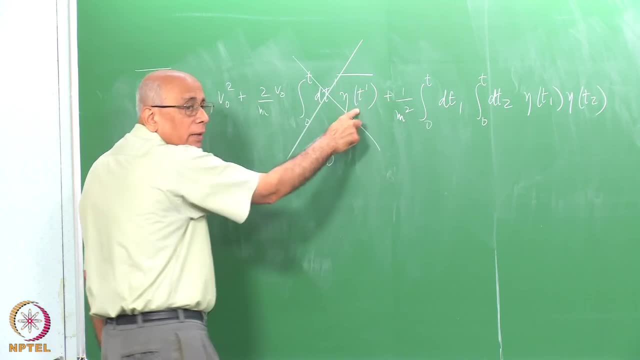 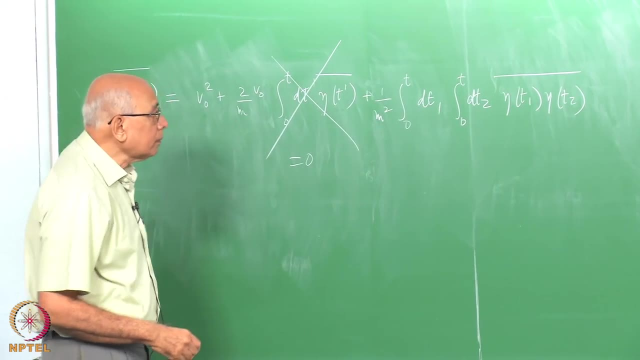 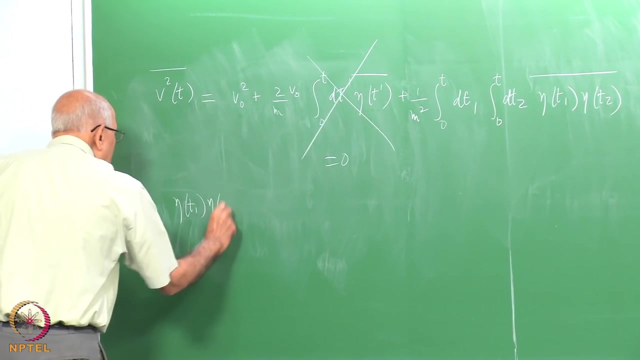 that averages zero And that average is zero because this averages to zero. And then inside I have this average here. So now we need a model. I need to know what is eta of t 1, eta of t 2 average. We know. 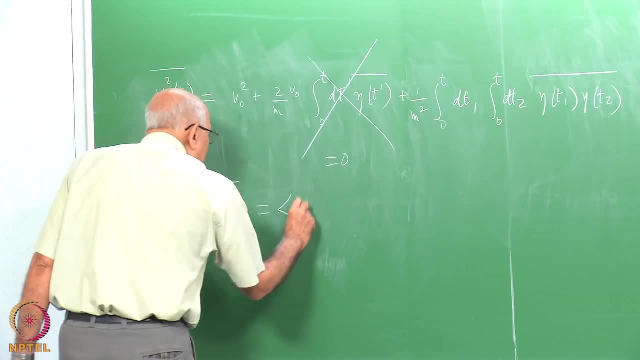 by our assumption that the bath is not affected by this particle, that this is really the same as eta of t 1, eta of t 2 equal to 0.. That's the tenth new integral. I am kilometers away from the p Ziemski kijken hier. that's the third female fraction. a question I'm wondering. 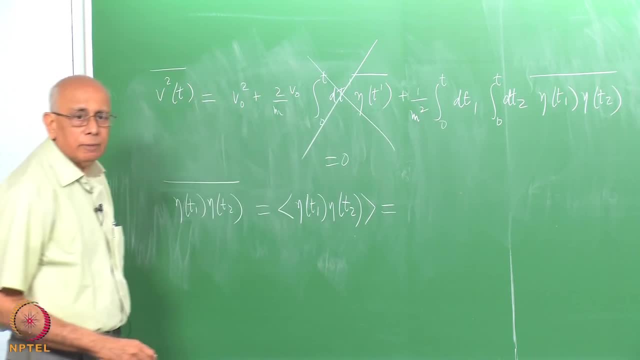 not you. I am looking at points where r is equal to r or a, so I take r over s minus by sesv, p and i concentration with l ABC into q. Now the question is actually: how do you fold? OK, equal to what is the question? Ok, Now here is where the physics has to come in. Ok, And 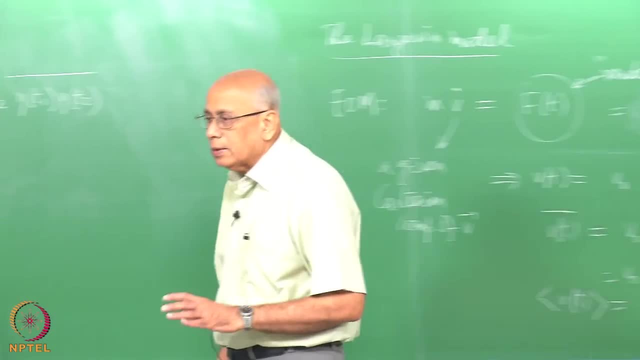 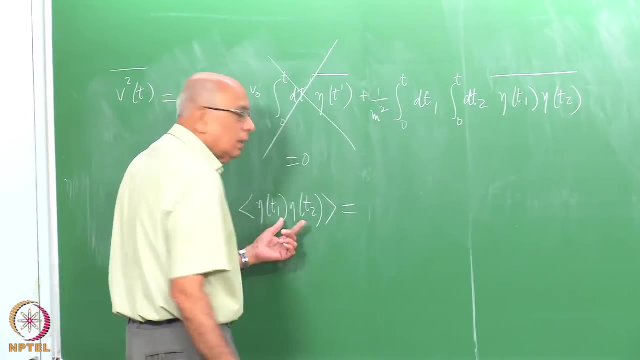 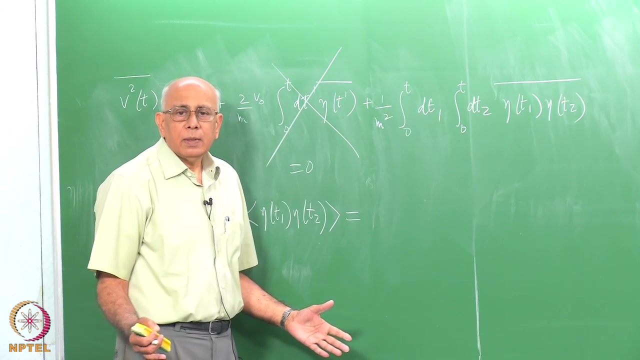 this is why I said this is applicable to a particle whose mass is much, much larger than the mass of the molecules. So the statement is that this noise, which is due to individual molecules hitting this particle, Ok, is completely uncorrelated. In other words, what hits it? 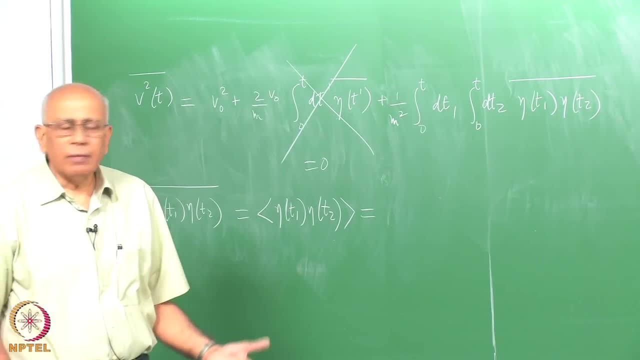 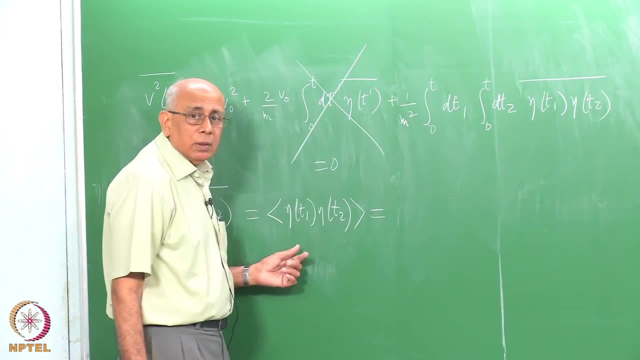 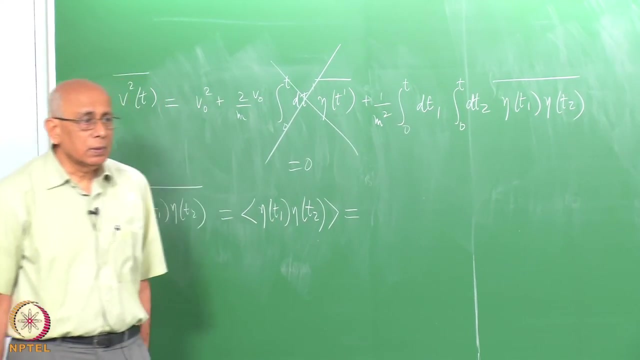 at time, t 1 is very different from what hits it at t 2, and they have nothing to do with each other at all. So this thing here, which is telling you how much of memory sticks on here, is essentially 0 if t 1 is not equal to t 2.. This memory would in fact drop exponentially. 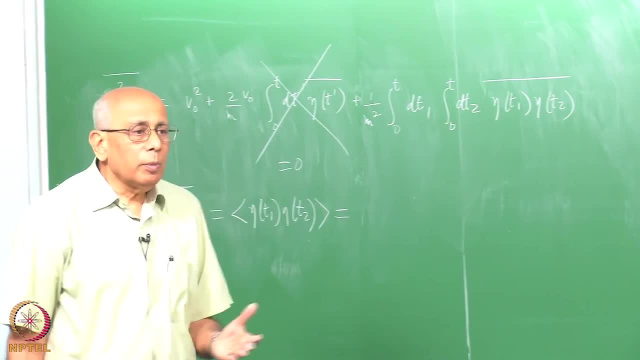 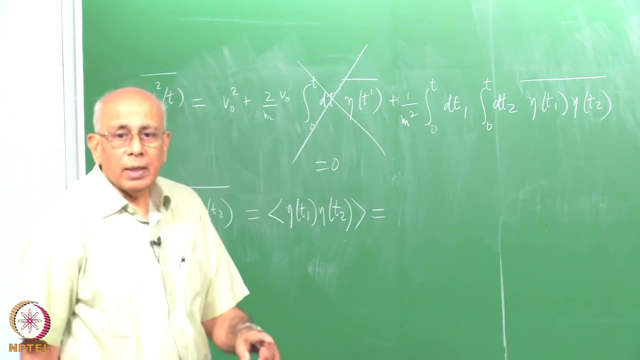 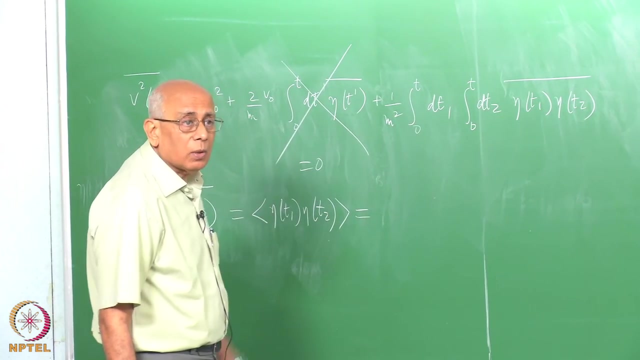 and it would drop like a characteristic time there would be of the order of the mean time between collisions, That's of the order of a picosecond, But we are looking at much longer timescales here, So this is effectively a white noise. That's the whole point about delta: correlated white. 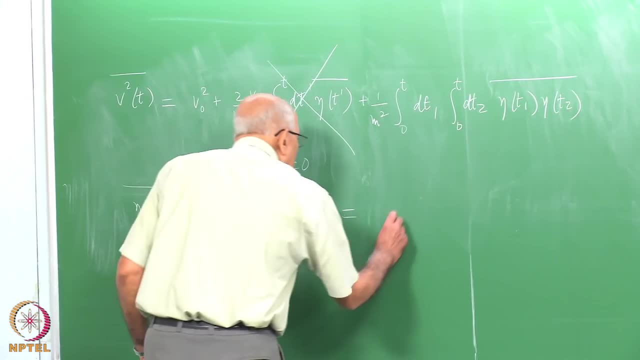 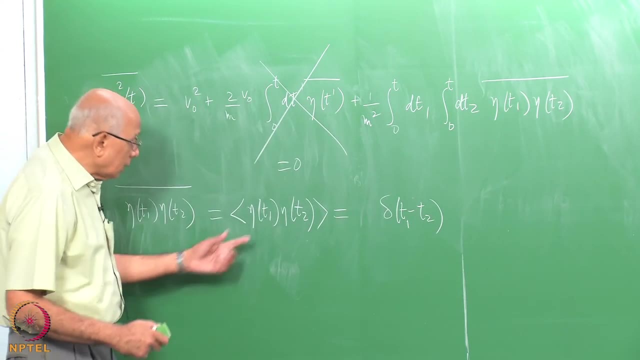 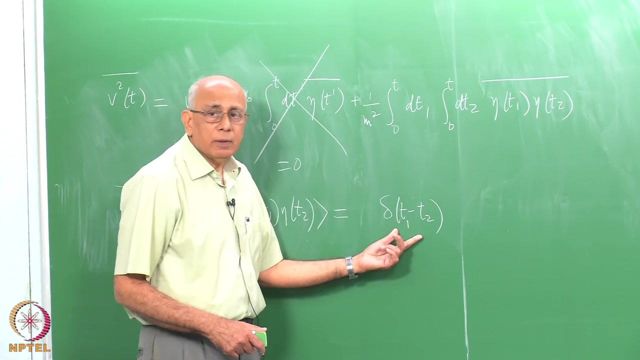 noise, It's true, noise, which is delta correlated, So it's proportional to delta of t 1 minus t 2, which has the wrong dimensions because this is the square of a force. So you need to fix the dimensionality. What's the dimensionality of this quantity? 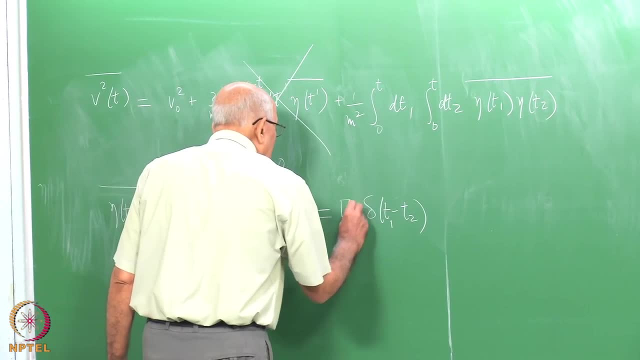 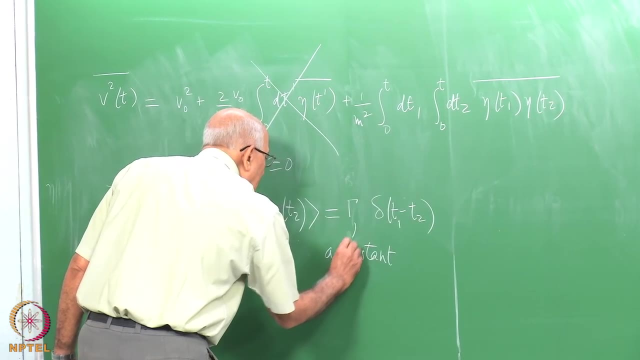 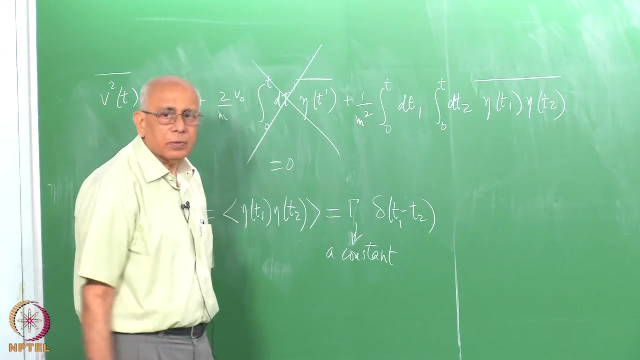 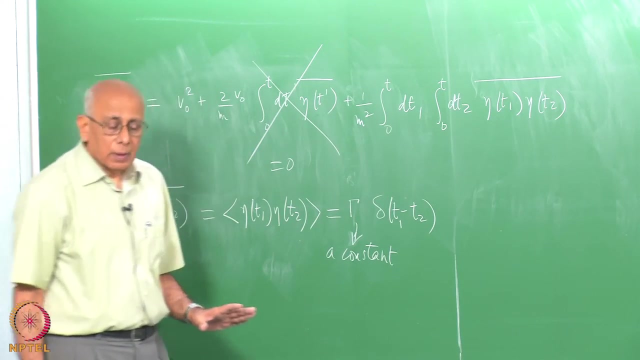 1 over time. 1 over time. So you put in a constant gamma here. This is a constant which tells you in some sense the strength of this force. The larger gamma is, the stronger the force. So this is why I called it a white noise. We will come to a technical definition of white. 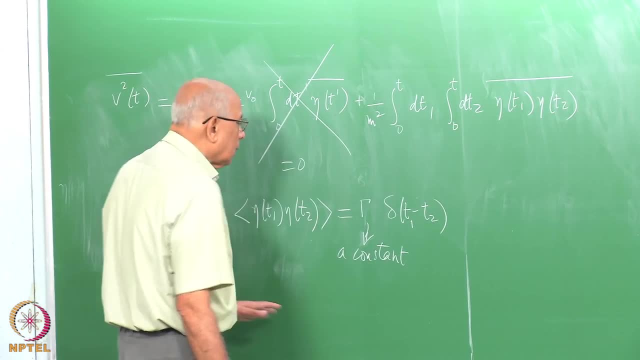 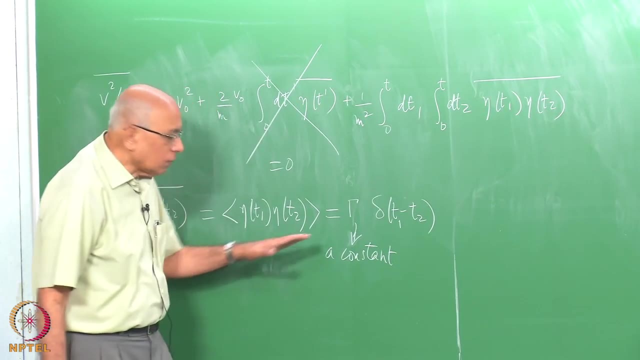 noise a little later, But it's something which has a flat particle. It's something which has a flat particle. It's a power spectrum, essentially a delta correlated noise. We need to make additional technical assumptions about what sort of this is very nice for the correlation function. 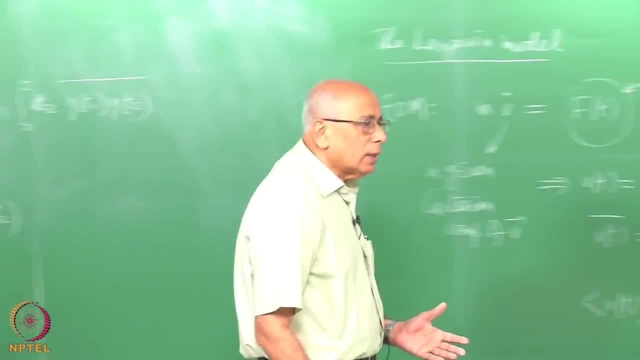 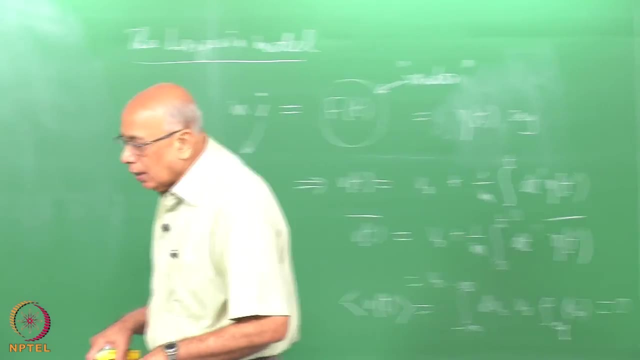 But if you give me a noise, a stochastic process, not only should I tell you all its mean values, I should also tell you all its correlations, an infinite number of correlations at different time, And I should tell you the shape of the probability density functions for this random. 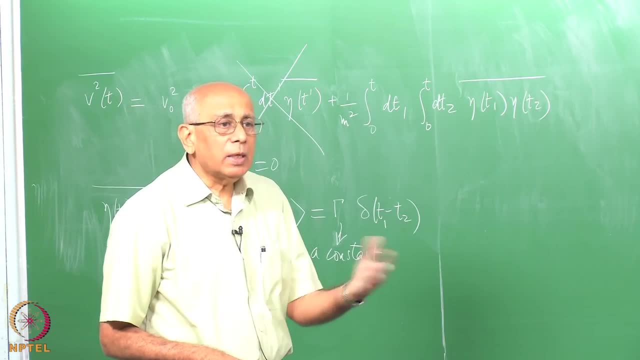 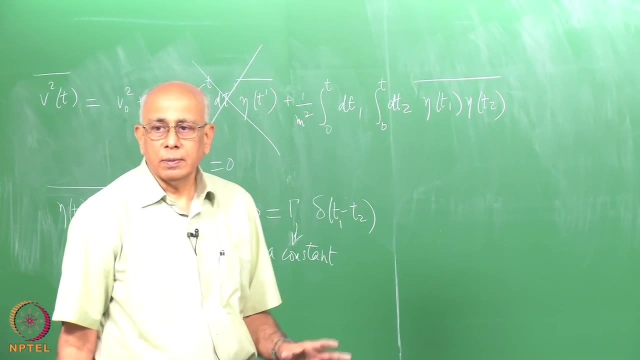 process, Not just one time, but two time, three time, etc. All the joint probabilities I have given you completely, And we will make the simple assumption that they are all Gaussians Because we invoke at this stage the central limit theorem. it says: if you have a large, 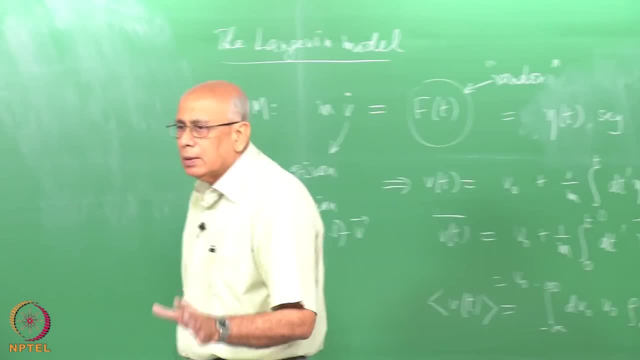 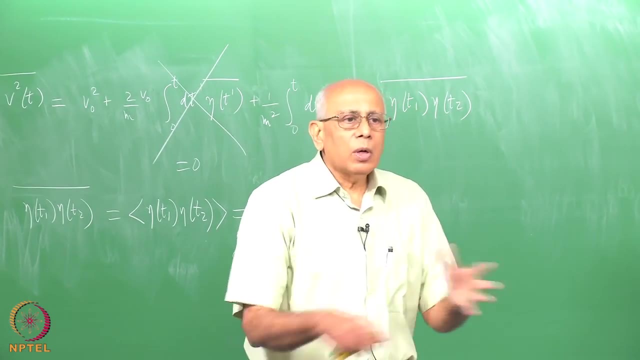 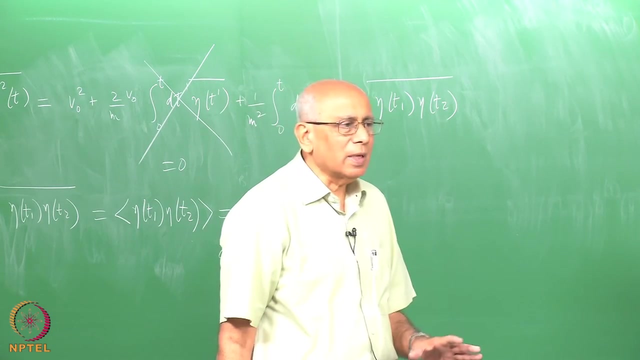 number of effects which are independent of each other and each of them has a finite variance and a finite mean. then when you add them all up in some linear combination, the resultant distribution is a Gaussian. That's, very roughly speaking, the central limit theorem of statistics. 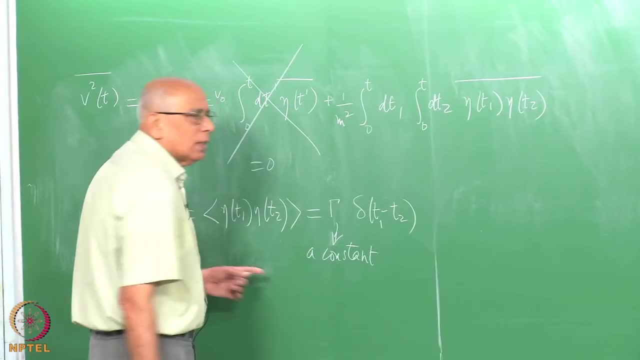 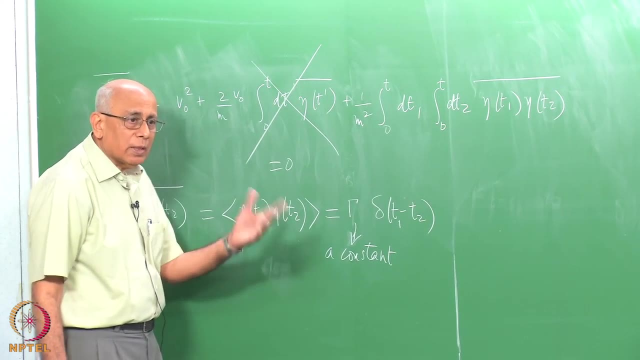 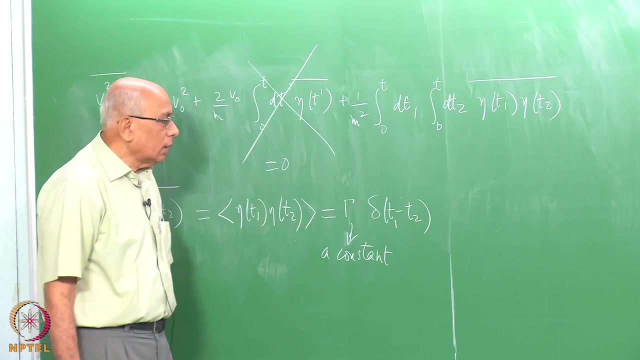 We will invoke it when the time comes, But right now we need just this assumption about the correlation. Notice that this is a function only of T 1 minus T 2, what I expect stationary noise. It's also a symmetric function of T 1 and T 2, it doesn't matter which came first. So 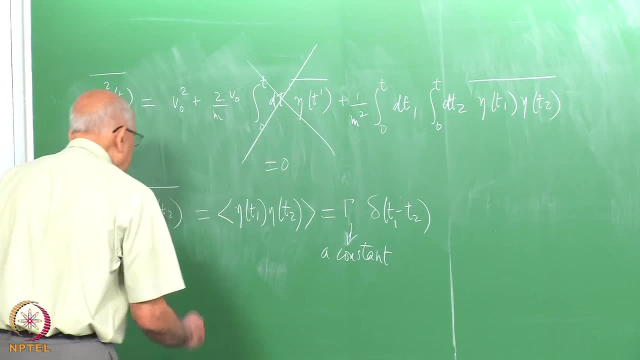 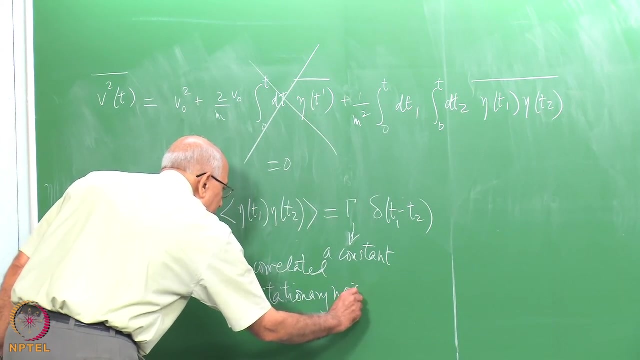 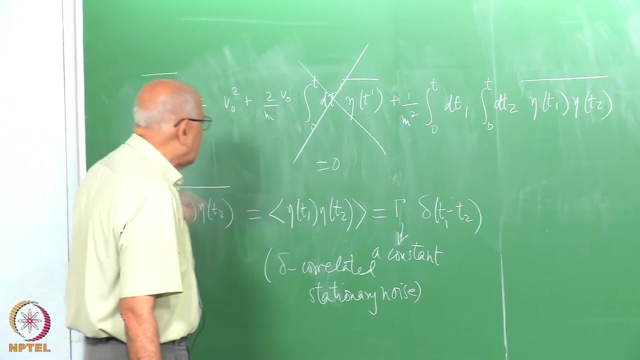 this is the one assumption that I have been talking about. Delta correlated noise stationary noise Stationary because its statistical properties don't change as a function of time. So all these, the average value 0, this is a function only of the time difference. the three point: 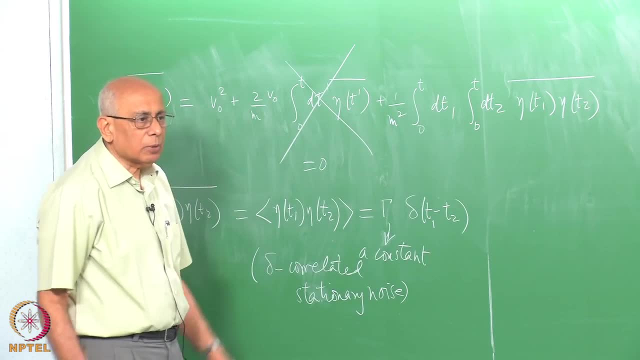 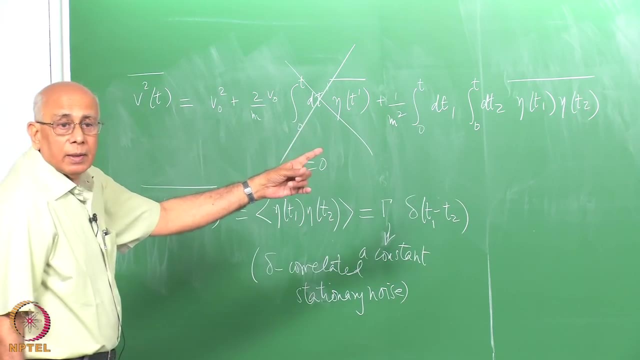 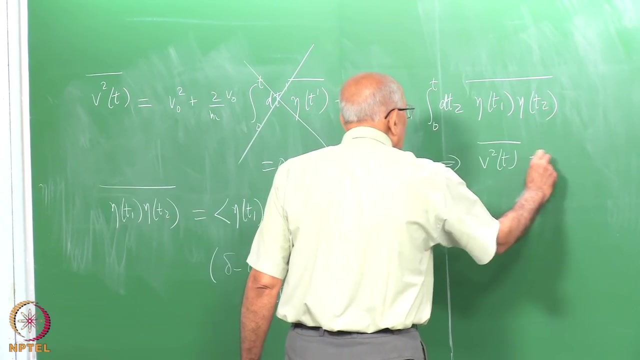 function will be a function only of two time differences, and so on. The absolute origin of time doesn't matter. So let's put this into that and see what happens. So I put that in. This implies that V square of T average is V, not square plus 1 over m square. and now 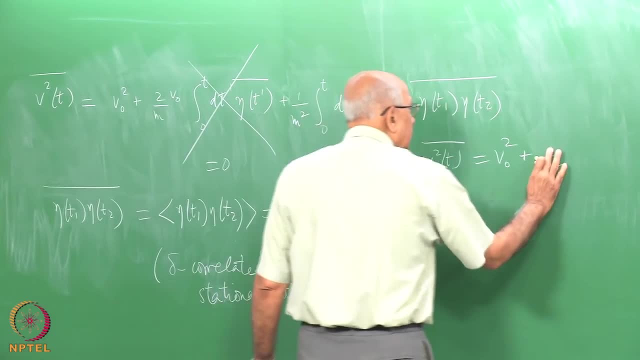 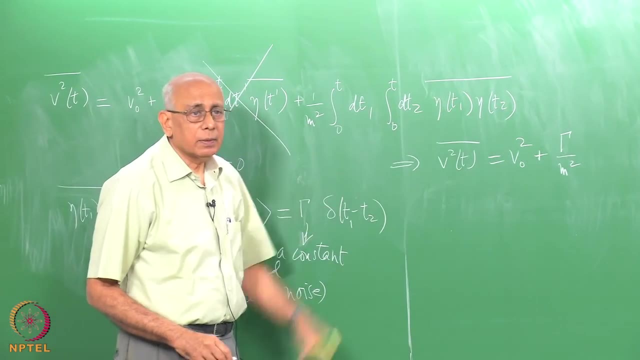 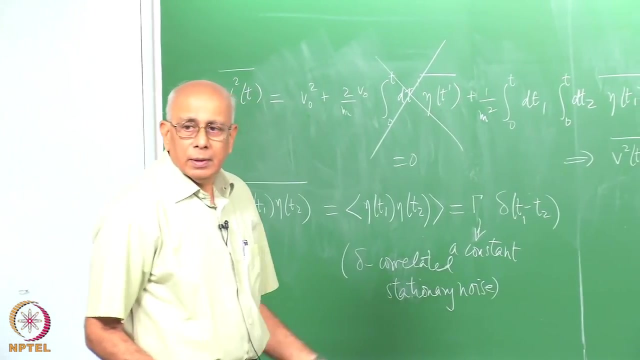 I've got to do this integral. The gamma comes out and I have to do a delta function integral inside here. Ok, But the delta function just says: replace T 2 by T 1, right, And you have to be careful here again, You have to be careful here. You need to be careful here, So you 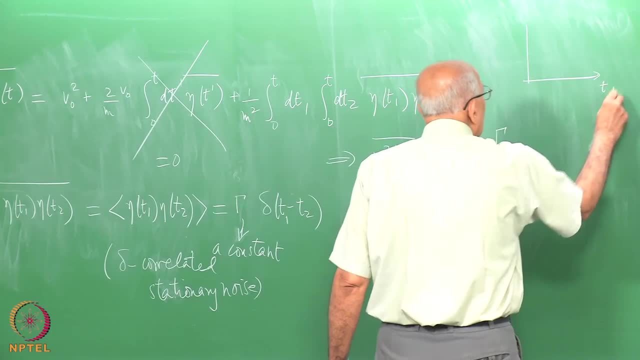 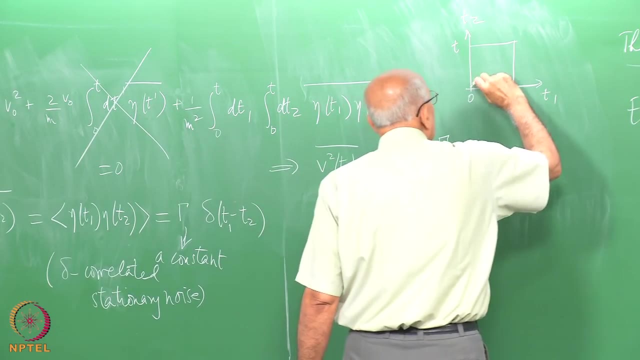 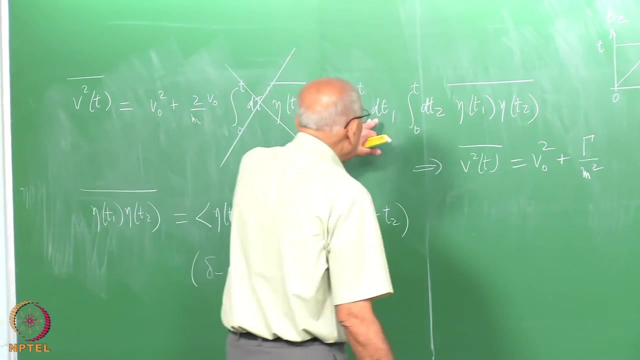 again, because if I plot t 1 here and t 2 here, the integral runs from 0 to t in each of the variables. and that's the line, the 45 degree line, is a line on which t 1 is equal to t 2.. And now, if I do the t 1, t 2 integration first, it means I fix a value of t 1 and I 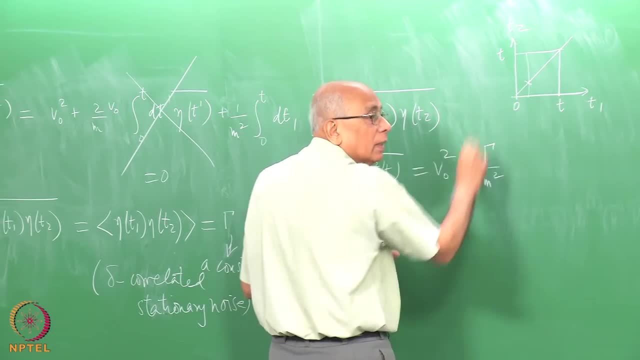 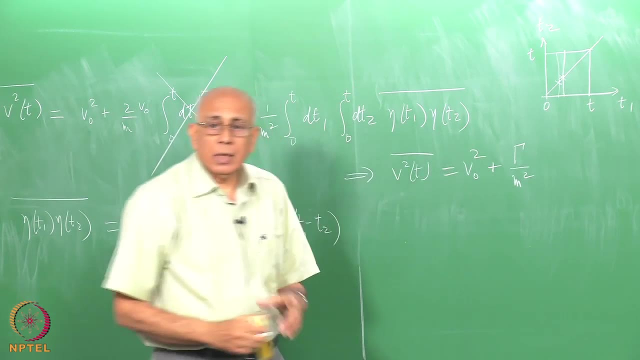 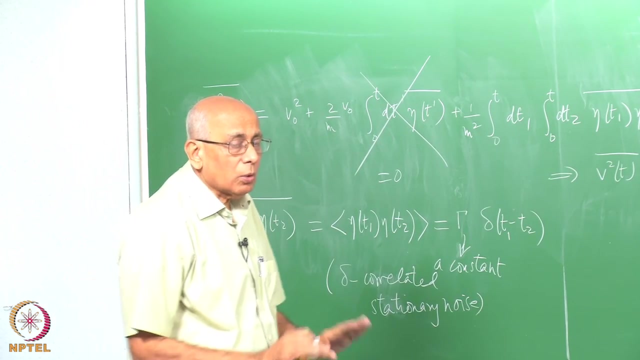 integrate in t 2 from 0 to t and the delta function fires here I go to the next value of t 1 and the delta function fires here, etc. So it is clear that through the range of t 1 from 0 to t there is the delta function fires for every value. So I can close my eyes. 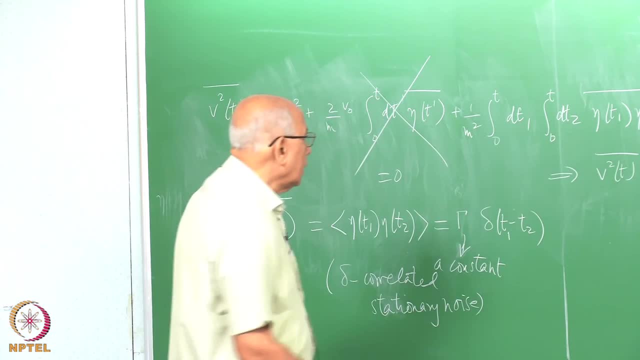 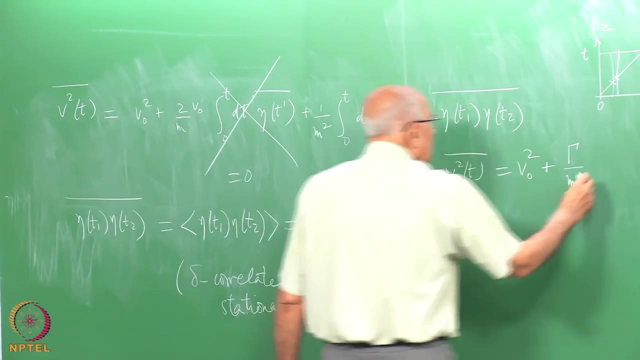 and remove t 2 and put t 1 wherever it appears right And of course there is nothing to put. there is no t 1 here, it is just a delta function which goes to 1 and I get an integral 0 to. 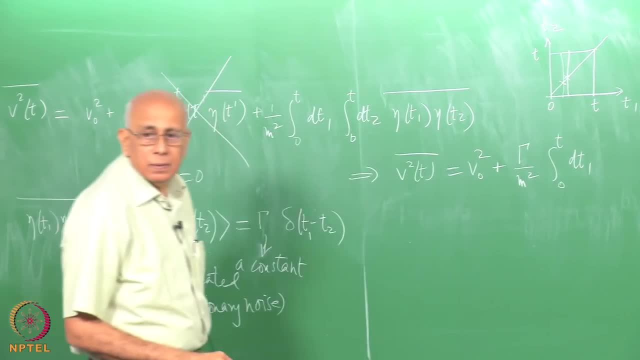 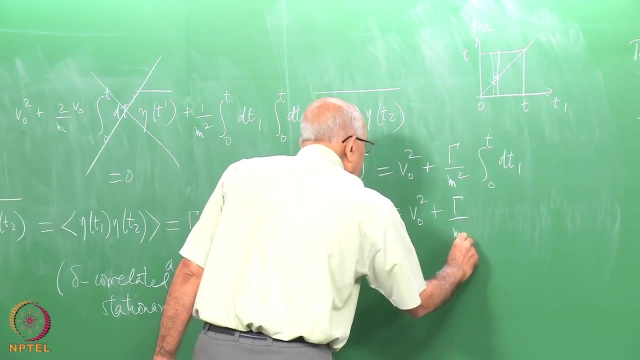 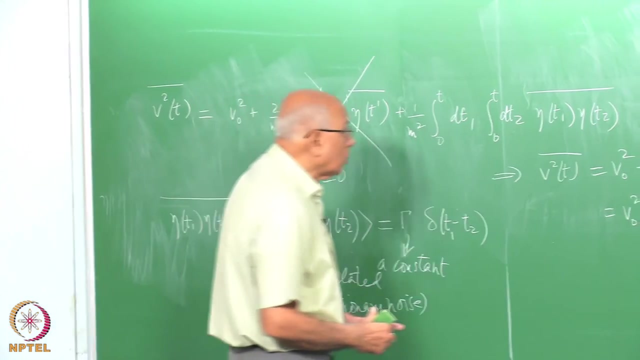 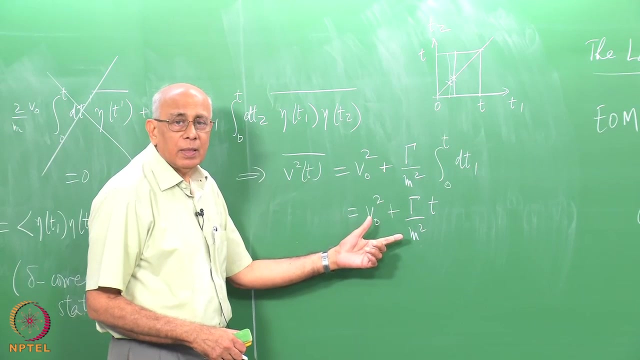 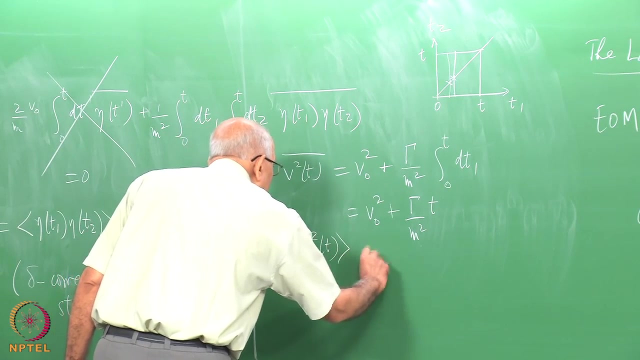 t d, t 1, Ok, Which is v not squared plus gamma, over m square t. Very bad news, because this is now telling you that for this initial condition, this fellow is actually increasing with time linearly. And now, if I average and do this, v squared of t, this is equal to an average over v, not. 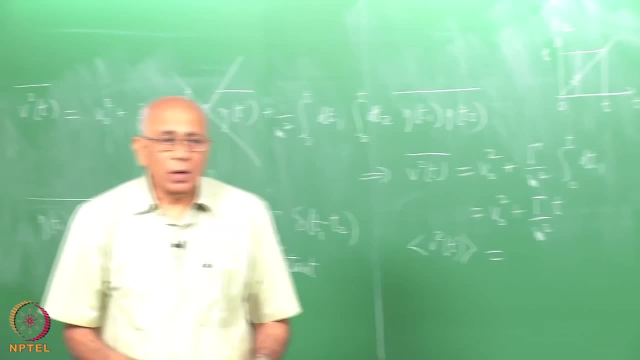 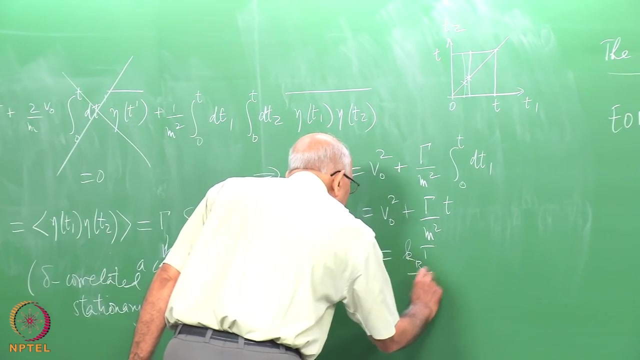 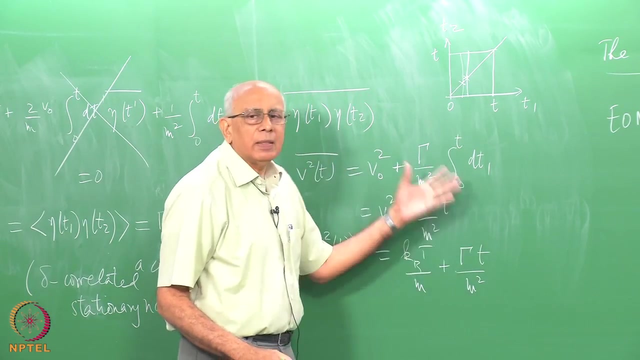 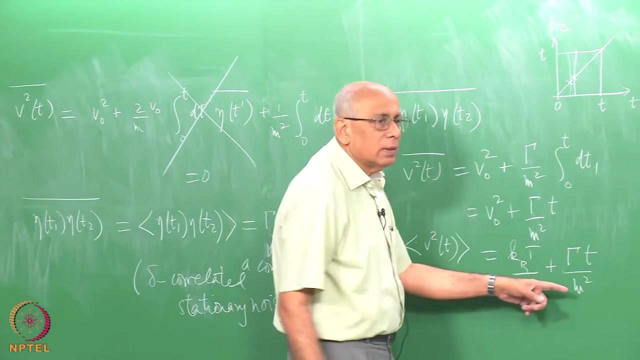 squared. So I can do this, which is just the mean square value of the velocity over the Maxwellian, and that is k t over m plus gamma t over m, squared. There is nothing, there is no v, not dependence here. So the average value remains where it is and it is this thing here, And 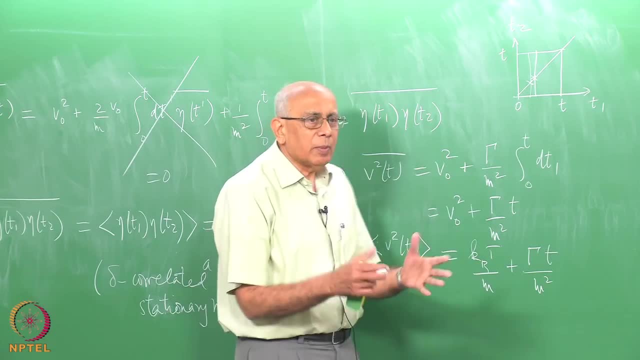 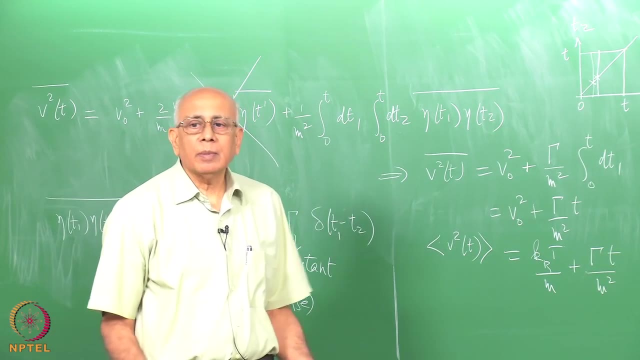 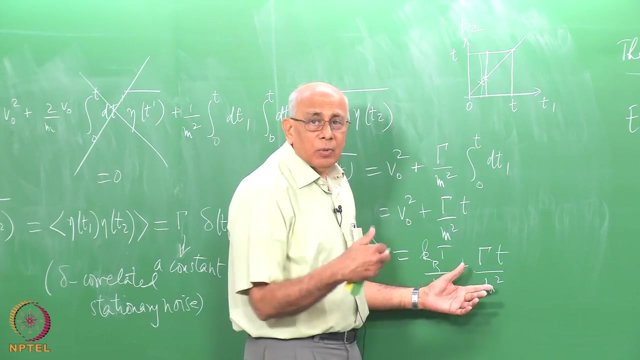 it is completely unphysical because it says: if you leave this beaker of water alone, put the colloidal particle in it, then its energy, the particle's energy, will spontaneously increase till it becomes infinite, as t tends to infinity. So it is actually taking energy from all the 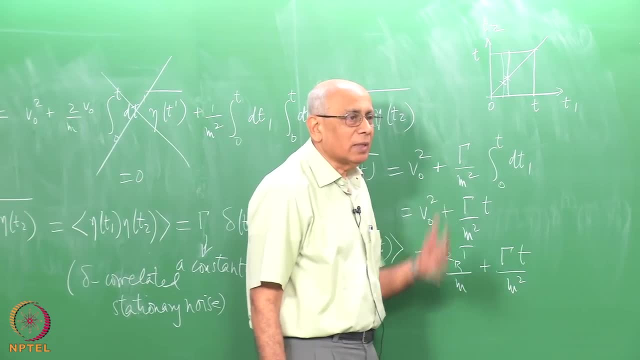 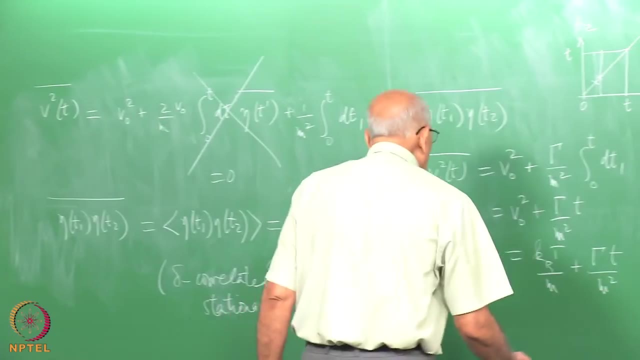 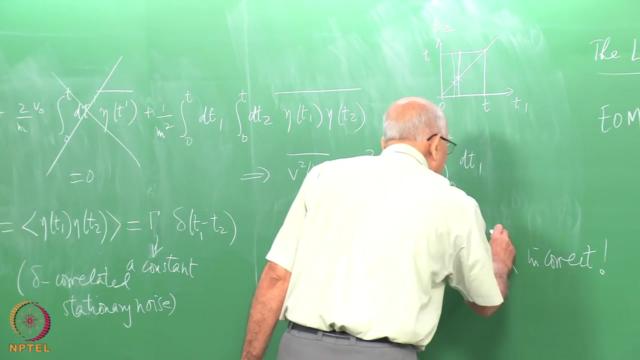 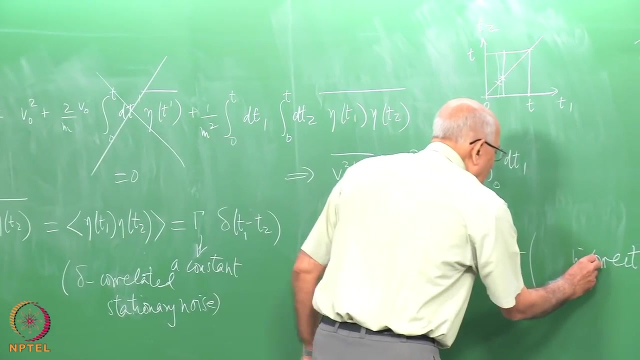 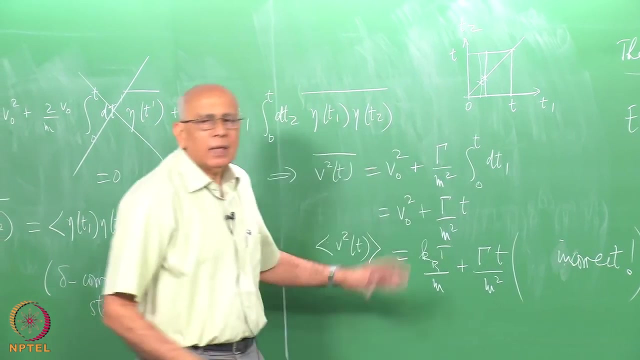 molecules and reaching infinite temperature or energy, if you like. Ok, which is wrong? This is just plain wrong. So this is completely wrong, Incorrect or incorrect. So this is: What do you think has gone wrong? So this is fairly incorrect. 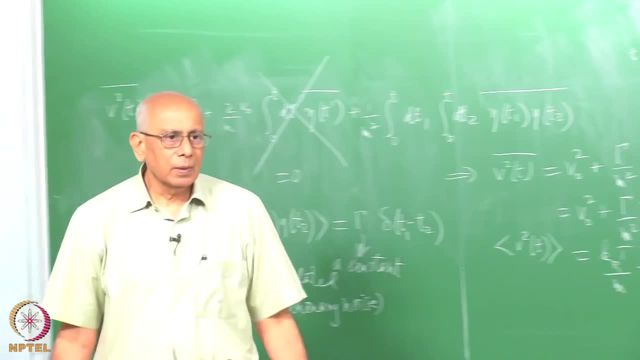 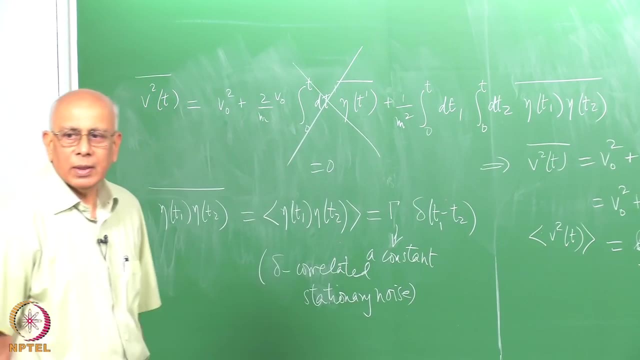 It is clear that some assumption there made. there is wrong, one or more assumptions. So what assumption do you think is wrong? We will eliminate it one by one. What assumption do you think is wrong? One possibility is that this is not correct. 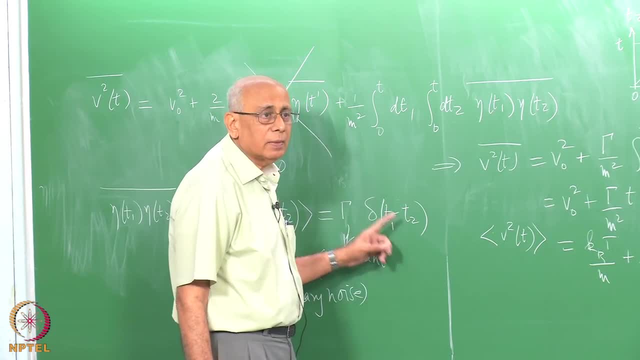 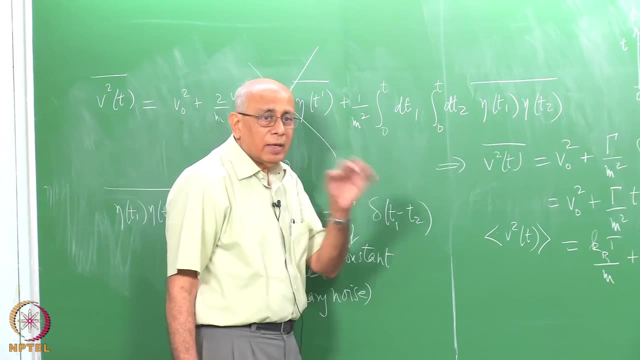 A very strong possibility is that this is not right. This is really not doing this at all, but it has got some exponential correlation. It is a finite time. It cannot be. there is no such thing in real life as a delta correlated noise, because there 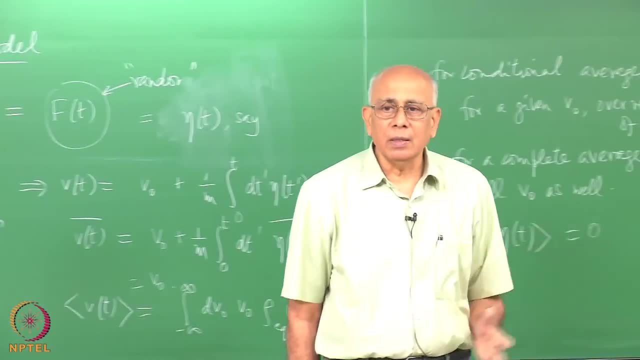 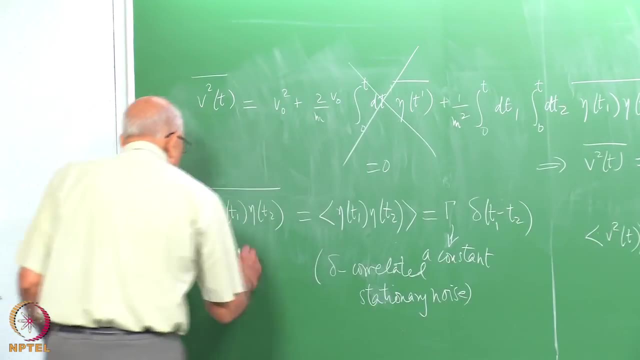 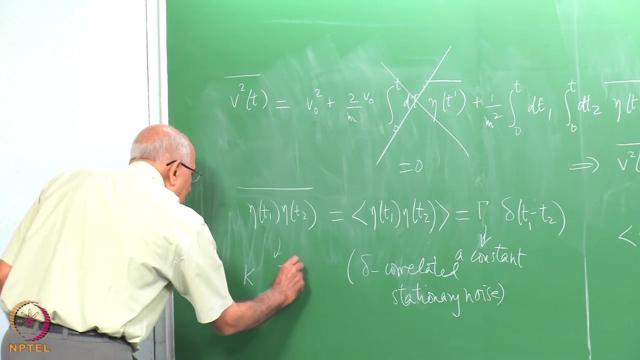 is some correlation time. no matter how small, It can never be mathematically zero, right? So that is the first step. So let's do that, Let's say that this quantity is not that at all, But it is some other constant k times: e to the minus t over tau, e to the minus mod. 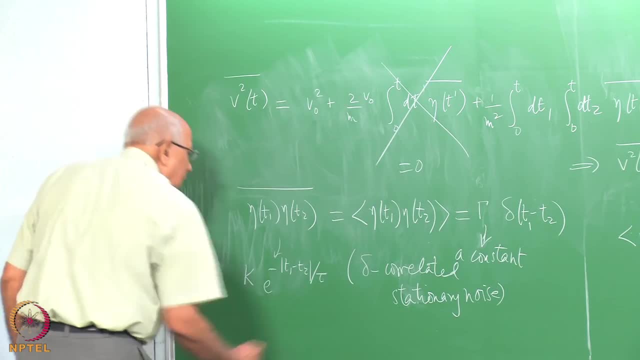 t 1 minus t 2 over tau. That is a symmetric function, It is stationary and so on. So we could say, good, we will put this in. So this integral is not so easy. Instead of a delta function, you have got to put this in. 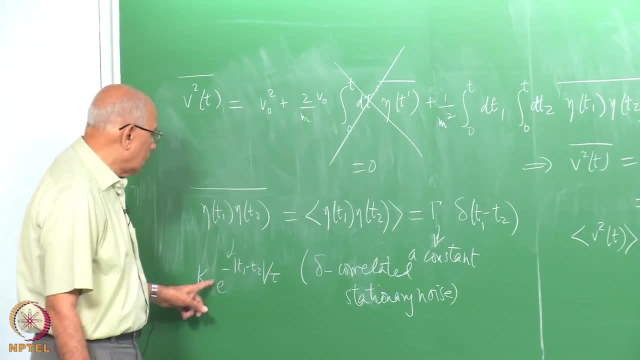 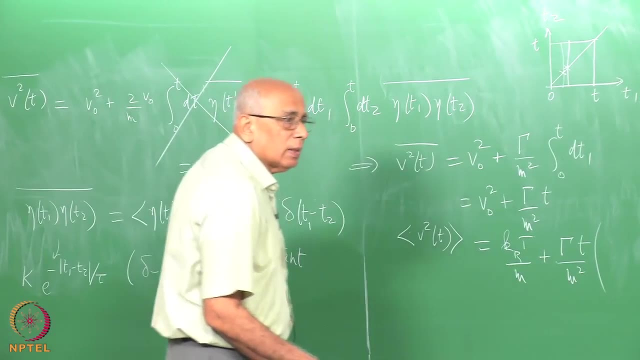 Let's do it, Let's do it, Let's do it. I will leave you to check that. you can do this integral once again now. It is a very reasonable assumption to make. It is an exponentially decaying function instead of just a delta function. 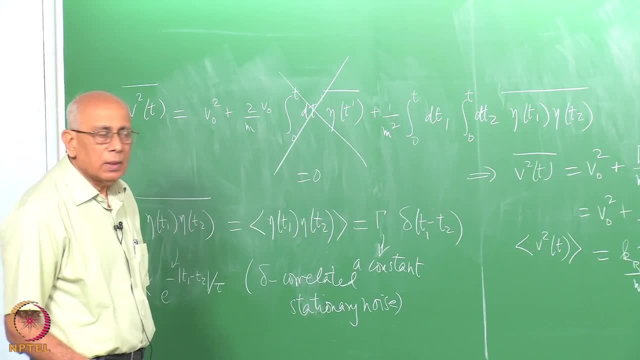 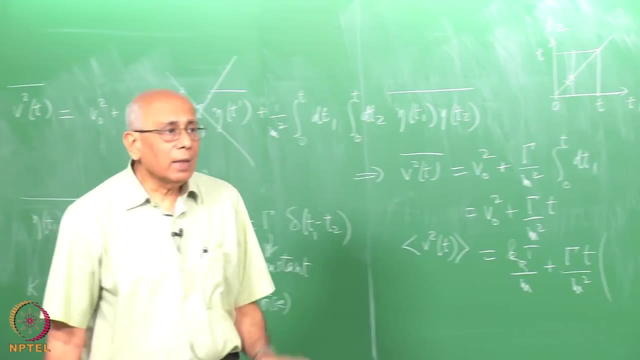 And one can say, alright, let me do that integral now and see what happens. A little more hard work, because you have to do both integrals, t 1 and t 2.. But I will leave you to check that you will again run into exactly the same problem. 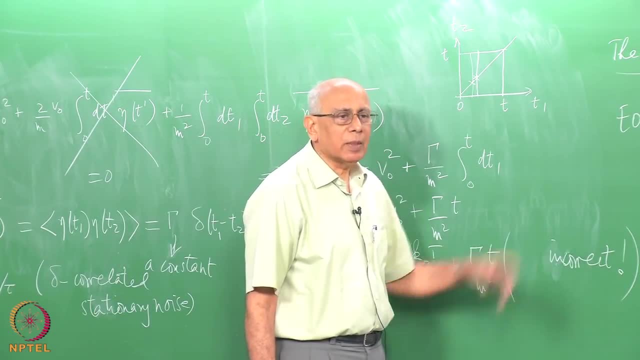 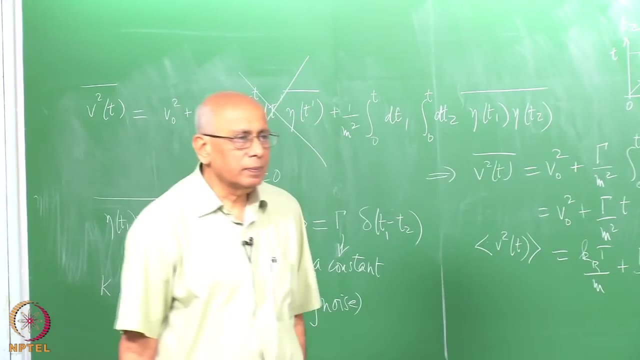 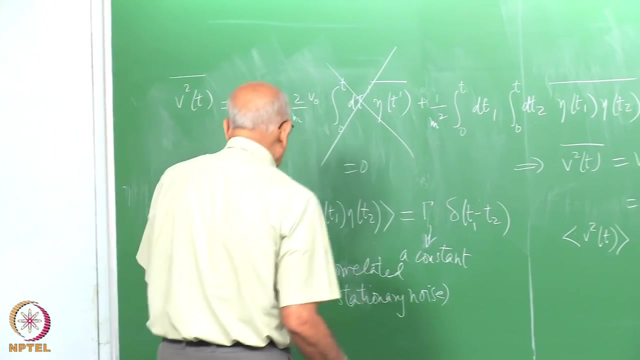 This. it won't quite be. it will be a little more complicated explanation, But there is no doubt that eventually you will end up with something that increases with t and doesn't stay in equilibrium. So check that the incorrectness of this model is not due to the assumption that this noise 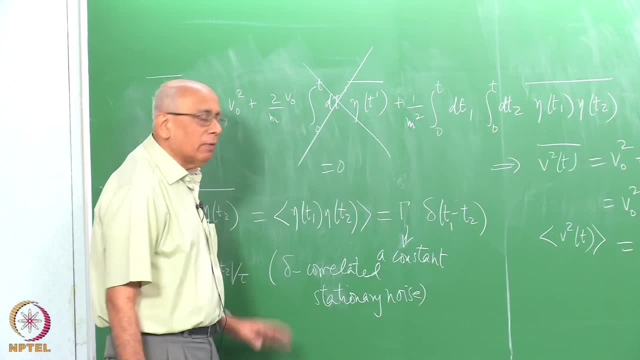 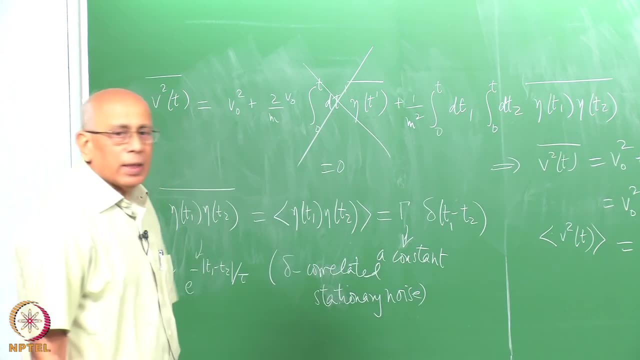 is delta correlated. Even a finite correlation time will still produce the same thing. So that is an exercise for you to check out, But it still does it. So that is out. That explanation is ruled out. What is the other possibility? What other possibility is there? 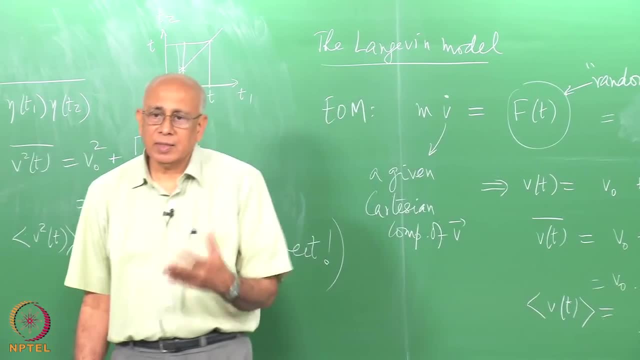 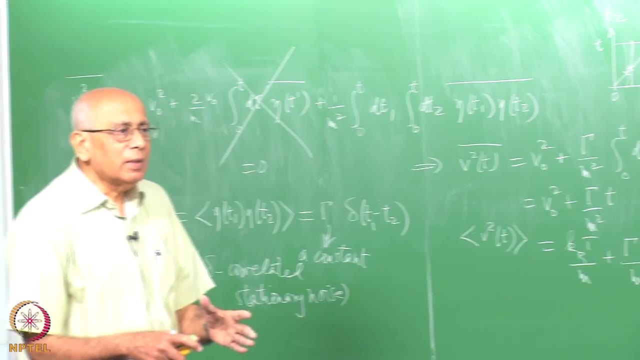 Would you say Newton's equation is wrong? No, it is a classical particle. It has to satisfy Newton's equation. Would you say the fact that the mean value of the velocity, the noise, is zero is wrong? No, that is not, because that will just remove the mean value of the velocity itself will. 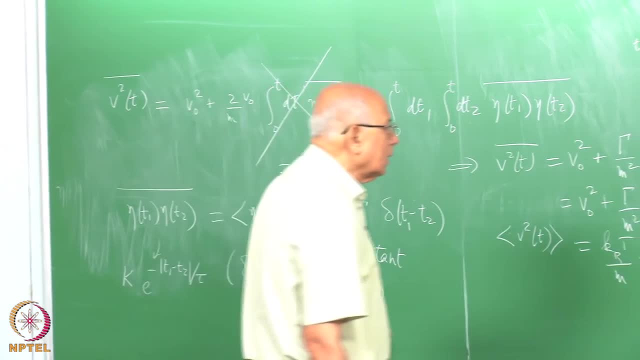 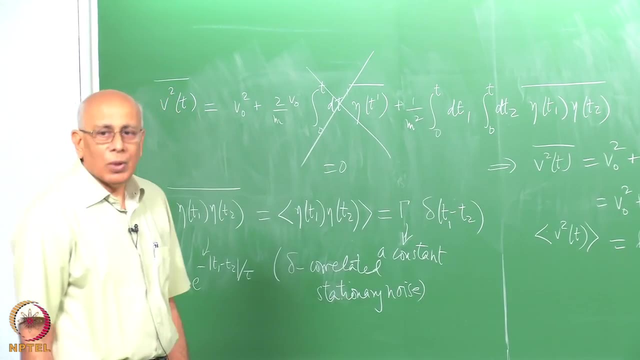 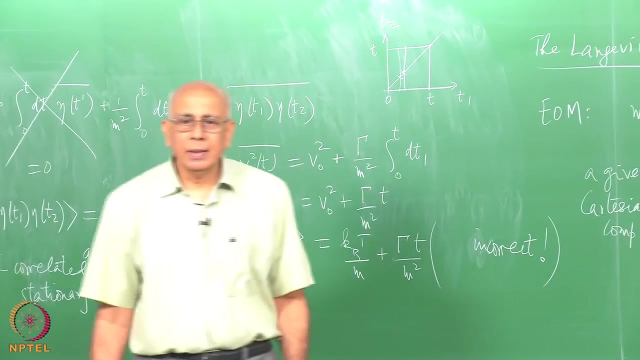 disappear will not be correct if you do that. Ok, So we have ruled out all the other possibilities. So what do you think is wrong? If the particle is moving in the fluid, it will probably have a drag. Yeah, So there are subtle effects like that. 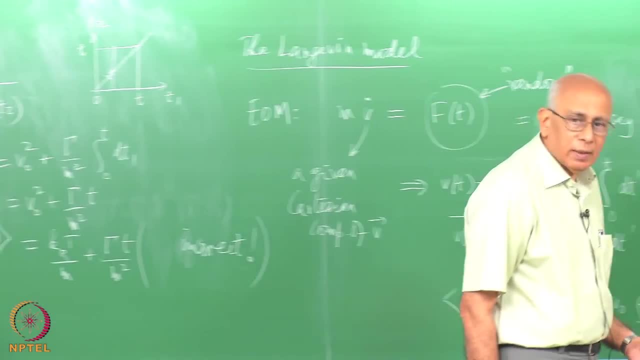 There is a back flow. there is all kinds of complications like that. There are many, many such effects. There is a reaction on the particles, definitely. There is certainly a back flow and a reaction on the bath particles. Ok, Thank you. 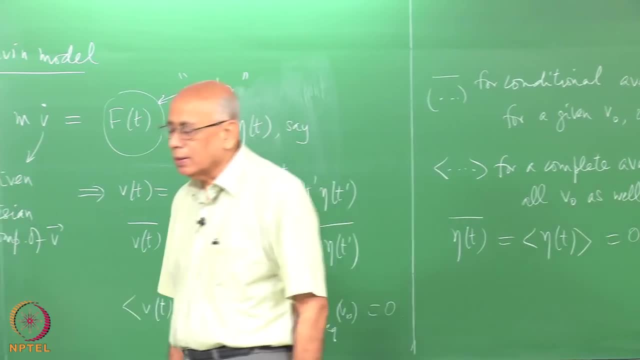 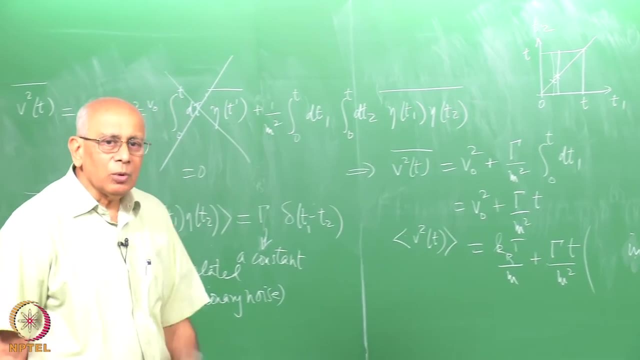 Thank you, That is not taken into account here, But that is not the reason in this case. One can take that into account in some fashion, but it is not. But the other statement you made, that there is a drag on. this is certainly a place to. 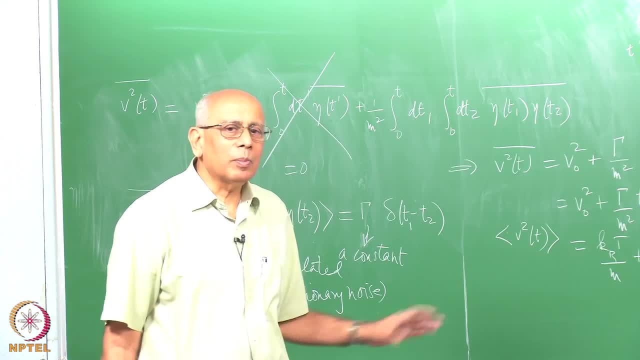 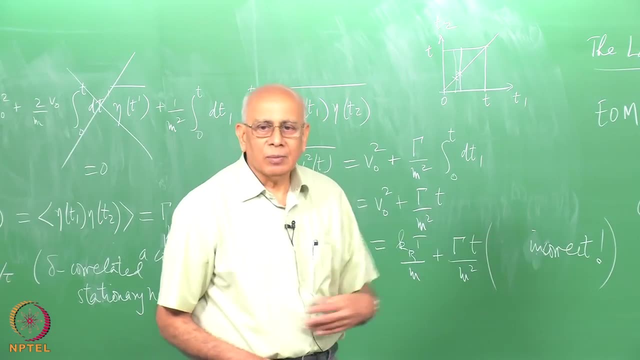 pause and give some thought to it. How does this drag show up in this model? How will it show up? Well, imagine this particle. I am the particle and it is one dimensional motion, so I move this way. It is not being buffeted on both sides by molecules. 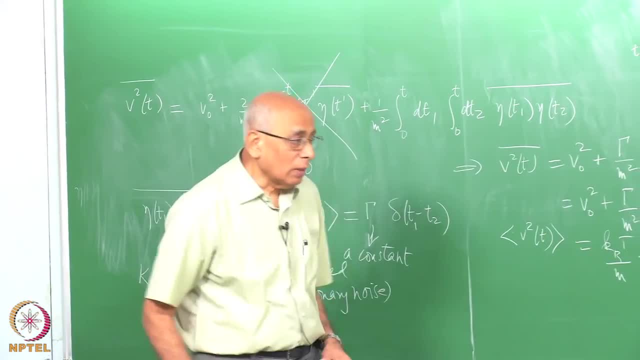 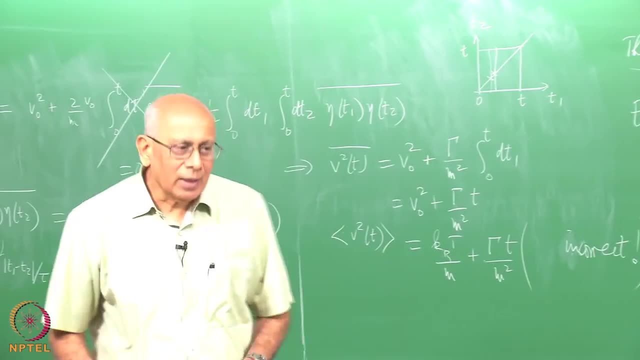 What happens if I move relative to these particles in one particular direction? What happens when you walk in the rain? and the rain is coming straight down but you walk, Where do you get wetter? in the front or at the back? In the front? 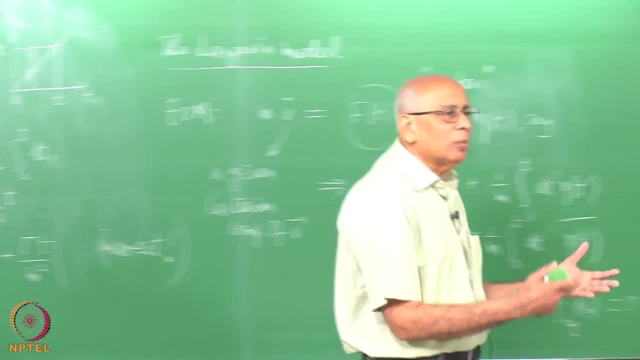 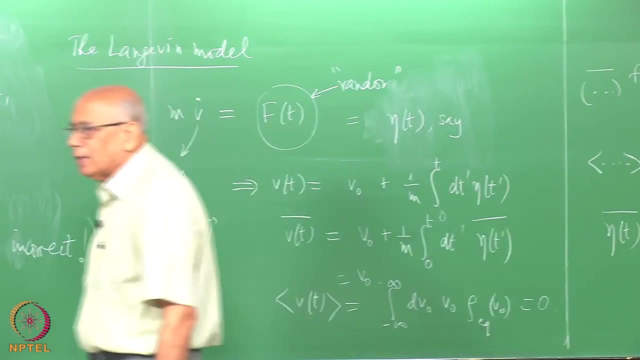 Certainly what happens is when you move in a crowd, there are more particles hitting you per unit time from the front than from the back right, And they impede your motion. You turn around and walk in the other direction. there are more particles hitting you from. 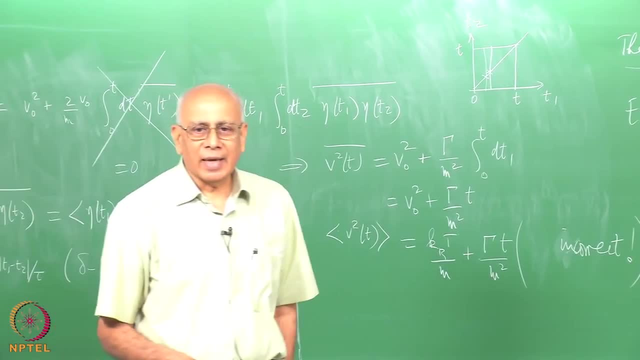 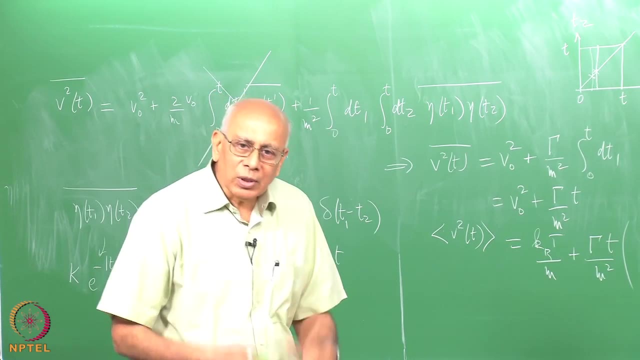 this side and they impede your motion. That is what you call viscous drag. That is precisely it. So there is a part of this random force which is actually dependent on the motion of the particle itself. That force disappears if the particle had zero velocity- instantaneously. 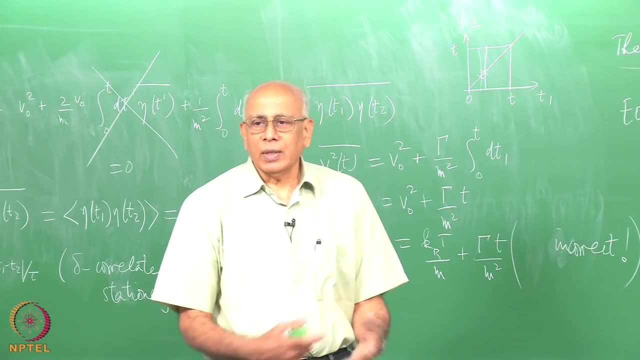 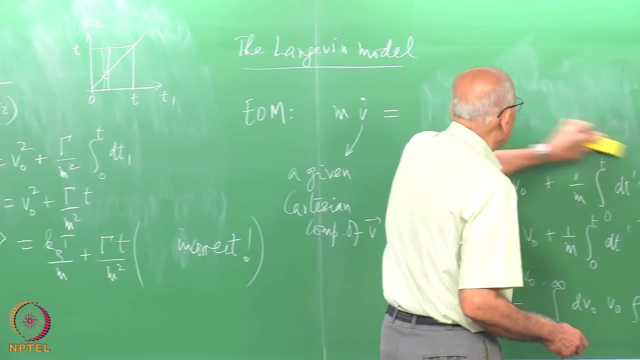 But the moment it starts having a velocity, there is a drag on it, a viscous drag right. So it means that this model is incremental, It is not just a drag, It is incomplete. This force, this random force, has really got two components. 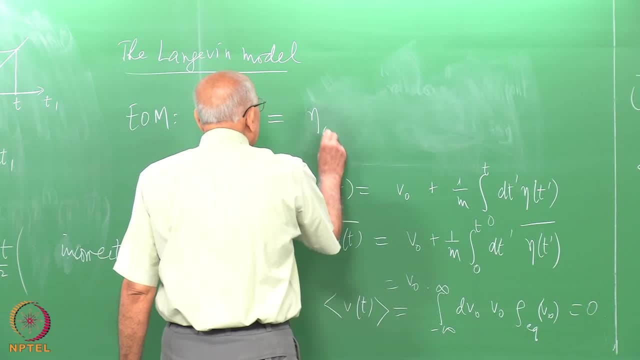 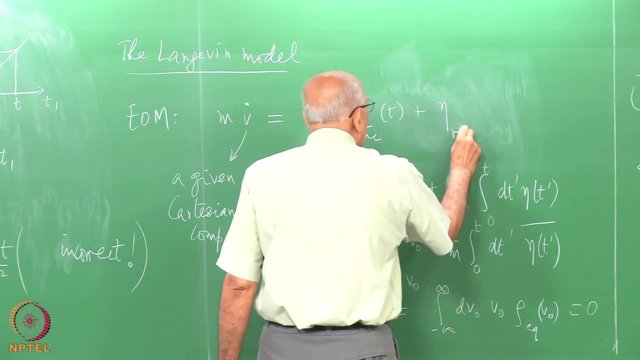 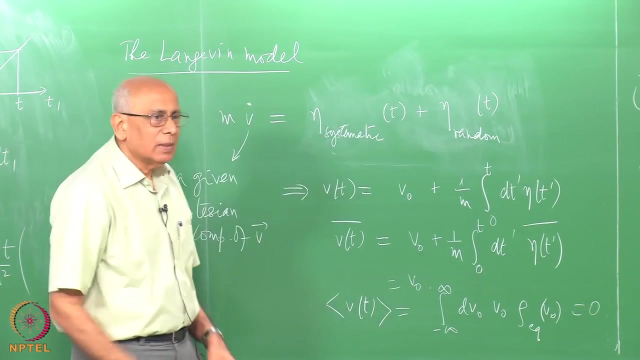 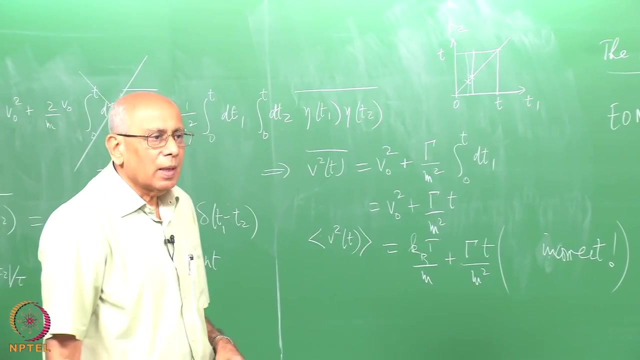 So there is a systematic eta, systematic of p plus eta, truly random, truly random. let's put it in quotation marks: This is acting like noise, but this depends on the state of motion of the particle itself. Ok, And what is the simplest model of viscosity? 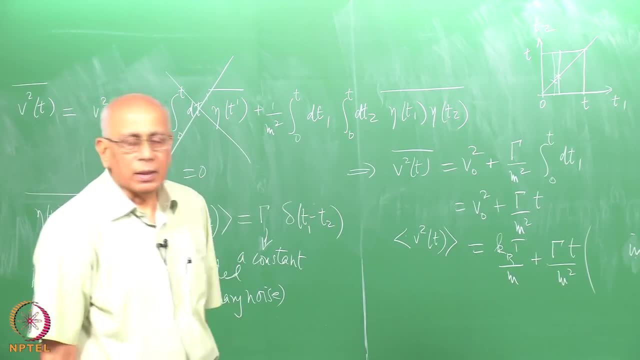 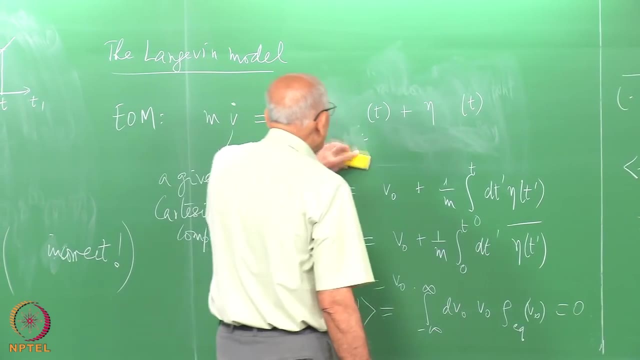 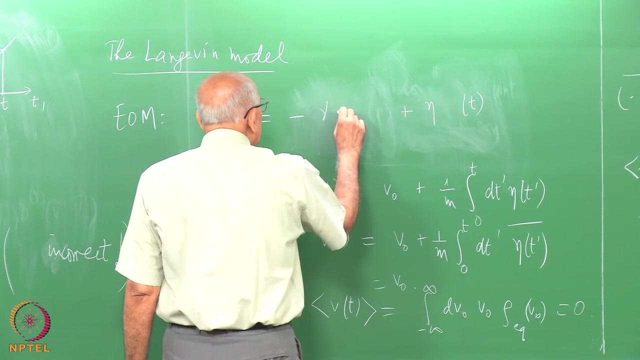 A linear model proportional to its velocity. So it is clear that what we ought to do is to leave this as the white noise out here. But this quantity here is in the direction opposite to the motion of the particle, multiplied by some constant gamma and then v of t itself. right, 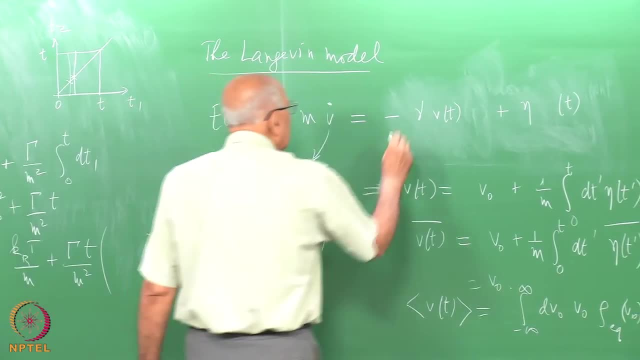 I want this gamma to have dimensions of time inverse, So let's put an m here, Sir. what is the drag force? Sorry, sorry, sorry. What is the drag force, Sir? yeah, yeah, What is the drag force? 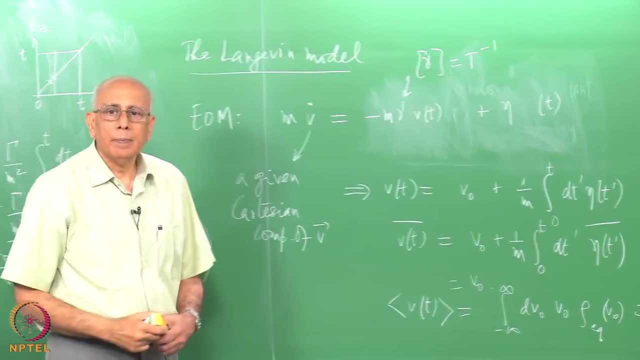 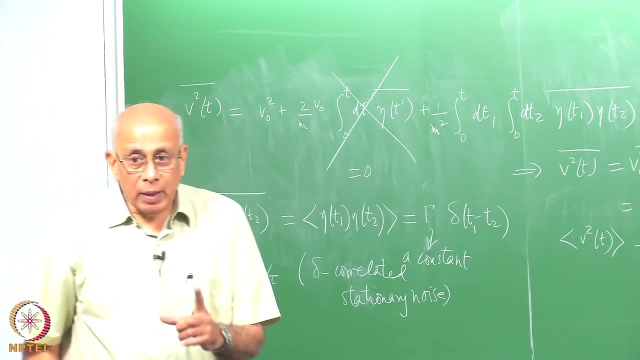 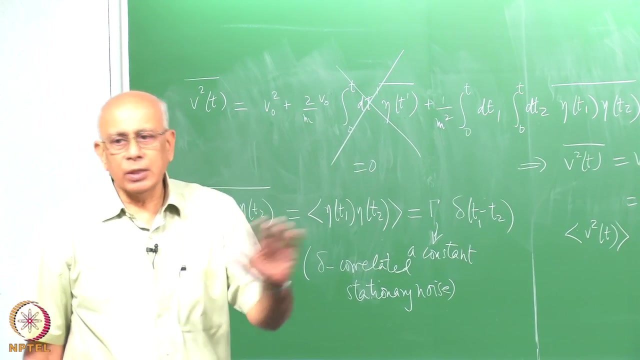 This is a much bigger particle right. What you call viscosity is the internal friction in a fluid which any given fluid layer sees due to the other particles in the fluid right. So we are now adopting an extremely simple, naive view. Yes, I can do that. 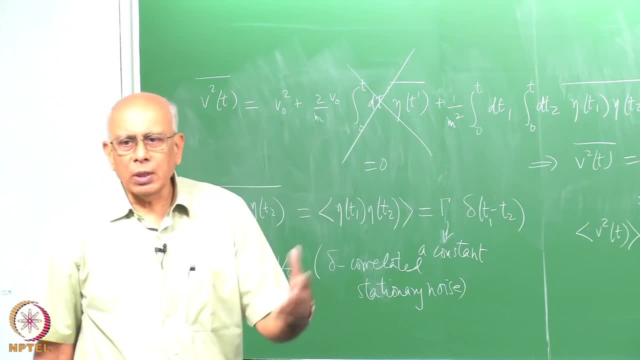 a naive view of viscosity as being simply proportional to the velocity to start with, But we will see if this can be refined. It should be refined, But that's the zeroth order, guess. Eventually, I have this vague feeling somewhere that this quantity, this 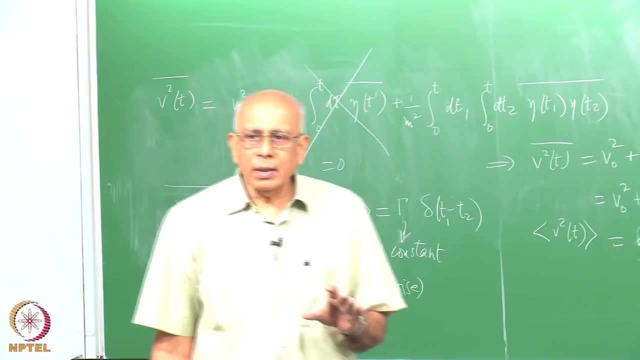 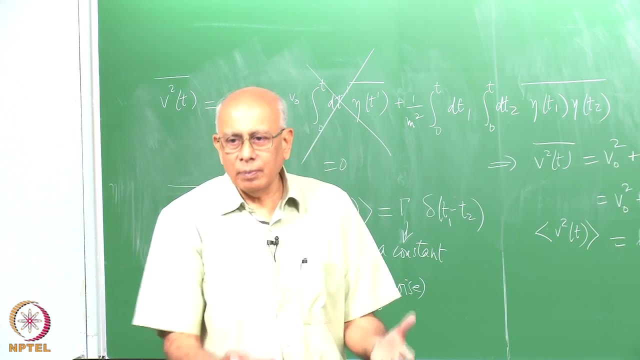 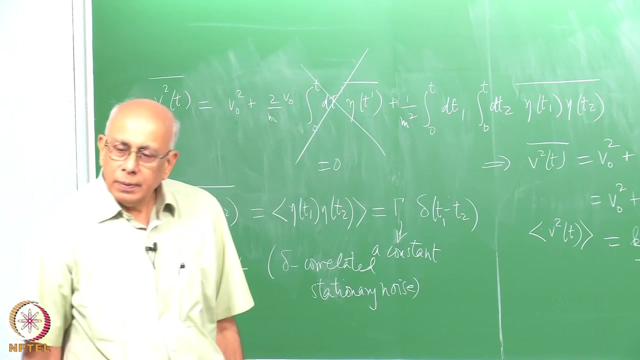 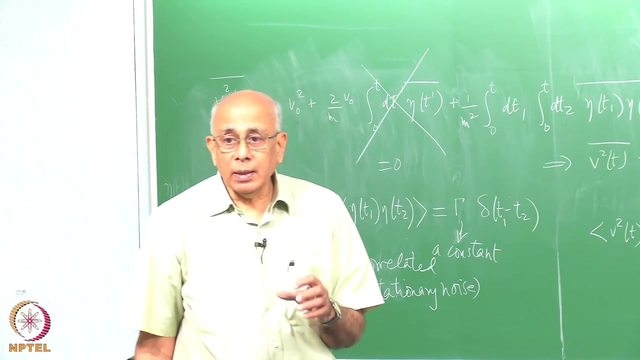 force, this gamma, this constant gamma, will get related in some mysterious fashion to the viscosity of the fluid. That's what I would expect, because that's what measures the level of viscous drag. drag forces on objects in the fluid right. But this object is much bigger than a given molecule. 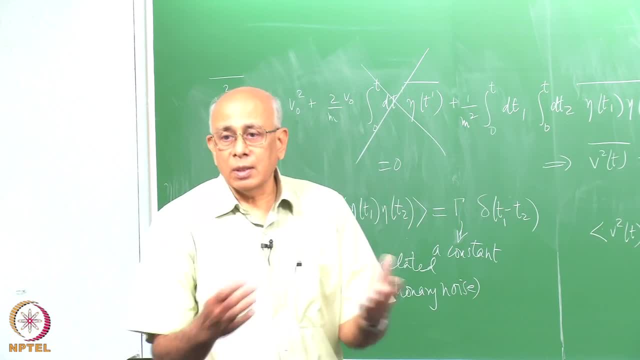 No, it's much bigger than a molecule. It's like when you calculate Reynolds number to tell you when turbulence sets in, etc. The viscosity plays a role because you put a big circular obstacle or spherical obstacle or whatever inside a fluid and then you measure what the drag on it is. 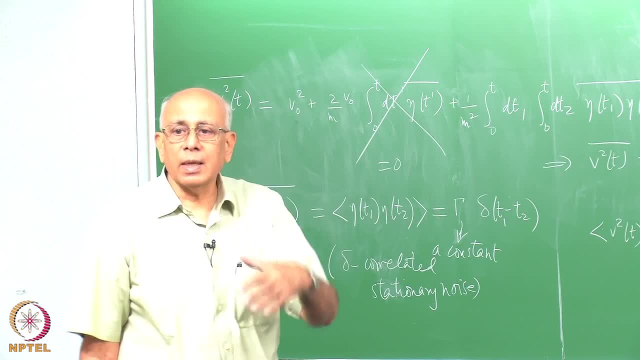 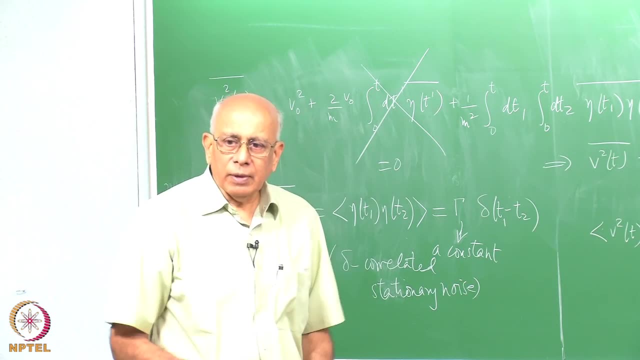 So that's one of the reasons I said: this particle we are talking about is tens of thousands of times bigger than the molecules, So it's not at the molecular level. But the manifestation of that will come from a property of the fluid, which is its viscosity. And yes, it's a hard. 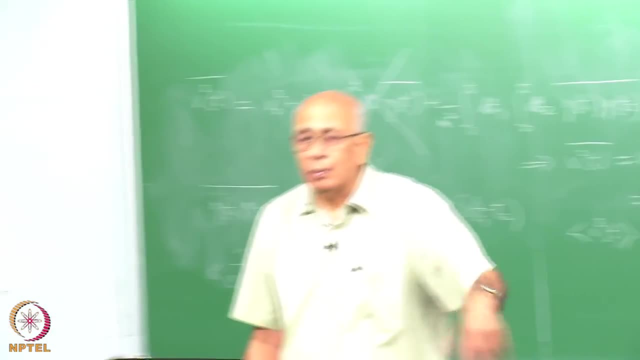 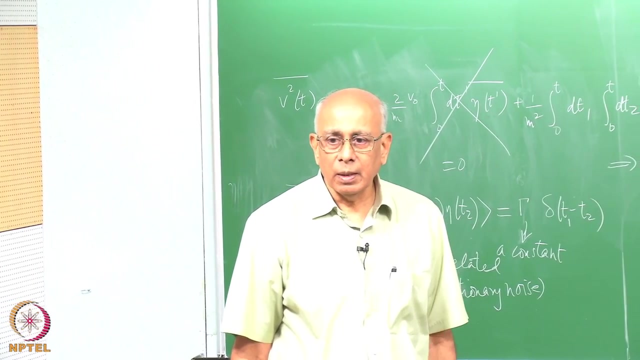 problem to calculate what the coefficient of viscosity is from the molecular level. But that's a standard problem in many body theory. There are computations for it. I might even mention some of them later. So this is the model we are going to put in. 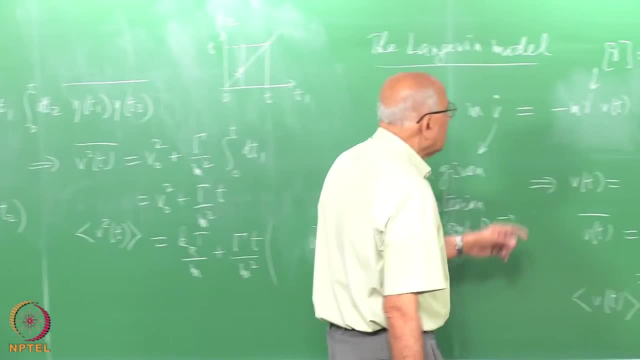 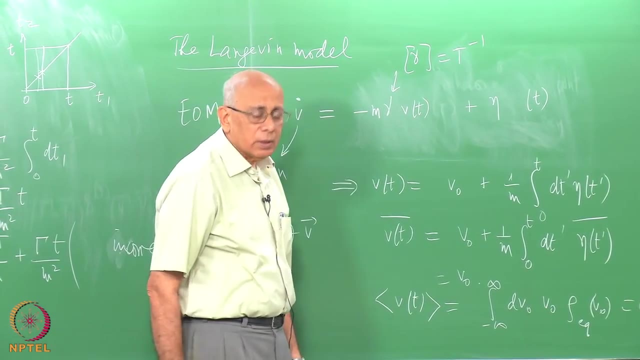 I will stop here today, since we have run out of time. But once you put this in and make the same assumptions about eta of t, we go through exactly the same calculations. Let me just write down just the first step in it. The solution, of course, is v, not e to. 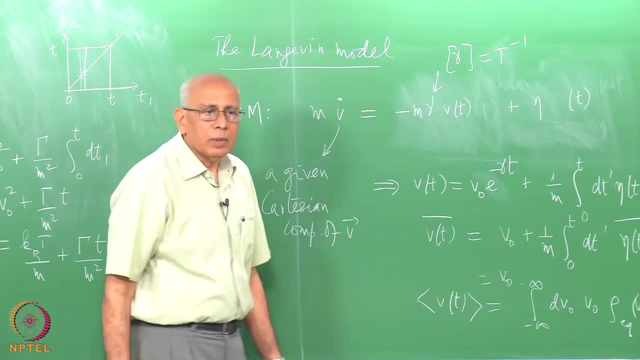 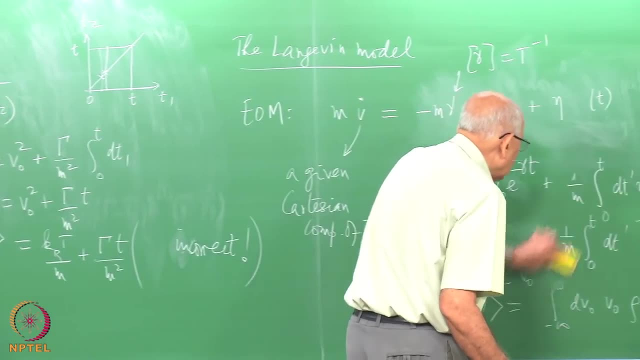 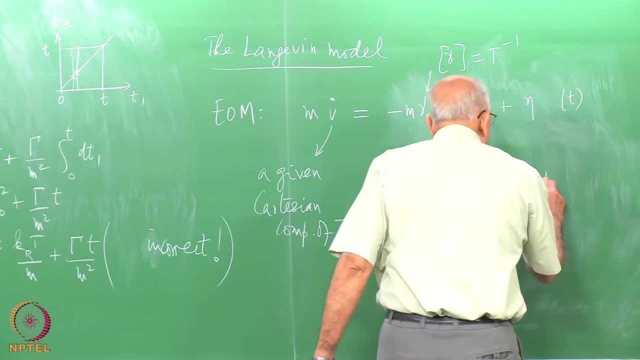 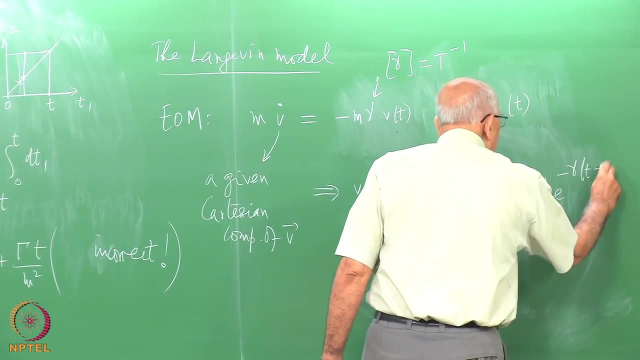 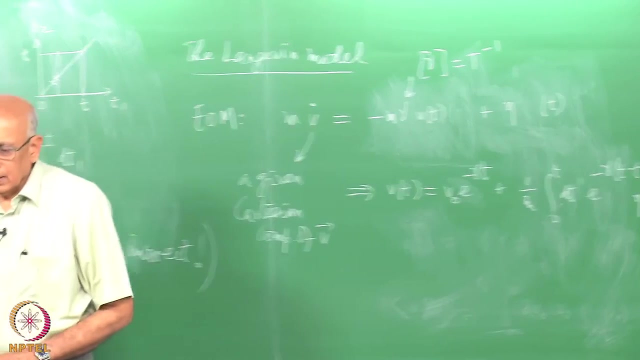 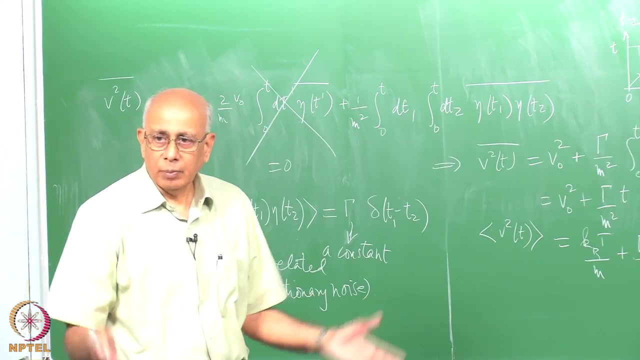 t. So you have plus 1 over m, integral 0 to t d t prime, e to the minus gamma t, minus t prime into k. So that's the solution, And I request you to find out now what the mean value is, first the conditional mean, and after that the complete mean, and then similarly.